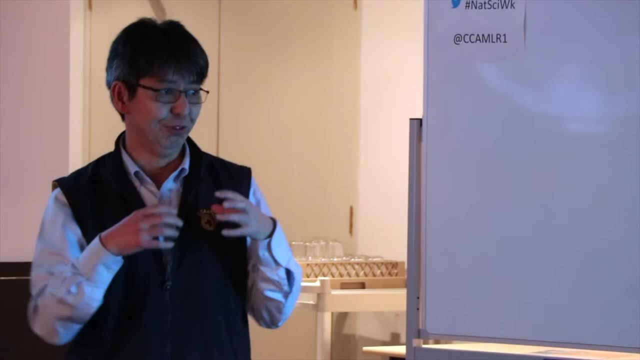 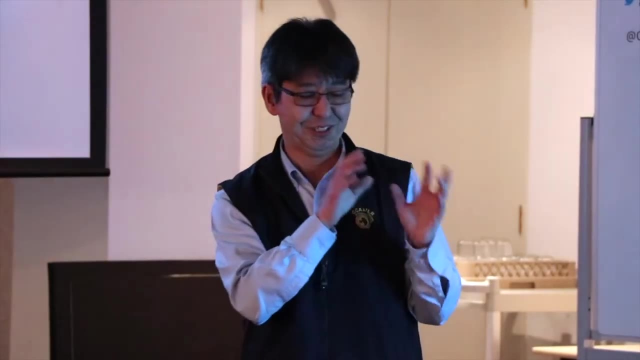 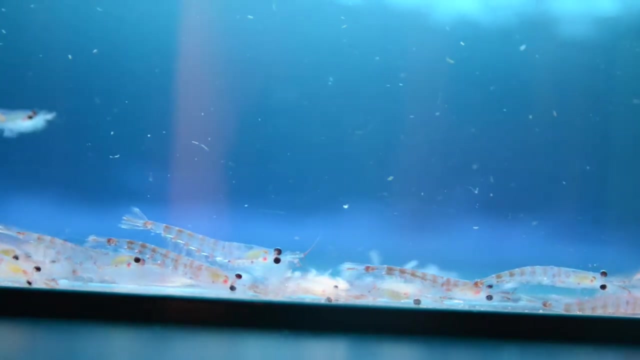 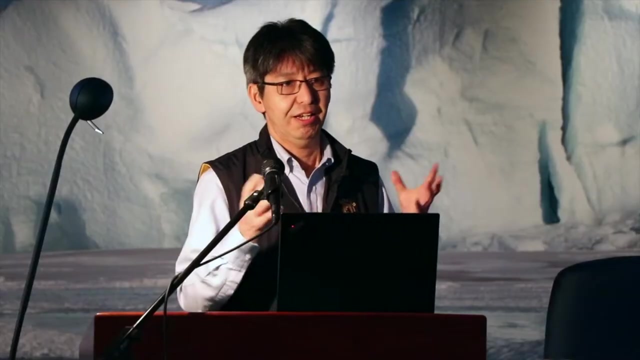 of those primary producers and then package it into their body and then passing the, the energy, to the, the higher predators. they are actually the key to the Antarctic ecosystem. They can grow rapidly during the summertime when they have lots of food, but also when they have less food they cannot grow much, or 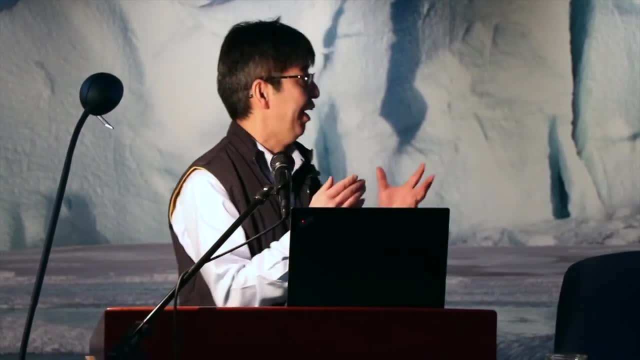 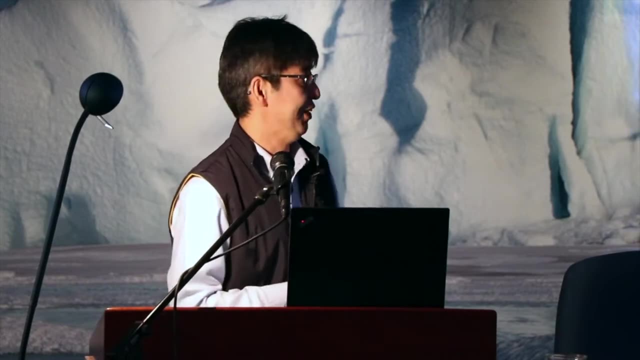 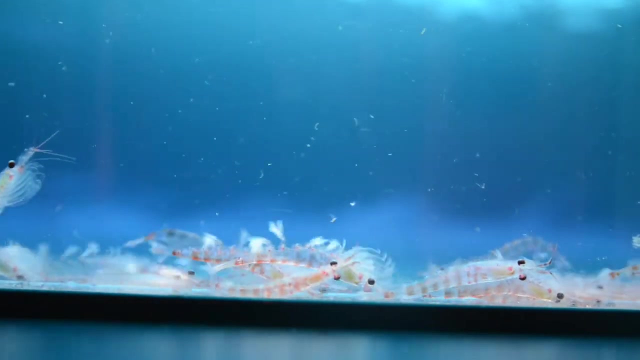 even shrink. So it's really hard to, you know, get the handle on their growth rates and so on, which is very important for our fisheries management and so on. You can see that mold. they are crustaceans, so they have to shed off the exoskeleton to grow their size, They shed. 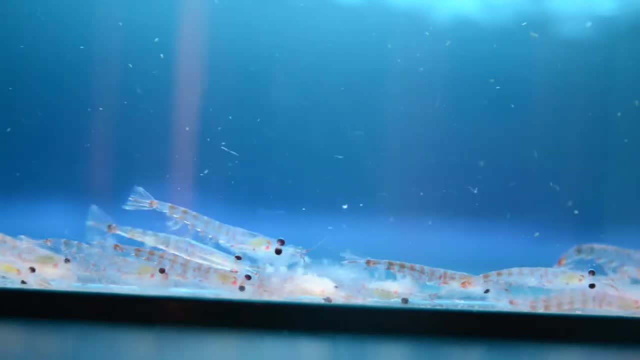 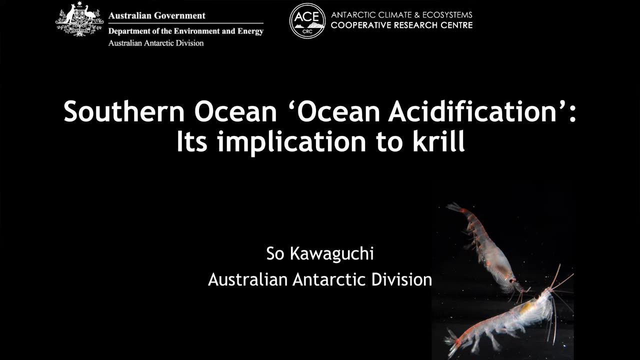 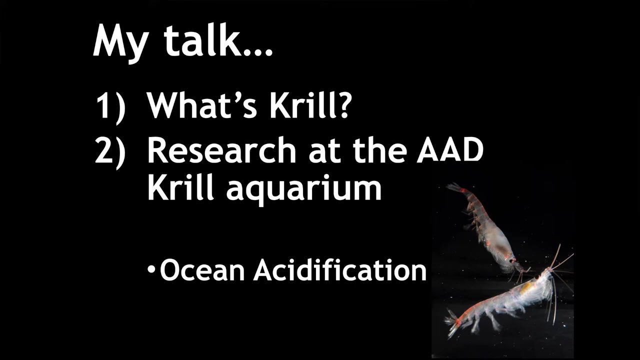 their exoskeleton once every two or three weeks, so they do that for the entire life. The first bit of my talk is a bit more about krill- introducing about krill- and then second half of my talk will be about my research at the AAD. 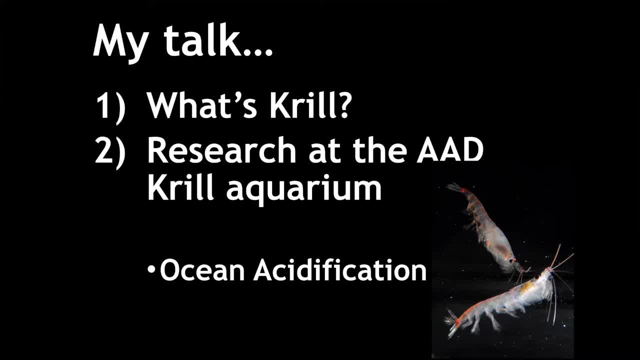 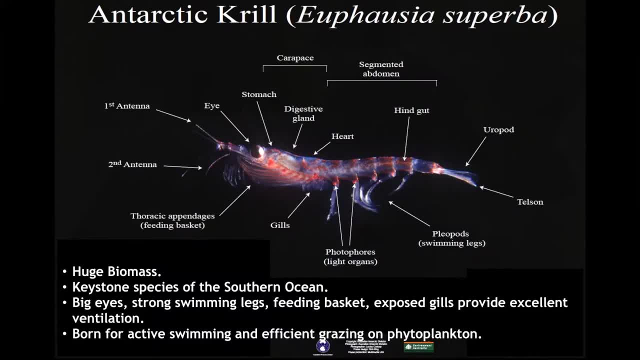 Aquarium. It's specifically about the effect of ocean acidification on Antarctic krill. This is a blow-up of krill and, as I said, you know they have huge biomass, of course, and keystone species of the Antarctic food chain. but basically, you can see these big eyes. these are the swimming legs. we call them. 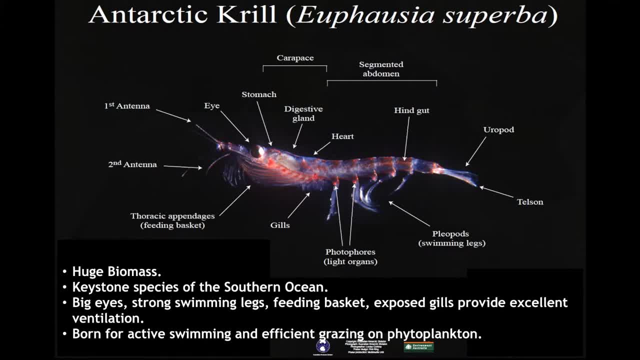 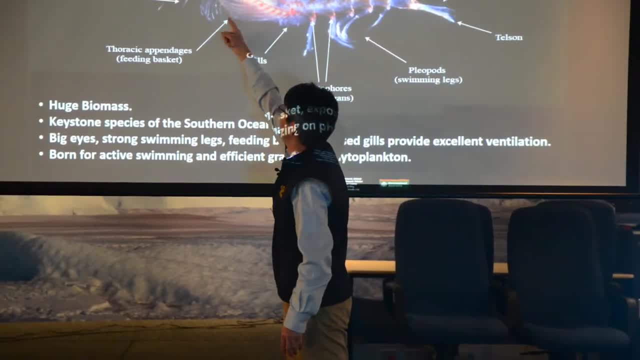 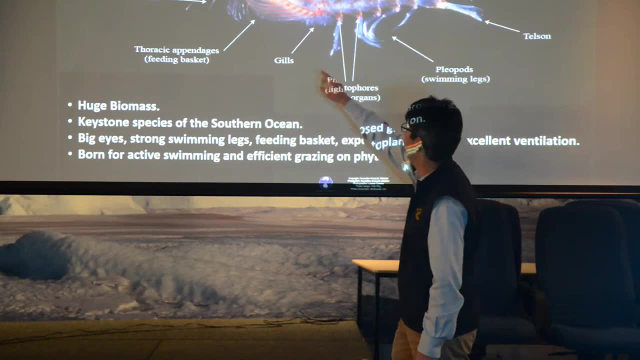 theopods that they are beating very, very strongly. and also you can here see the feeding baskets. So by moving these front legs they can sieve off the phytoplankton very efficiently. Also you can see the gills here which is sticking out from. 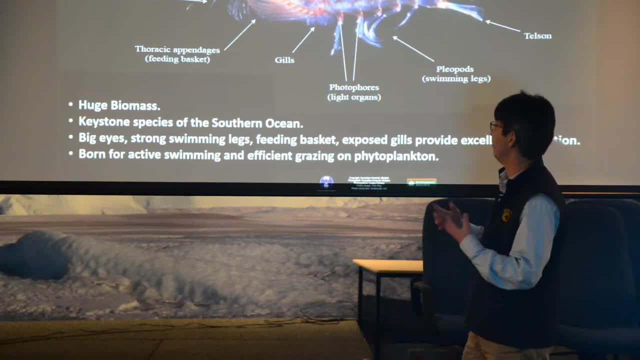 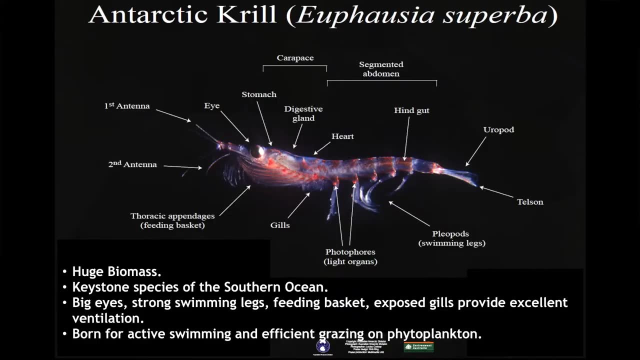 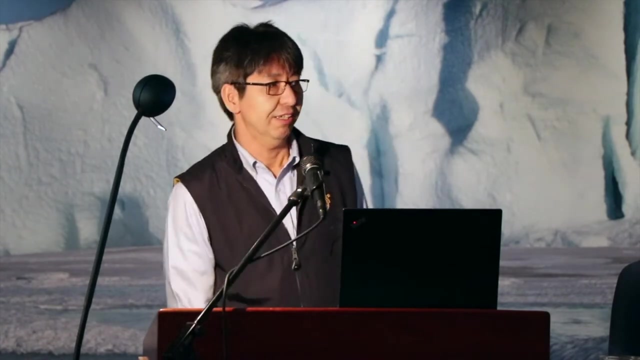 their body and that's really good ventilation. So born to be a very active, breathe very well, A lot of food and then swing fast. so that's the kind of feature of krill. They are young and they are more associated with the ice, sea ice and especially. 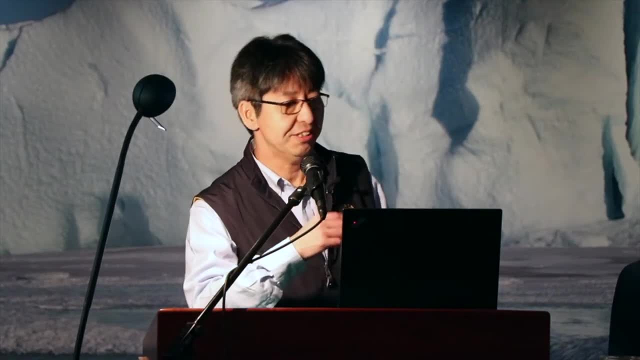 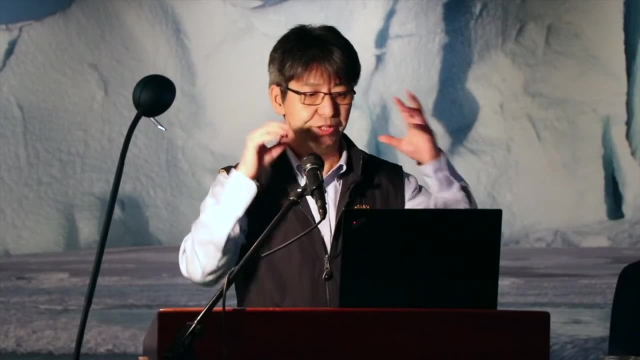 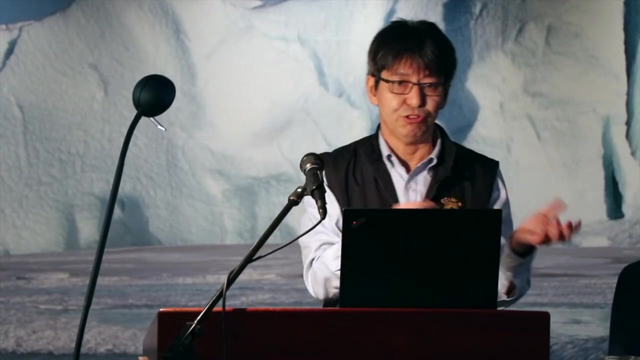 underneath the ice, where there is canyons and also the terraces They are. they love their places and then they huddle together and then hide within those features And also because they are associated with the ice, they won't be driven away, driven away by the current. 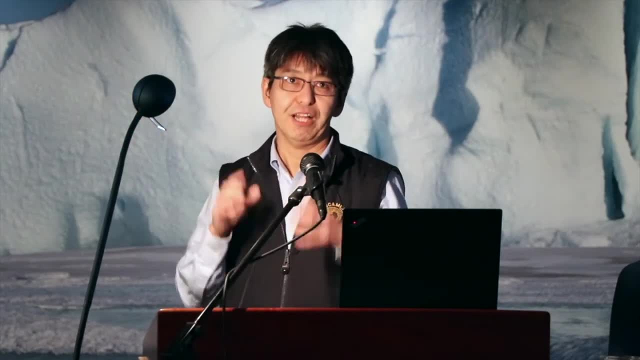 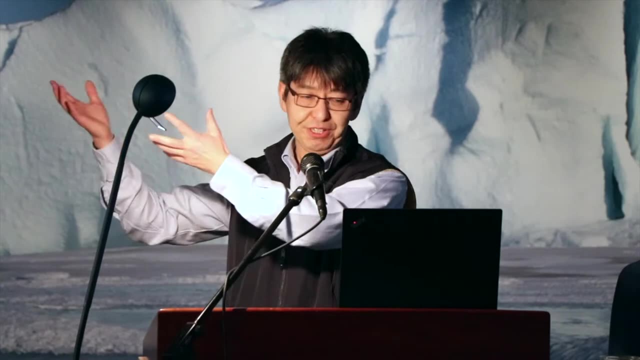 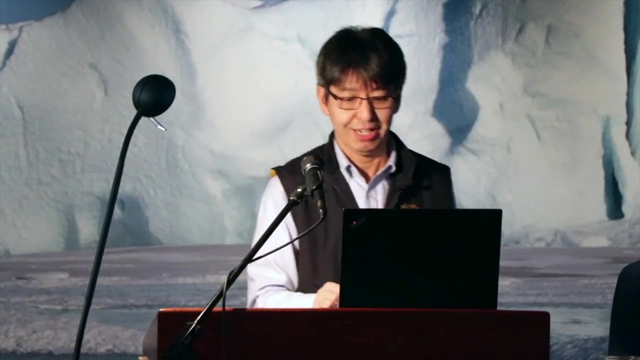 because when they are young they still don't have enough, you know, swimming capacity to swim against the current. So by being within those features they can stay together and make sure that they aren't, you know, driven away by the current. The other thing, when you look the krill from the sky. 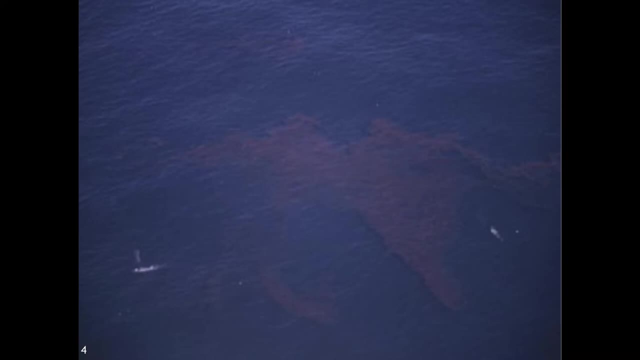 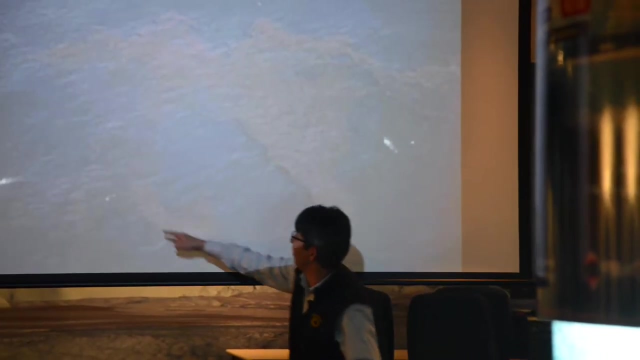 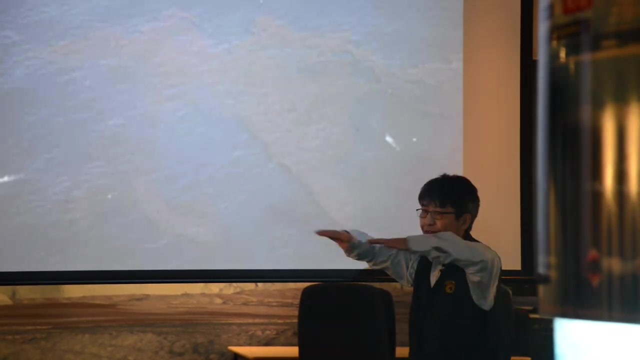 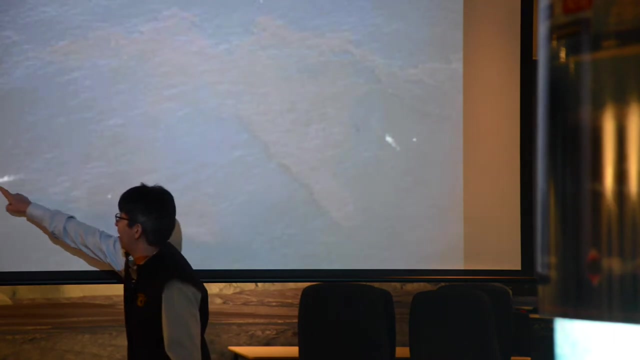 this picture actually shows that the the scale of the crew patch and also have of the krill patch and also how they're existing in those and if you can see this brownish big patch that is a swarm of krills floating at the the surface of the ocean, And what these are. 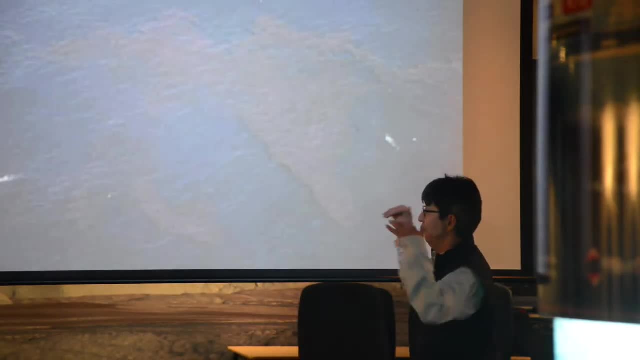 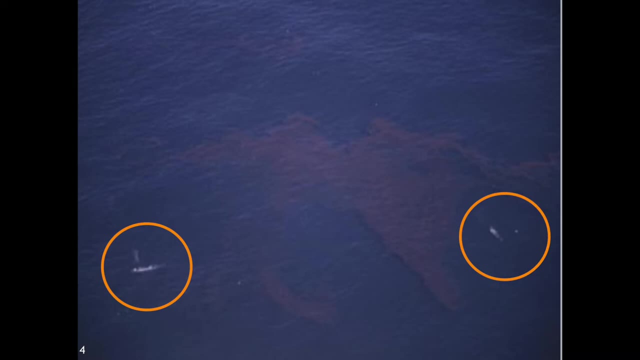 They are whales coming to the- you know the crib patch- to eat them and you can also see them blowing. and you can see a distinct line here where, when the whales approach the krill, they actually try to move away not to be eaten. so there are some kind of very dynamic interactions between krill. 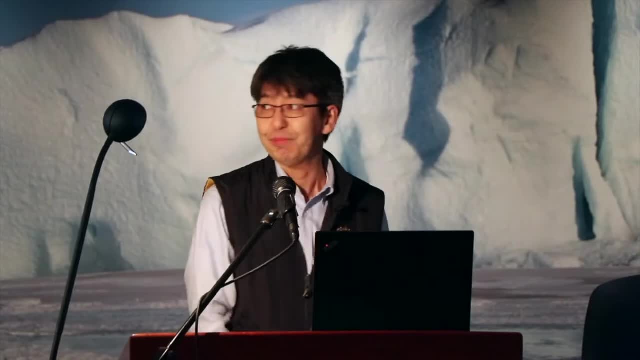 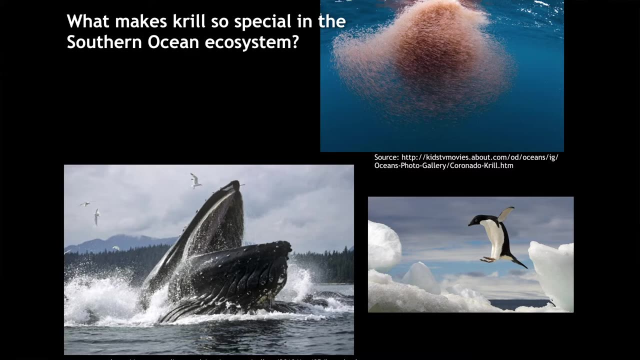 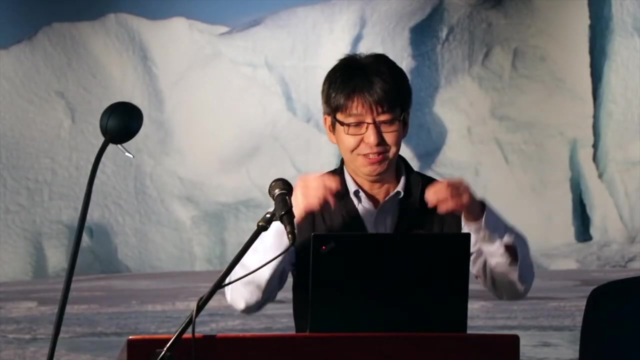 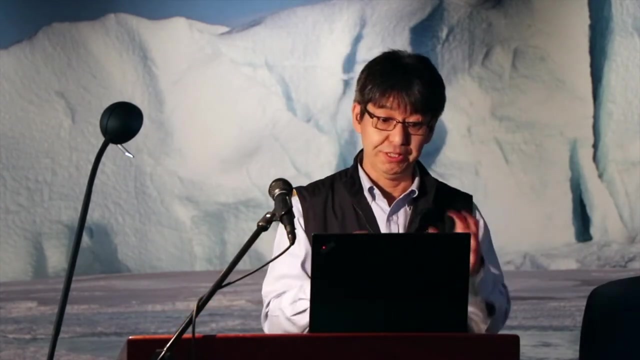 and whales. well, what makes krill so special? and I think, from my point of view, it's their behavior. because of this, you know social behavior. they're always you know, almost for the entire life. they are in the in a group, so that means that you know it is. it is very easy access for the larger predators to eat this. krill and that's why they are so special about nature, You know, being the good food for the higher predators. If something happens to krill- you know population or in the dynamics or the way they behave, it might have a very big implication to the value as a food. 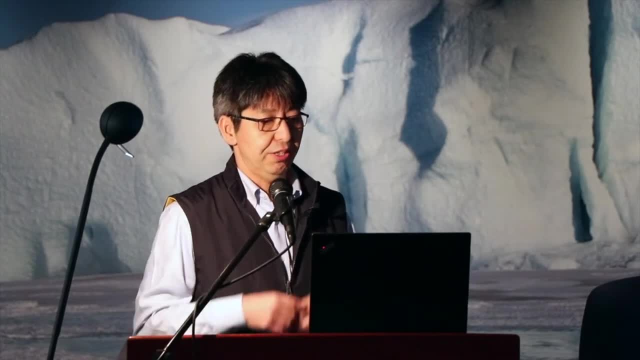 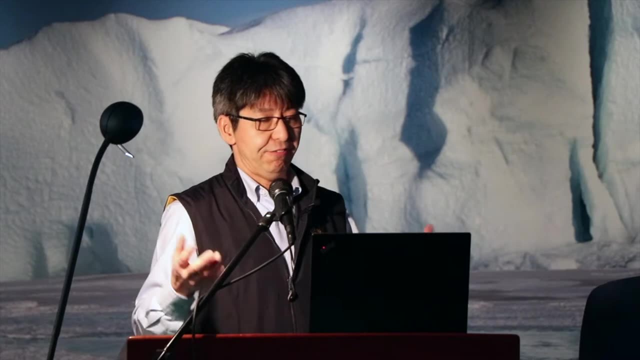 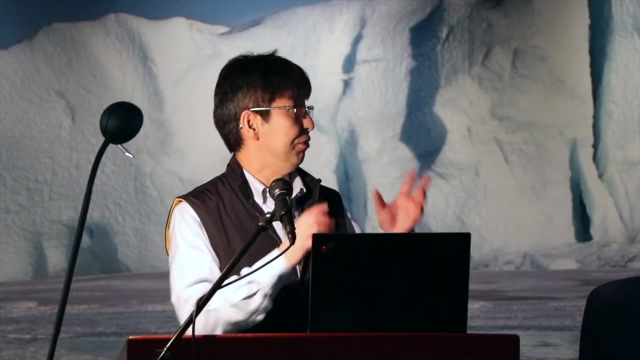 source for the you know the higher predators, and also it might affect the the amount of- you know- phytoplankton they see out of the water. so if anything happens, there might be a change in the food, Change in the structure of the ecosystem and so on. so it's really 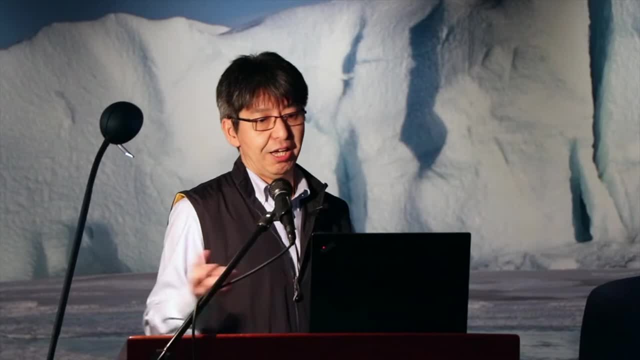 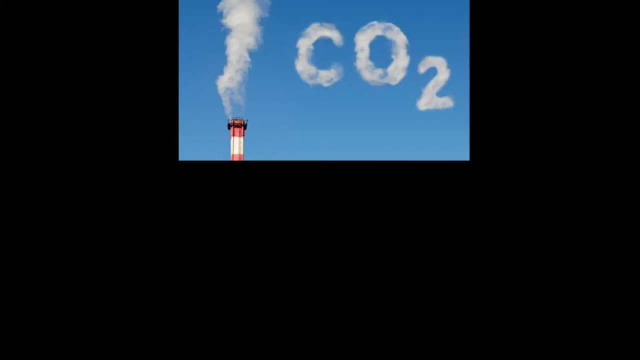 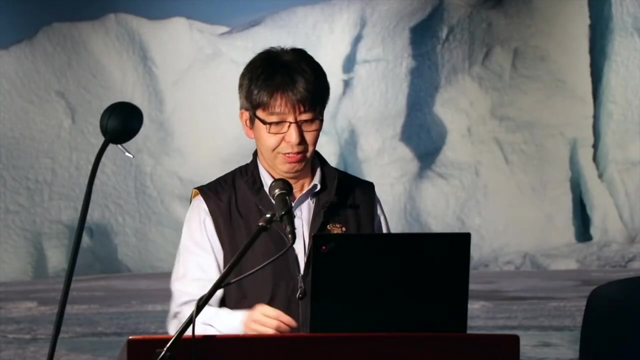 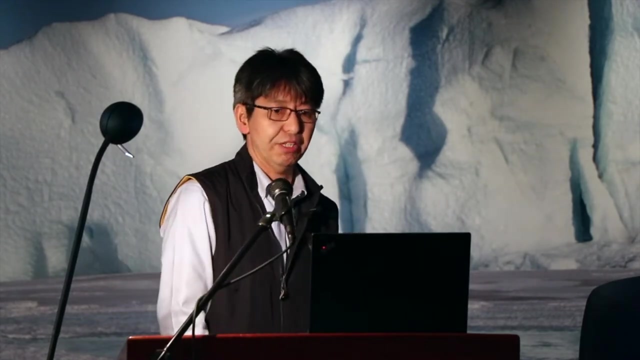 important that we understand how the krill are interacting with the environment and how they might be affected by the climate change and so on. CO2 is a greenhouse gas that is affecting the atmosphere to warm up, but also the other side of the story is that it's not only about the climate, you know. 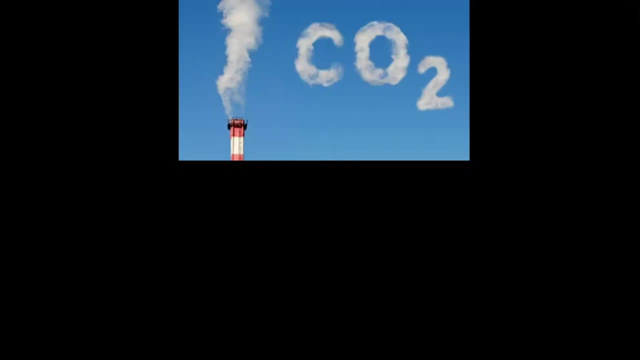 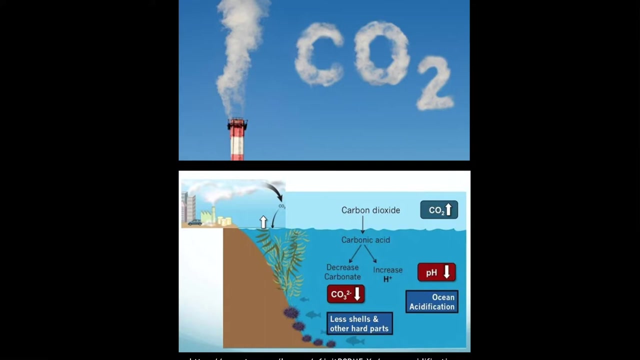 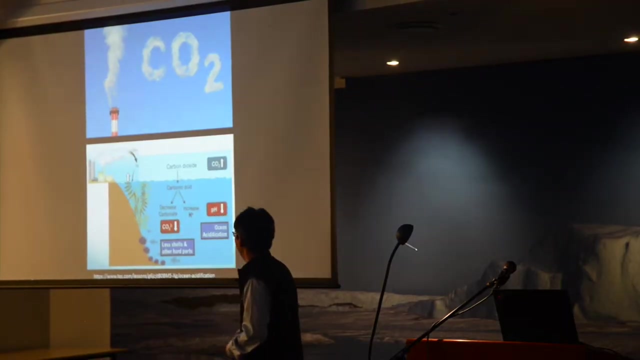 Warming, the, the temperature, the CO2 itself also will be dissolved into the ocean. As the CO2 being dissolved into the ocean, what happens will be that there will be a chemical reaction and, in the end, what happens is that the amount of carbonate which is important for the shelf life of the krill 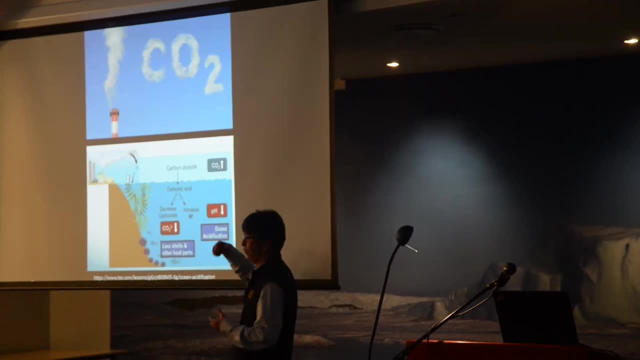 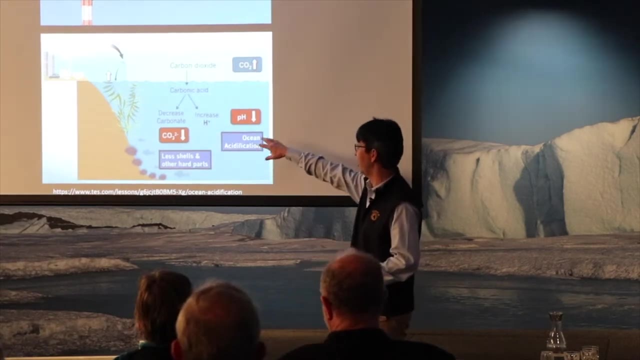 Shellfish to create their shell will decrease, but also the hydrogen ion will increase and then that will bring down the pH. so that is why we call it ocean acidification. As the CO2 increases in the atmosphere, the ocean pH goes down and, interestingly, the amount of CO2 that 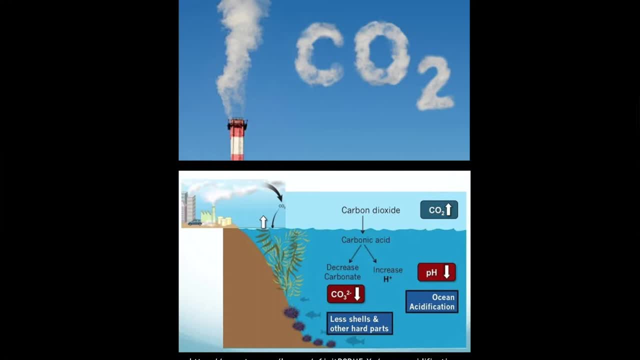 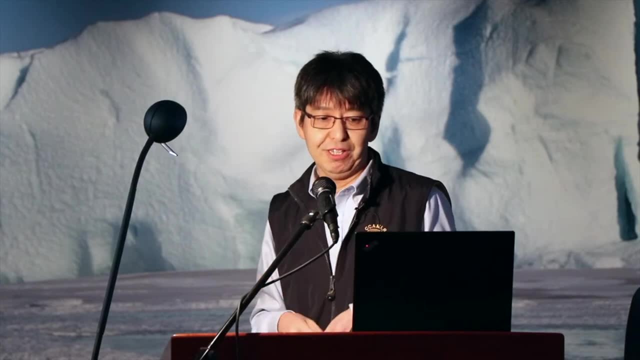 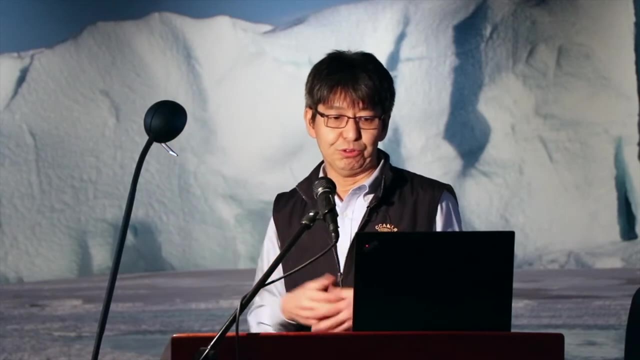 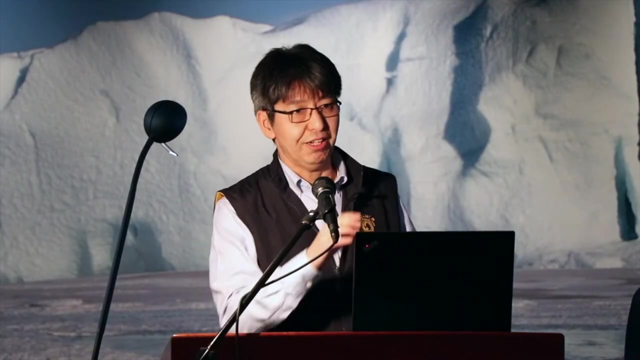 can dissolve in the water or the ocean depends on this, the temperature, so they are more likely to dissolve in the cooler environment. So the ecosystem like Arctic or the Antarctic they are, they thought to be the first ecosystem to be affected by this ocean acidification. We know that Antarctic krill is a very 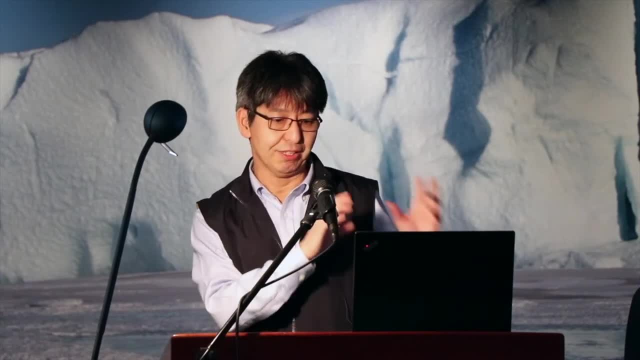 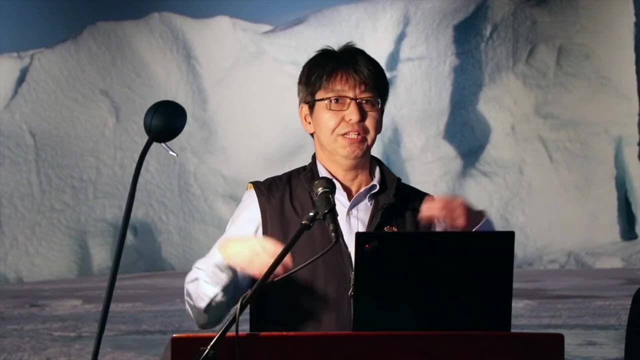 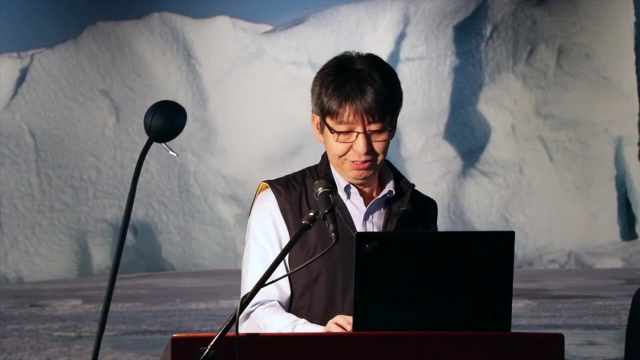 important component of the ecosystem in the Antarctica And we are really worried that what may happen if this, you know, the CO2 increase, the, the pH goes down in the Antarctic Ocean. So to find that out, we really need to do something about it. and that brings the importance of the experimental. 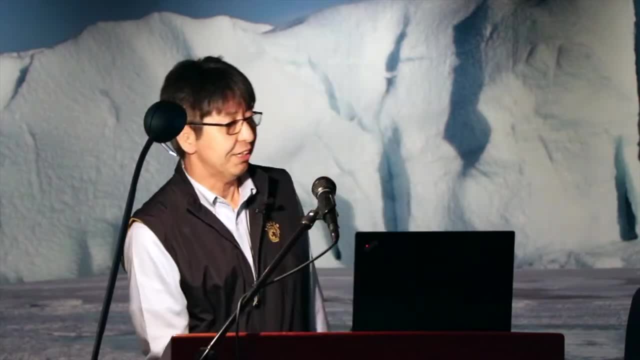 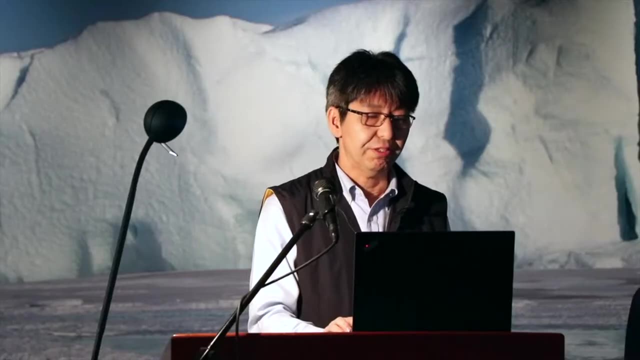 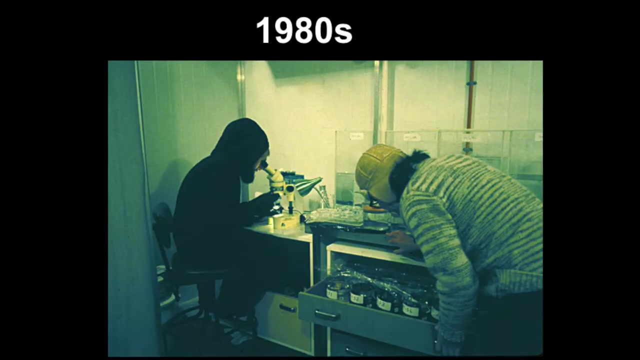 approach to find out the effect. Luckily, we do have a research aquarium dedicated for krill in the Australian Antarctic Division. The research aquarium actually started in the 1980s and when it first started it was just in a freezer lab. and we have to wear these freezer suits and doing a 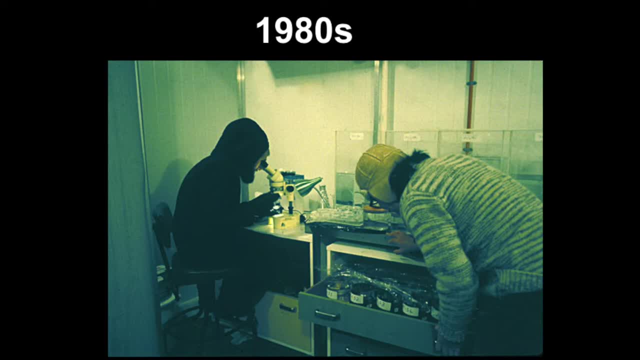 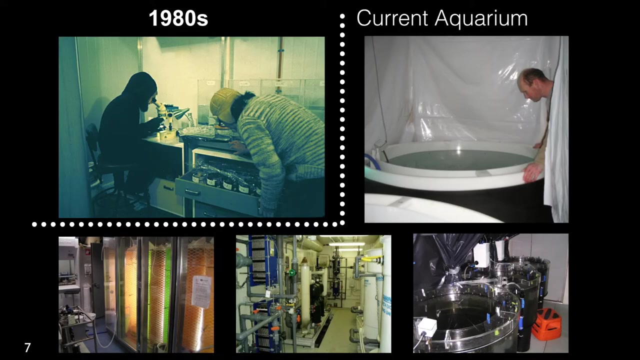 very small scale in a beaker doing the experiments, so it was very cold. you cannot stay in that environment for more than 15 minutes or so. it was very, very harsh. What we have is like this: the lab is in a room room temperature and the water 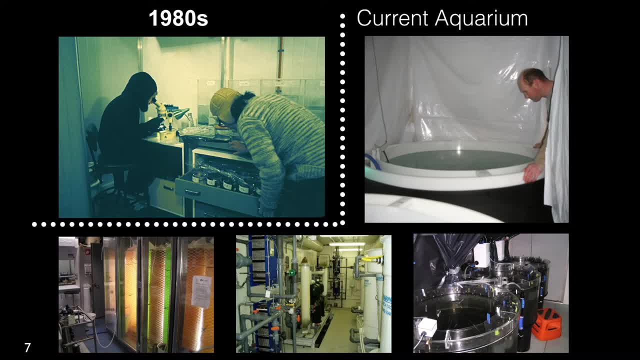 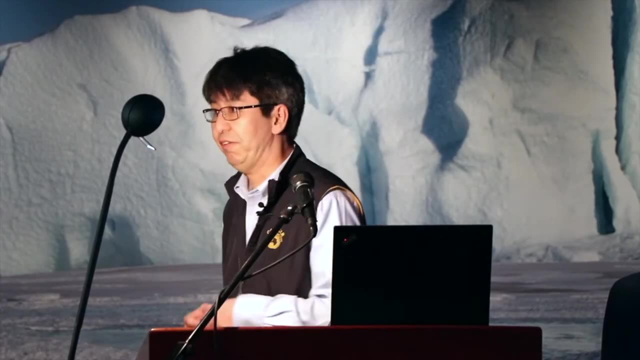 itself is only, only the water itself is cooled down to zero degrees. and we have these sophisticated, you know, instruments to control the things. Because of this development, now we can control the sea, water temperature and CO2 levels and all sorts of things to mimic whatever environment which. 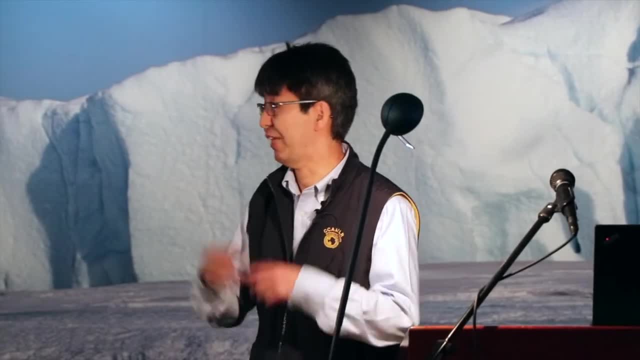 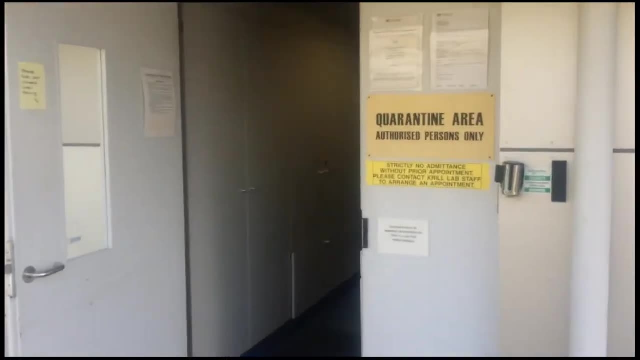 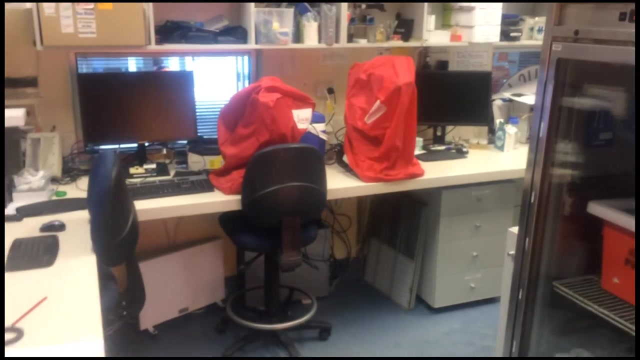 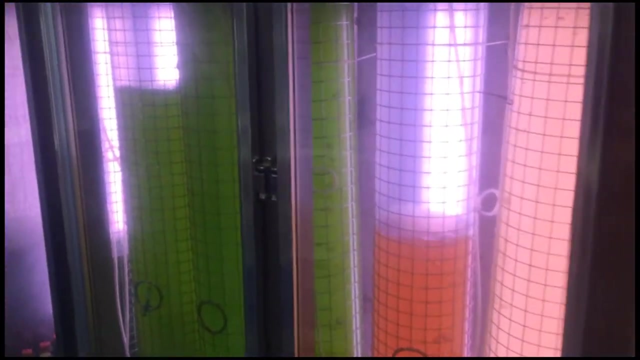 will be expected into the into the future. So that's why we can do many interesting experiments using our aquarium. As we walk in, we can see the main lab and we do have, you know, microscopy to look into the. you know the structure of krill. We culture phytoplankton as food for krill here and 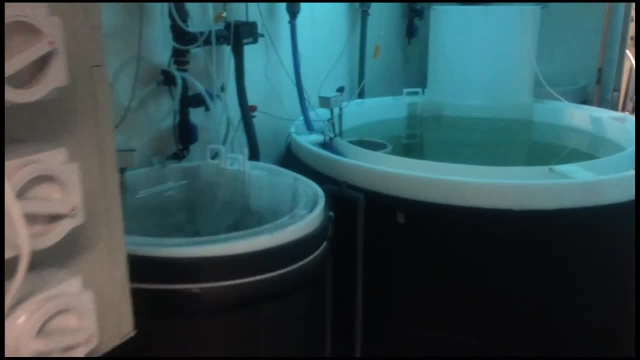 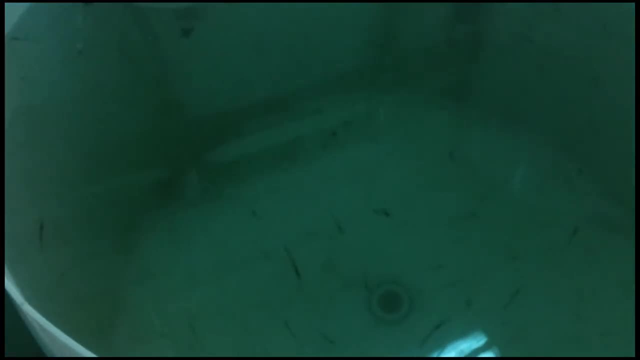 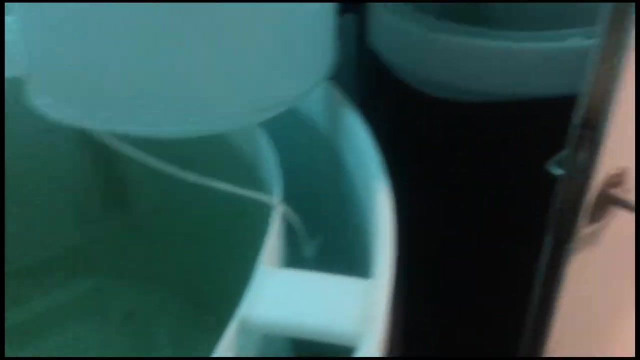 as we walk into the main holding room. this is where we keep our krill. This is a feeding time now, so the water is green, but actually this is a super clean water. the green color is because of the phytoplankton at the food. When you walk out this door, 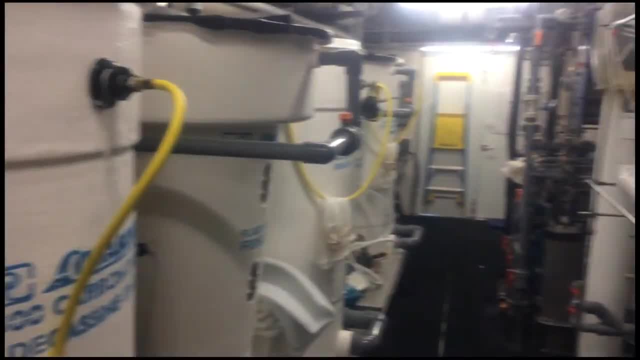 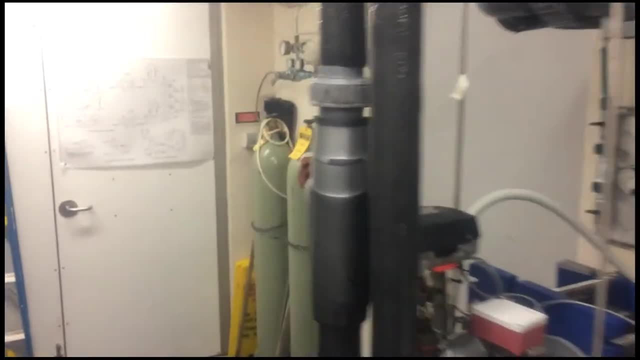 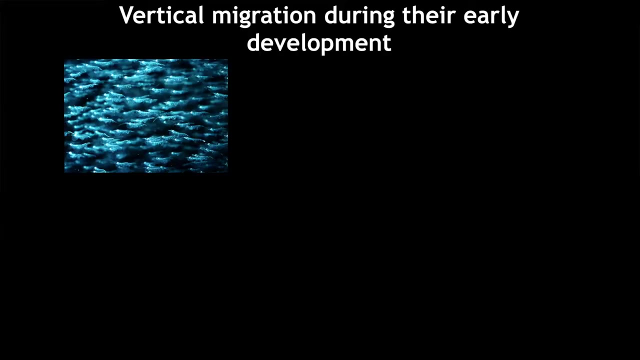 you can see lots of these things which this is a plant to purify the water, filter out the water so that krill can be always kept in clean water, because Antarctic water is very, very clean. Using that kind of aquarium, we started to do some experiments about the impact. 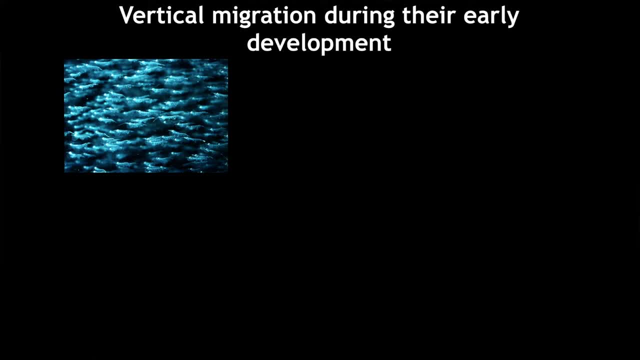 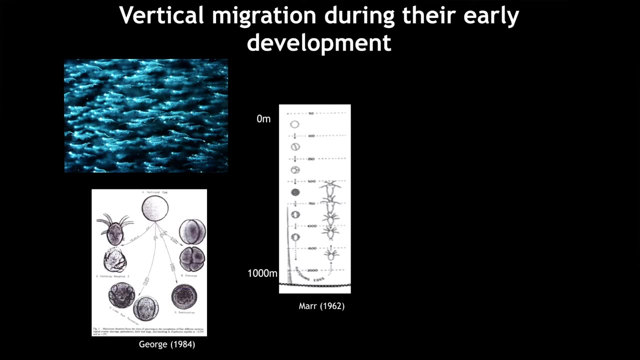 Krill lay eggs at the ocean surface, and then what happens is that, as the krill eggs develop, it takes about 5 or 6 days to hatch out. but what happens is that, because they are heavy, the krill eggs sink down to about 700 to 1000 metres before they hatch. and then they have. 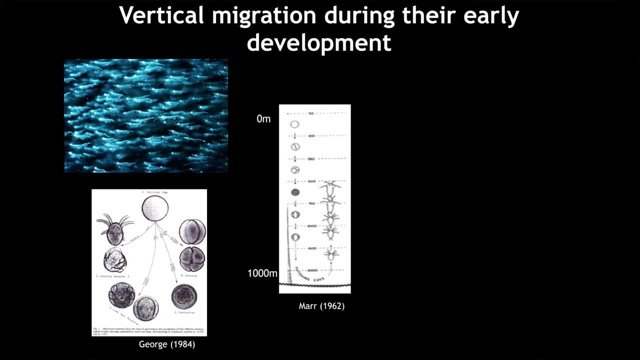 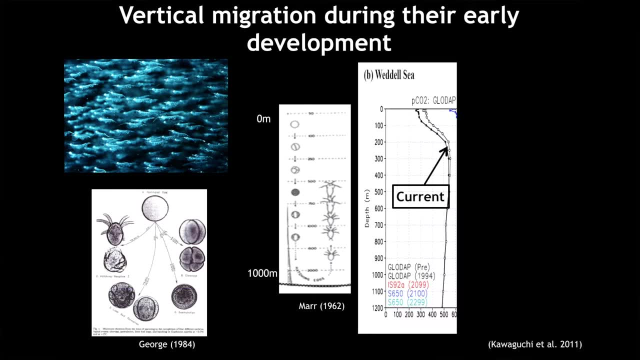 to swim up the water column to start feeding. The other thing that we have to note is that carbon dioxide level in the water it's not the same from the surface down to the bottom. It actually The carbon dioxide level increases with depth. 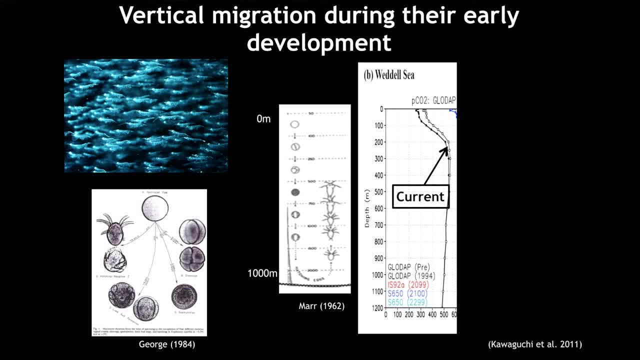 So even if the current situation atmospheric CO2 level is about 350 or 400, something like that, but if you go down the water column it goes up to 500 or 600. The krill eggs as they sink, they are experiencing this already higher CO2 compared to the atmosphere. 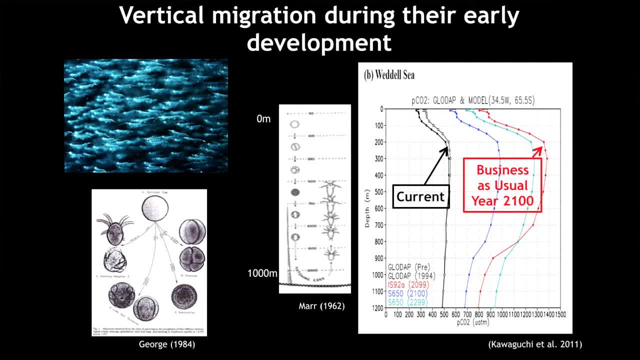 Now what happens in 100 years time? This is a business as usual scenario. so if we keep living in this way and not really do anything about controlling the emissions, probably the CO2 level at 300 metres- 400 metres- will go up to about 1400 ppm. 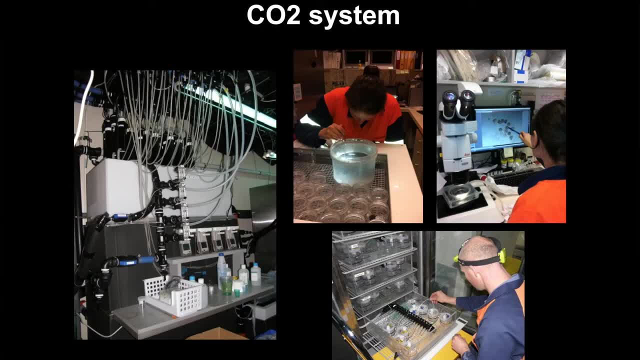 What does it mean to the krill eggs? Can they hatch out? We do have this fancy system that can generate high CO2 water At the same time. we can have a high CO2 water. We can have a high CO2 water. 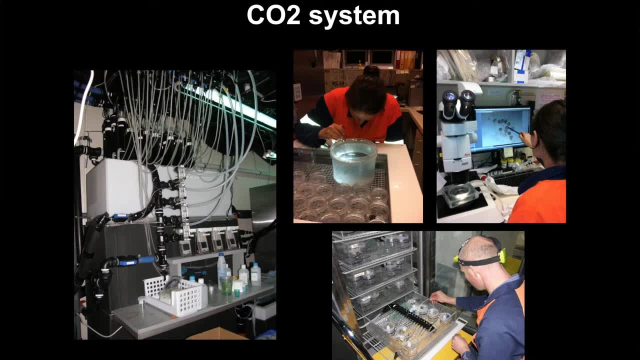 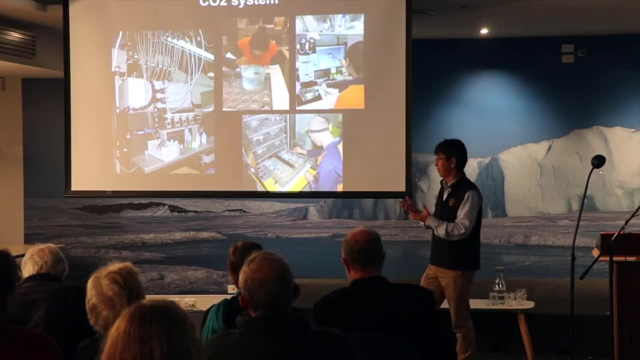 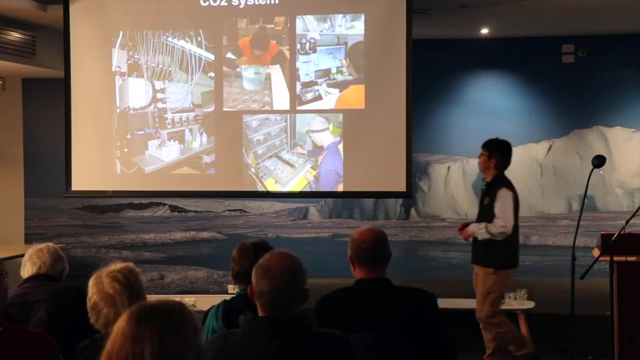 At the same time six different CO2 levels. So what we did was let the krill lay eggs and distribute those eggs into the jars, And then those jars will be put into a refrigerator with the right amount of CO2 level. Let them stay for five, six, seven days and see whether they hatch out. 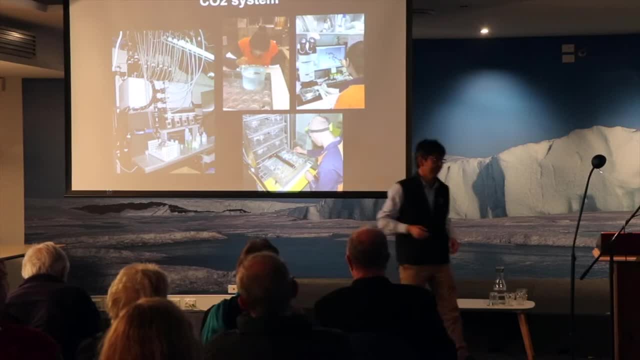 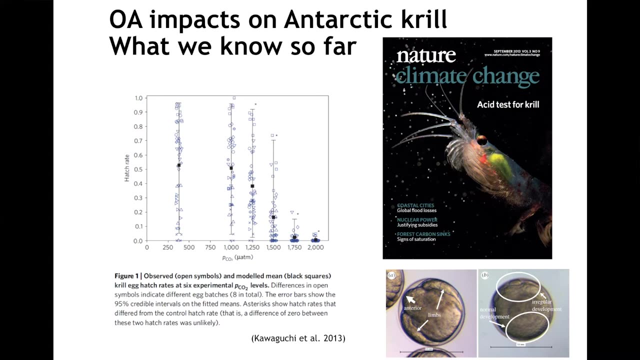 And then, after you know one week or so, we will count the number of the eggs that hatch out, And what we found out was that the hatch rate is quite good, up to about 1000 ppm. But as the CO2 level goes beyond that, the hatch rate rapidly goes down, and the early 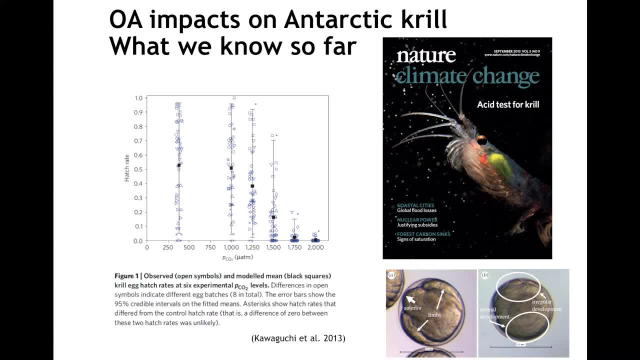 development is stopped. There's some deforming, abnormal development under the high CO2.. This 1000 ppm is not that high If we think of the vertical distribution. If we think of the vertical distribution of CO2, as I indicated in the last slide. 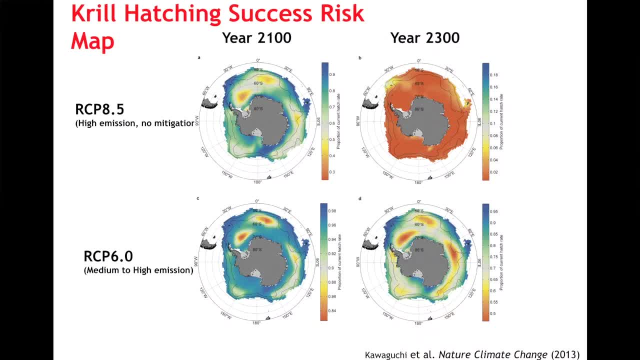 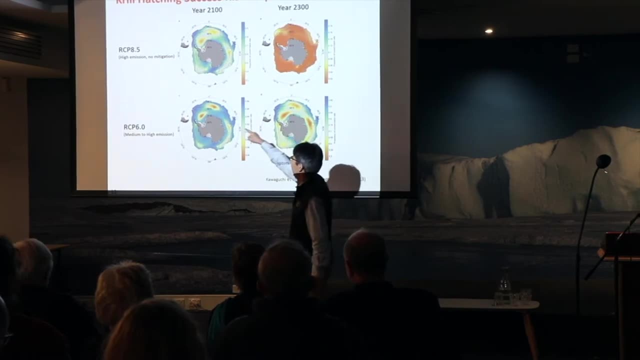 By using those informations we can actually come up with a risk map of the future hatching success in the Southern Ocean. And this is some example. after 100 years, after 300 years, RCP 8.5 is the scenario. that is a kind of a business as usual. 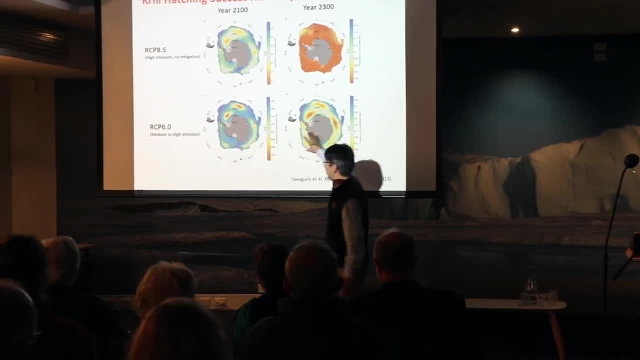 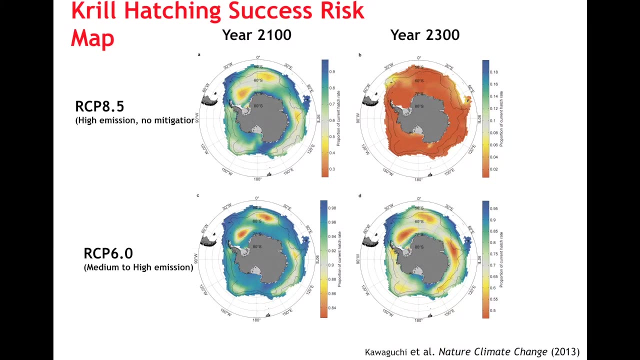 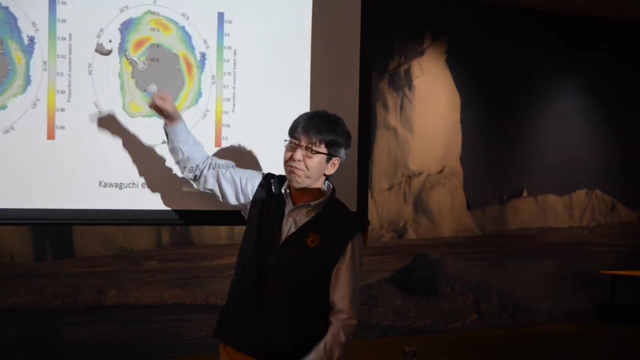 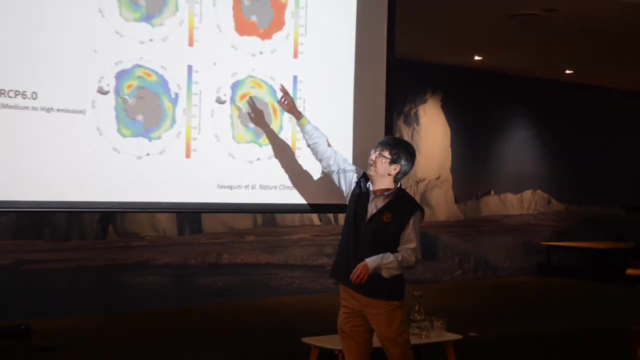 This is another scenario which is medium to high emission. The point is that after 100 years we will see the areas that crew might suffer. in reproducing The orange is about less than half of the current hatch rate can be achieved, So some of the areas might be a bit bad. 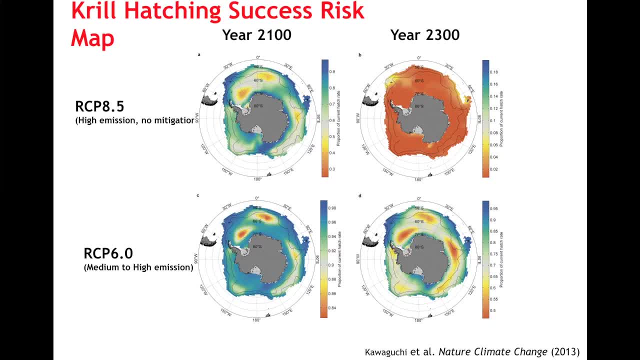 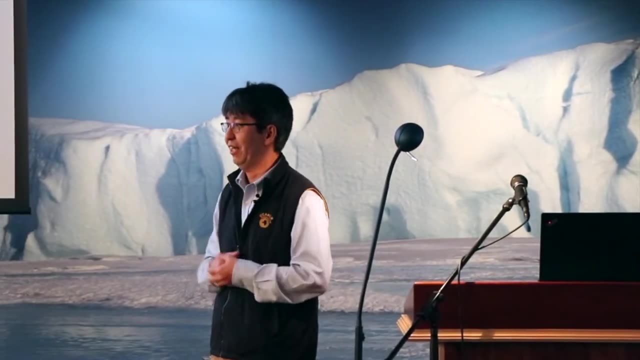 In 300 years time, Almost 100 years, Yeah. So the whole area within the Antarctic waters could be not really suitable for reproduction for krill. That's just only one side story, because we just tested the hatch rates under various CO2.. 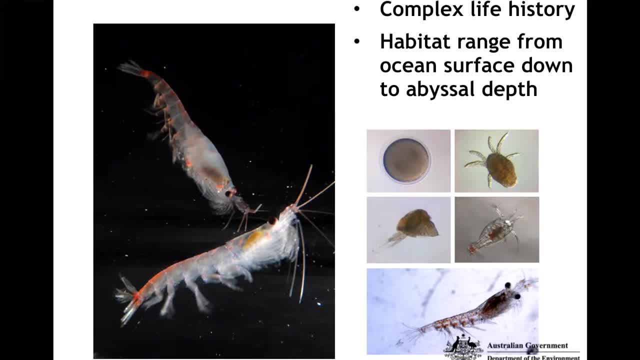 But, as I said, they have complex life history. from the eggs until the adults, They will go through 12 different forms of their larval stages. CO2 will be, of course, different from time to time. To get the full picture, I think we need to test the effect of CO2 throughout the whole. 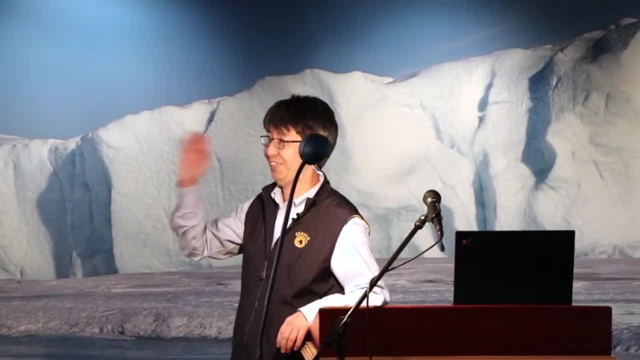 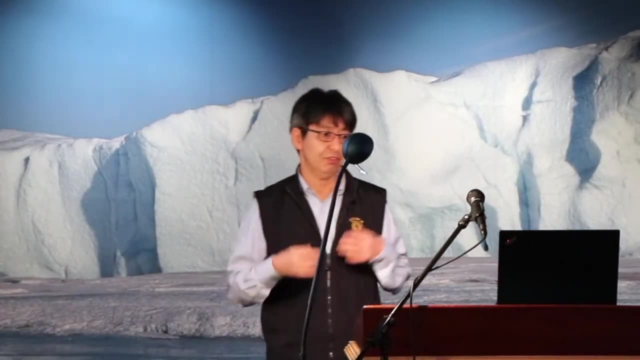 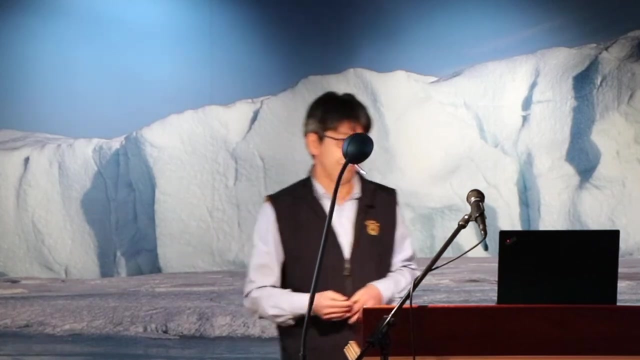 life history. And also, this is only the CO2, but also there's an increase in temperature and so on. What about sea ice? So there are lots of things to do to untangle what may happen in the future environment. Krill, as I said, they are the centrepiece of the Antarctic ecosystem. 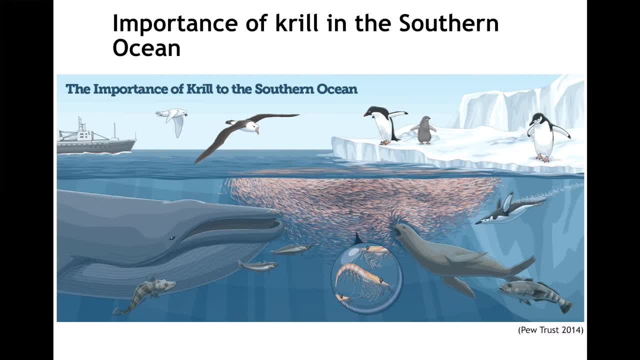 They will be eaten by whales and seals and penguins. And there are sea ice. There might be warming, sea ice reduction and also the increase of the CO2 in the ocean. So we really have to understand through good science and predict what may happen to krill. 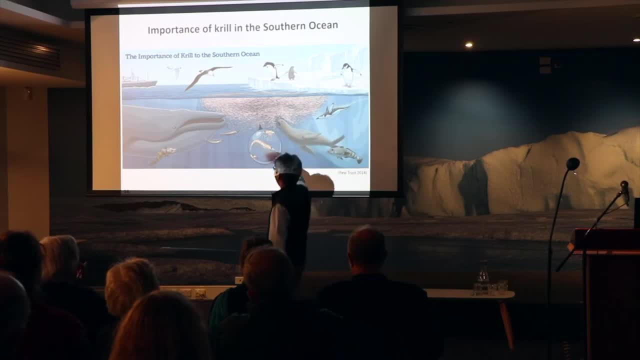 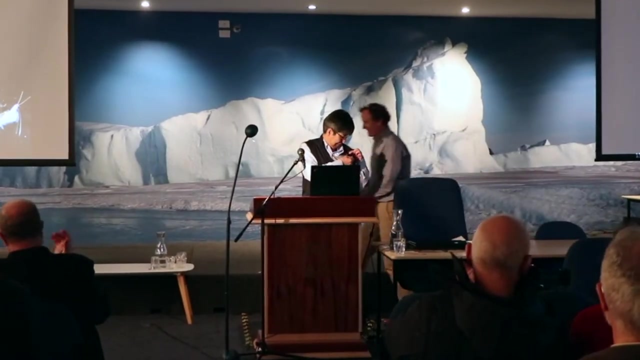 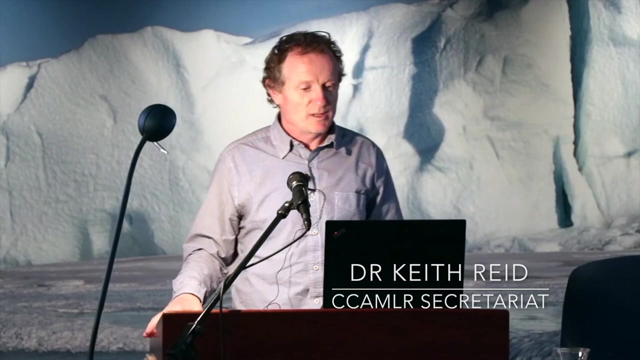 into the future And also In the ecosystem. there is also a fishing boat there which also behaves like one of the predators on krill And that's the end of my talk. I'll hand it over to Keith To start off with. so mentioned about the krill fishery and I just want to give a quick. 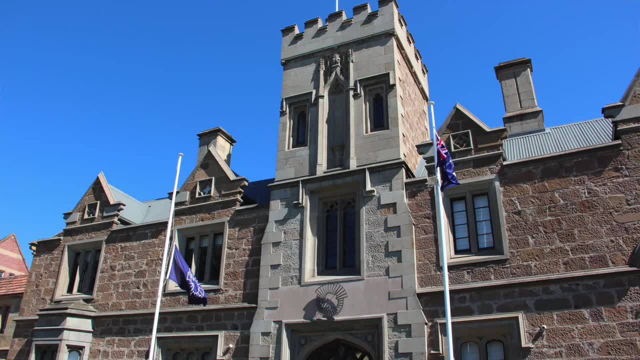 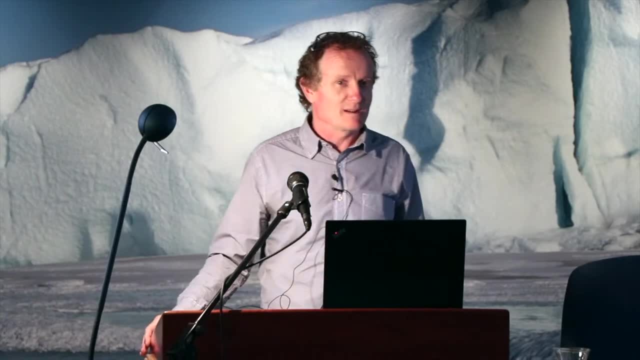 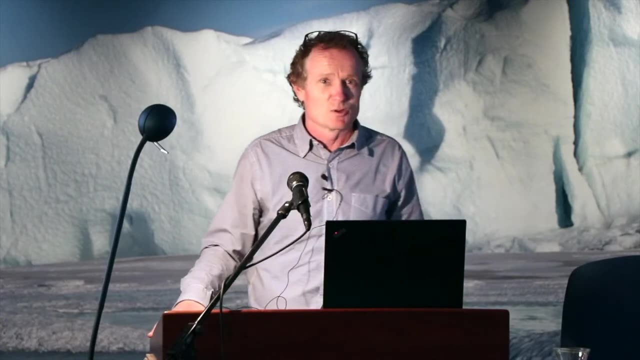 breakdown of what goes on from this building in terms of managing the krill fishery, And to start off with just a quick description of what CAMELAR is: apart from being a sort of difficult acronym, It's the Commission for the Conservation of Antarctic Marine Living Resources. 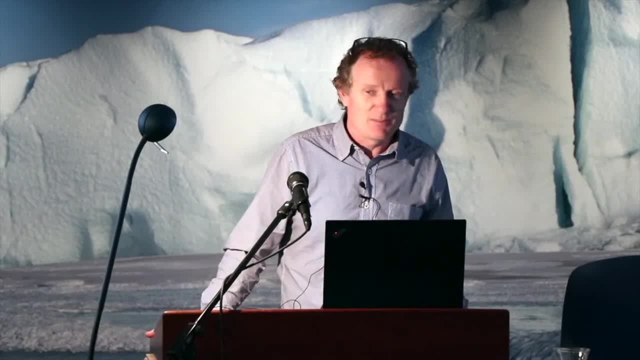 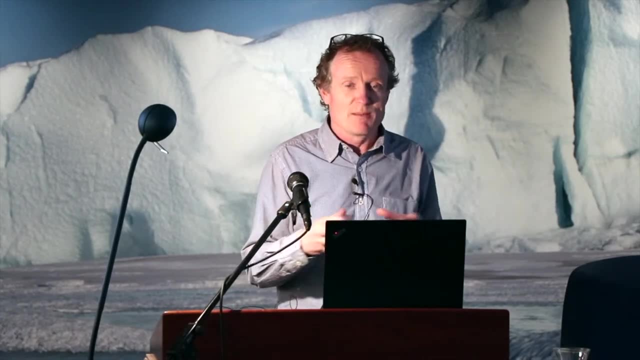 And it's. I did a little thing on ABC radio last night and I described how the members, the member countries of CAMELAR. there's 25 member countries of CAMELAR. it's an international commission. The 25 members' flags are above you here. 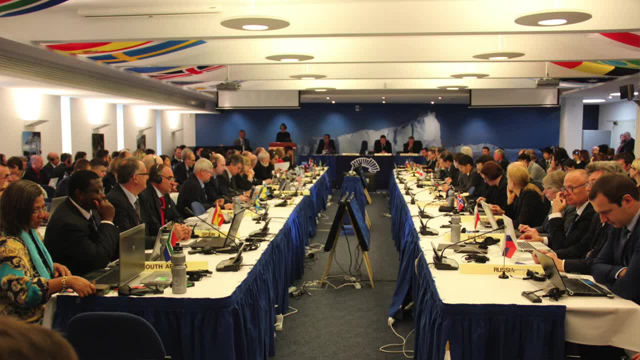 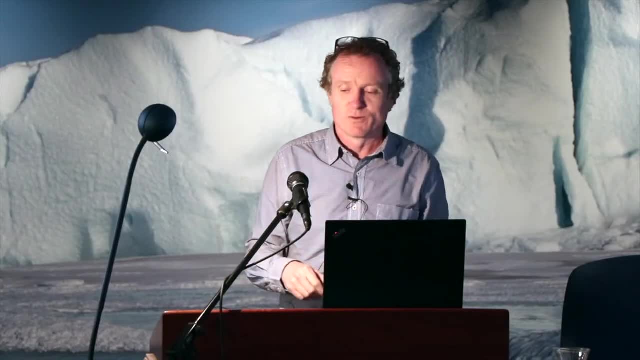 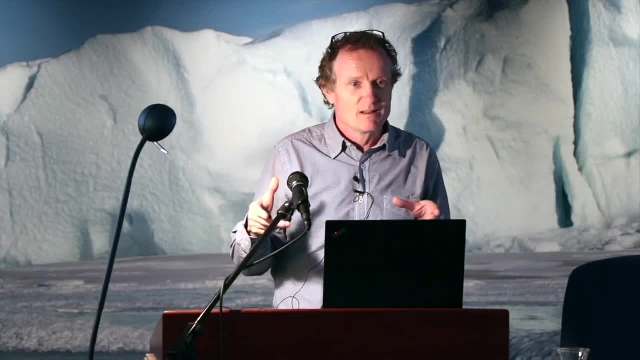 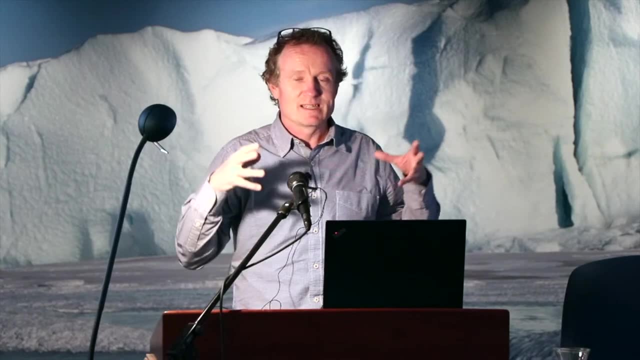 And we described it last night a little bit like the parliament of krill. So all the countries that manage the krill fishing come together and make decisions. They're not always easy to make, but it's an international commission. It's based here in Australia, but it's not an Australian entity. 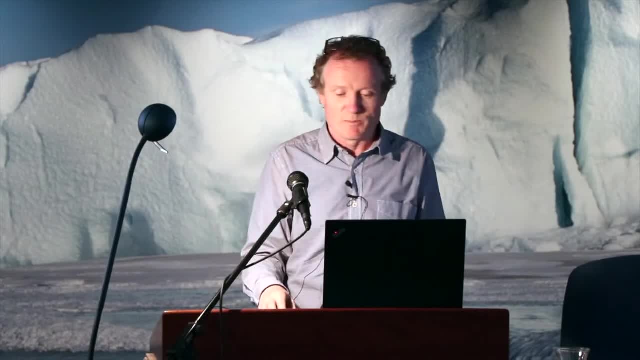 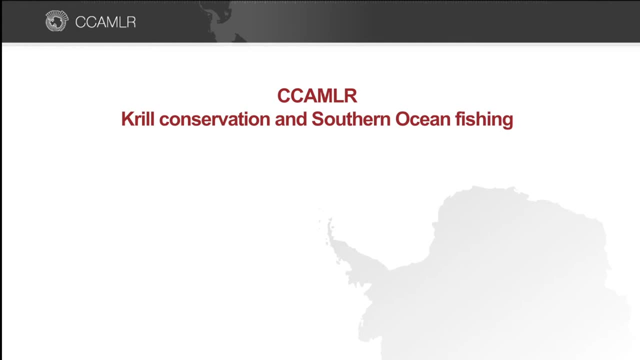 So it's an international commission, Australia, of course, A very important part of it. So what I'm going to talk about is the krill fishery. a little bit about the krill fishery, a little bit about how it's actually managed. 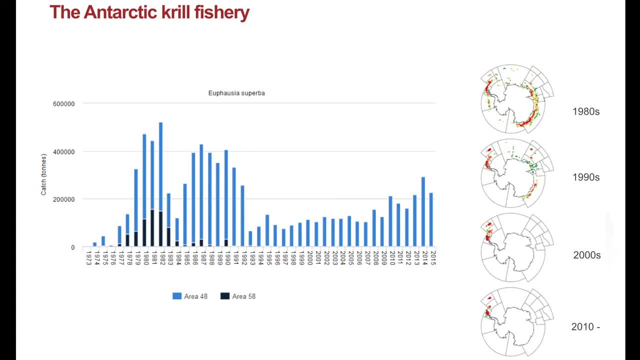 So this is a sort of one slide history of the Antarctic krill fishery. In the bar graph shows the catches in each year in tonnes. You can see it started in the 1970s and has progressed up until today. The maps on the right hand side. 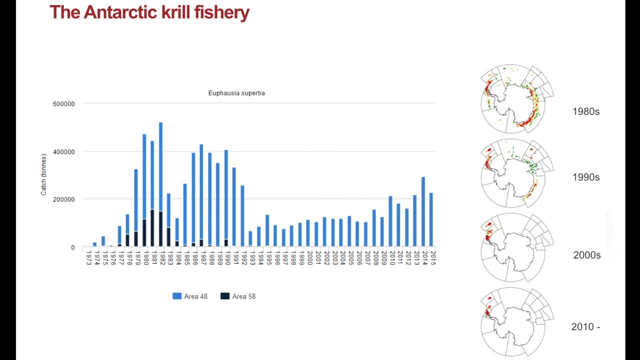 Show where that fishery has taken place. The sort of red colour shows there's more catch, the greens a bit less. And on that bar chart you can see we have area 48 and area 58. The zone that Camelot manages in those maps it's about 10% of the world's ocean. 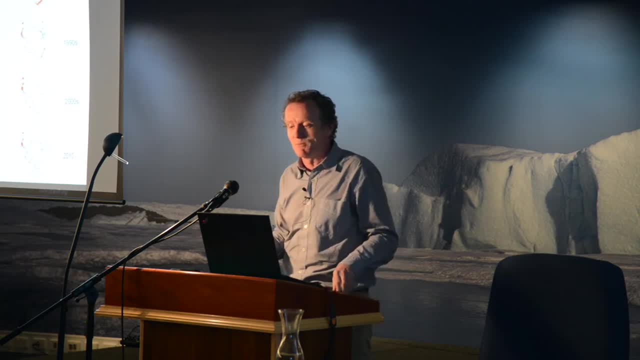 So we divide it into different chunks to help be able to manage it. Area 58 is basically the bit on the right hand side in East Antarctic, And area 48 is on the left hand side And the bit around the middle And area 48 is on the left hand side. 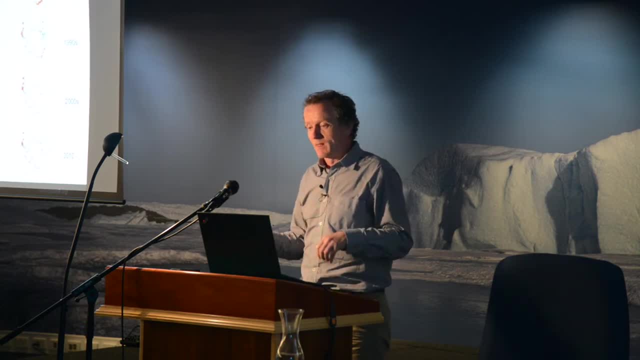 And the bit around the Antarctic Peninsula and the SW Atlantic. When the fishery started it was predominantly the Soviet Union and also to some extent Japan, but predominantly the Soviet Union. And that big change from the 1970s, 1980s and the early 1990s. When you see that big change and then the much lower catches afterwards- That was the breakup of the Soviet Union- Japan continued to fish for krill along with some other nations the 1990s, In the mid 2000s- you can see that the catches started to go up again. that was. 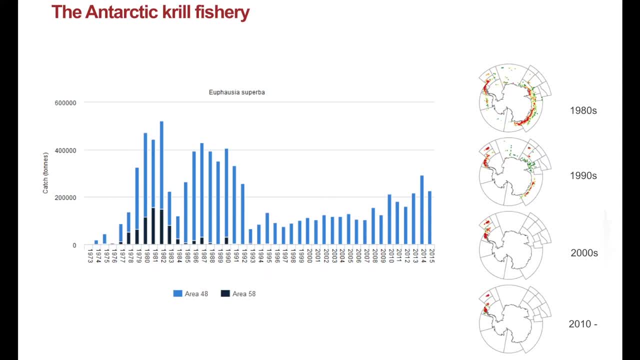 predominantly with the entry of Norway into the fishery and also to some extent China, And you can see that over that sort of time scale the fisheries operation has moved from being somewhat circumpolar and in the East Antarctic to almost now almost solely operating in that area. 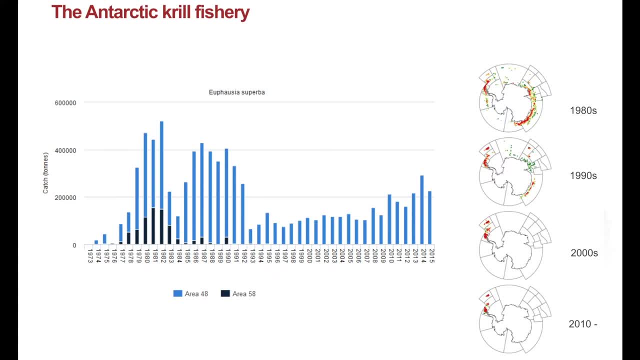 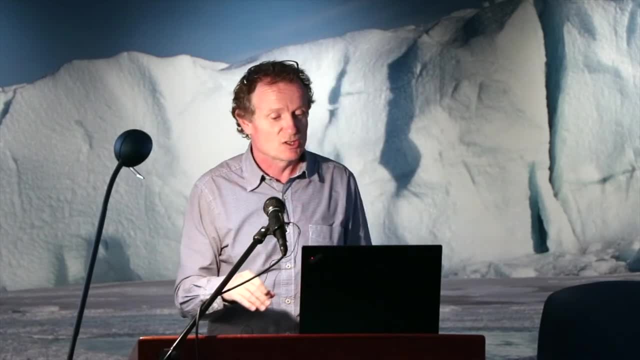 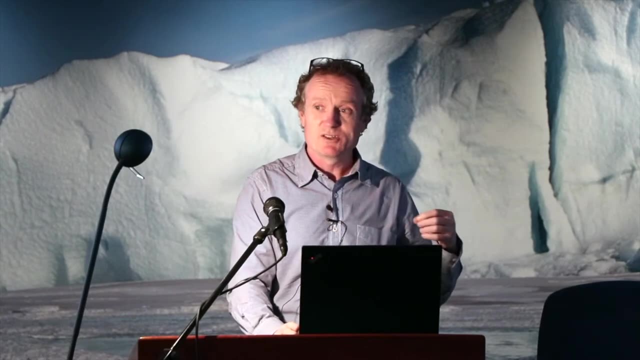 in the South West Atlantic and so in the last decade the fishery catches have increased but the area of operation to some extent has decreased. So that's a very potted history of the krill fishery. so there's been changes in the catch levels, changes in who's taking the catches and changes. 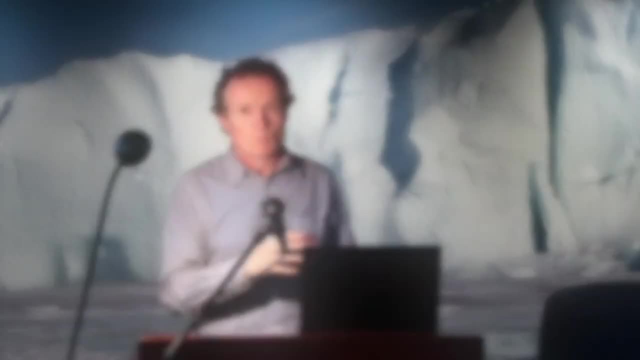 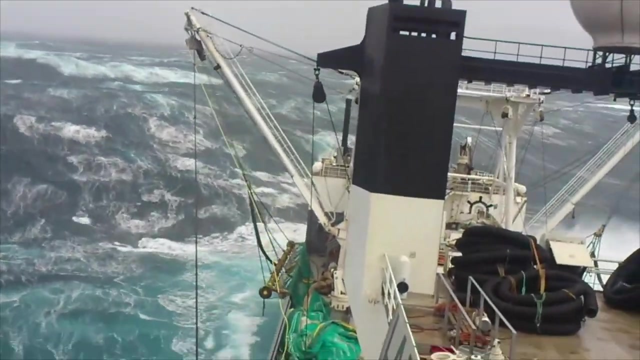 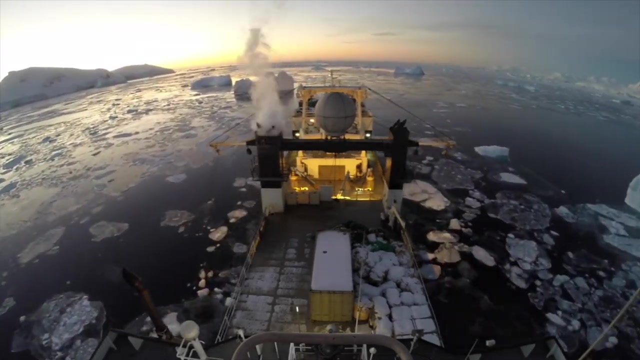 in where those catches have been coming from. When the fishery started, it was basically a free-for-all: there was no catch, There was no management regime in place, and it was that recognition even then- so he's been talking about that central role of krill in the ecosystem- that led to a concern that 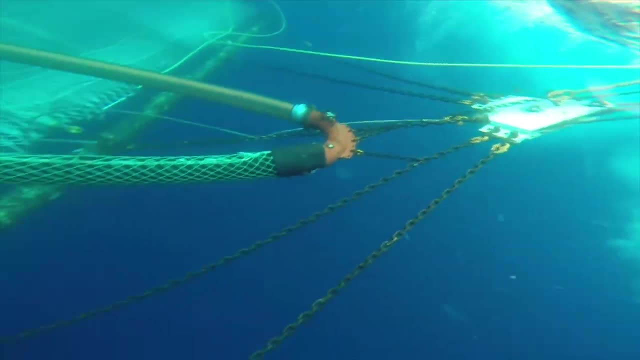 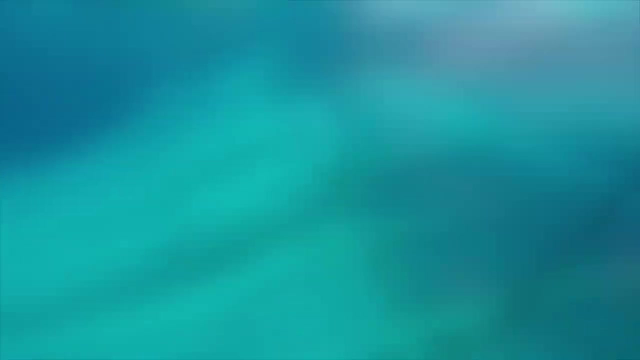 if the krill fishery started and increased pretty quickly, if it went the way that lots of other fisheries have gone, where they start off, increase pretty quickly and then just collapse, that would be pretty catastrophic for the whole of the Antarctic food web. So it was that concern. 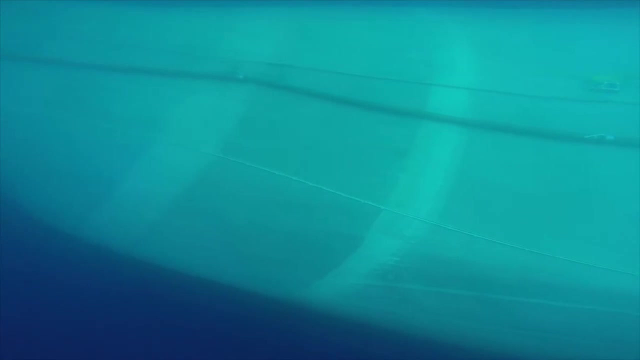 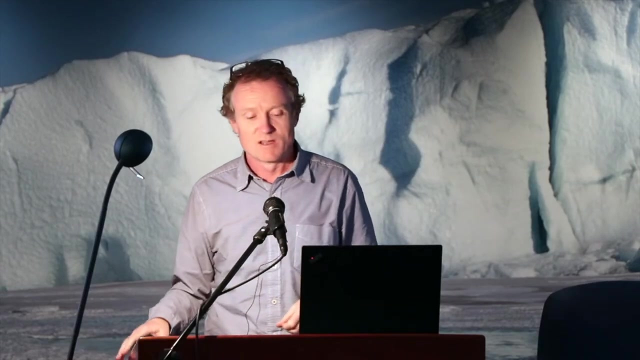 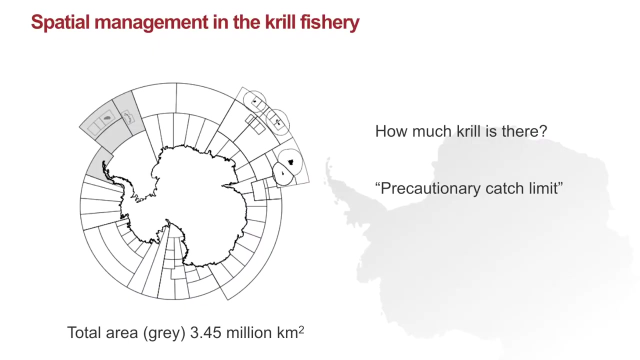 that led to the negotiation of the convention which established Camelar as the body to manage fishing in the Antarctic, and at that time it was very much focused on becoming the krill parliament. well, it wasn't really, but that was the. the emphasis was on managing krill And because the krill fishery now operates almost solely in 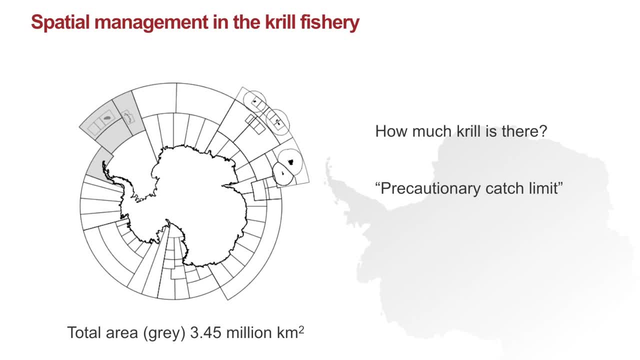 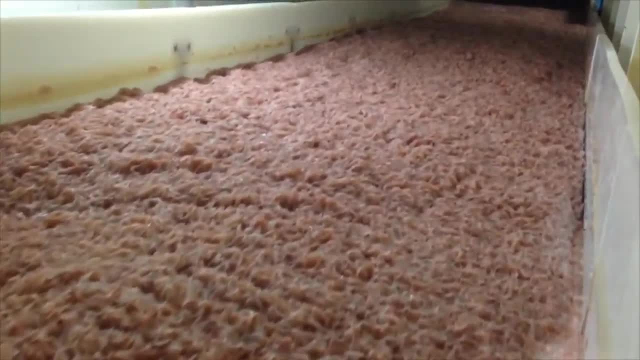 that area in the South West Atlantic. you can see on the the plot. here is the area shaded in grey. in order to manage the fishery in that area, the first thing you need to know is: well, how much krill is there? How much krill is there? 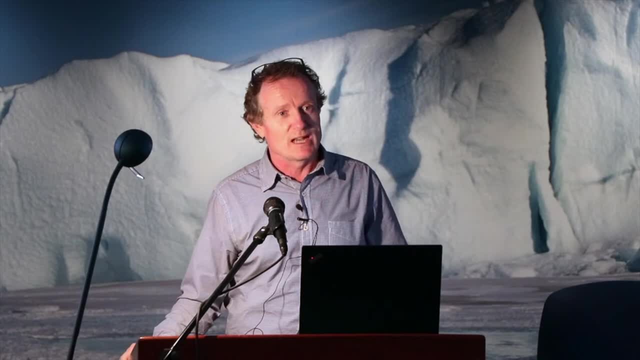 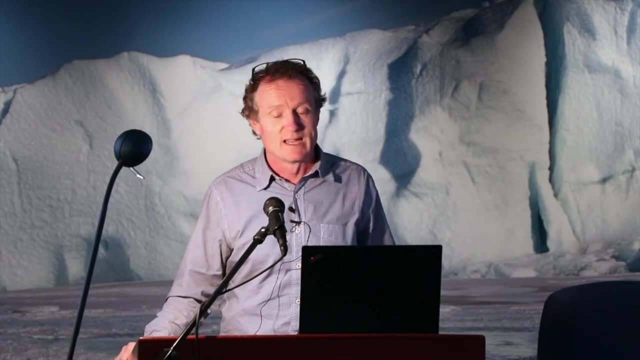 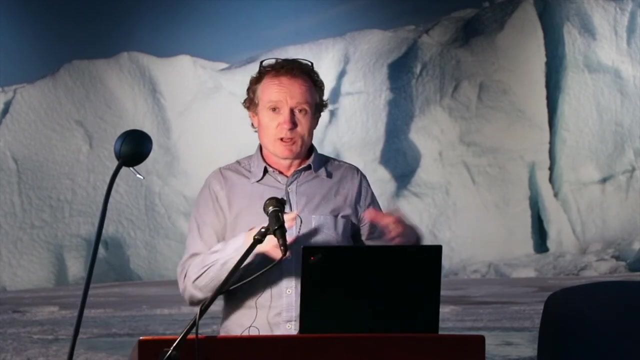 And that's a that's a pretty major undertaking, it's a very large area and actually the last major survey was a multi-vessel, multi-member multinational survey in 2000 which surveyed the whole of that area in grey using shipboard acoustics. and although that 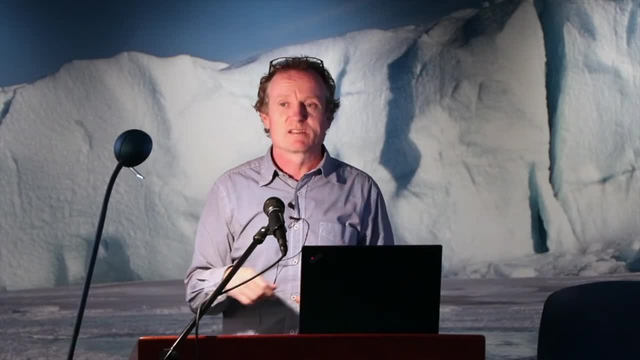 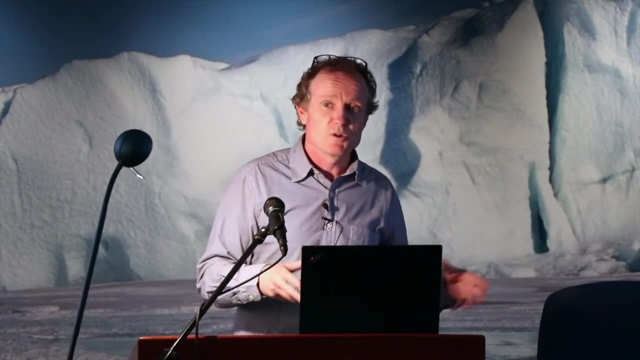 was quite some time ago. there are smaller scale surveys done almost annually in that area that show there hasn't really been any change in the krill abundance since then, Contrary to what you might hear or what people might think. it's a very large area and it's a very large area. 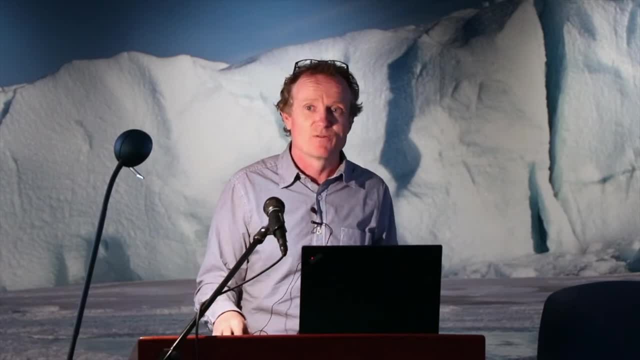 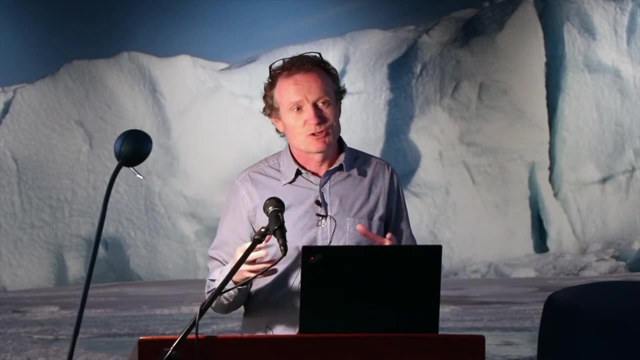 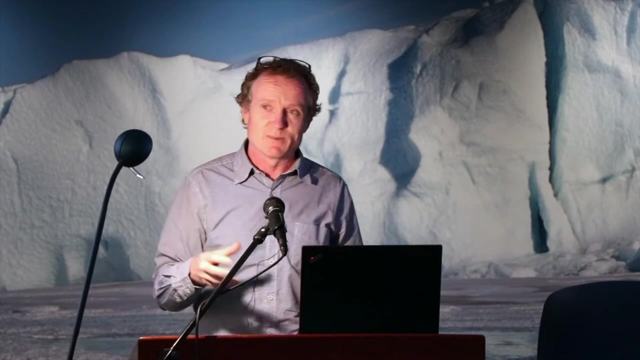 or what people might suggest. there really isn't any evidence for a major decline in krill at all in the in the last two decades. So once we know how much krill is there, we can go up about a process of setting a precautionary catch limit. and the reason I say precautionary catch limit is: 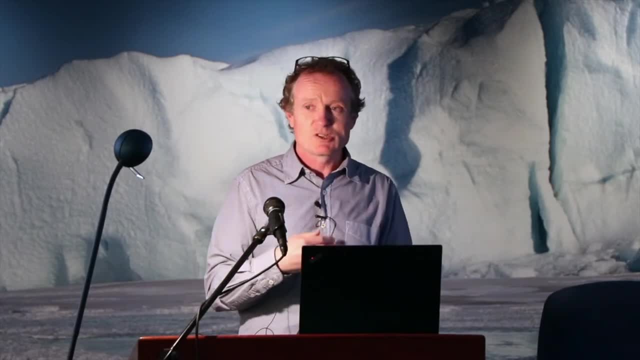 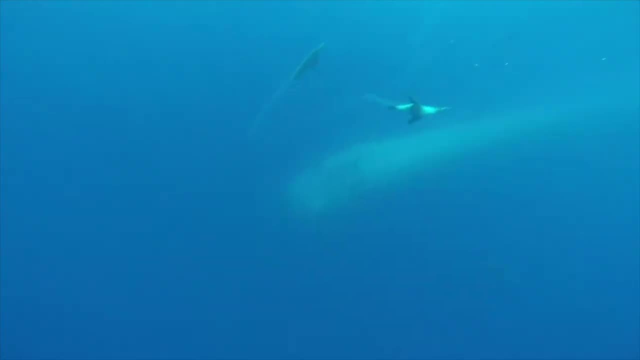 because of the way that Camelar was set up. It's not just about managing the fishery. it's about managing the impact that that fishery has in the ecosystem within that fishery takes place. recognising the importance of krill. it's about making sure that we don't have an impact on the. 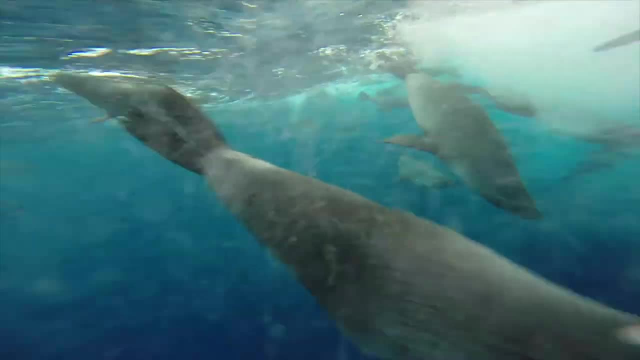 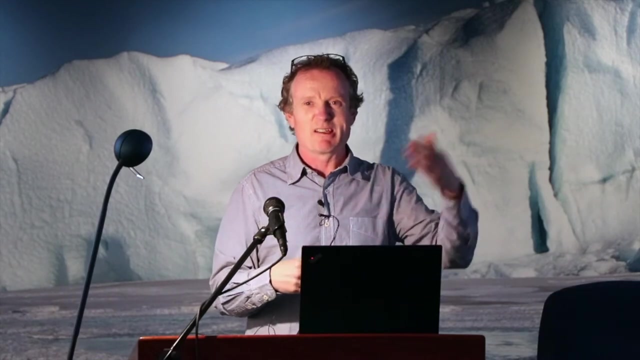 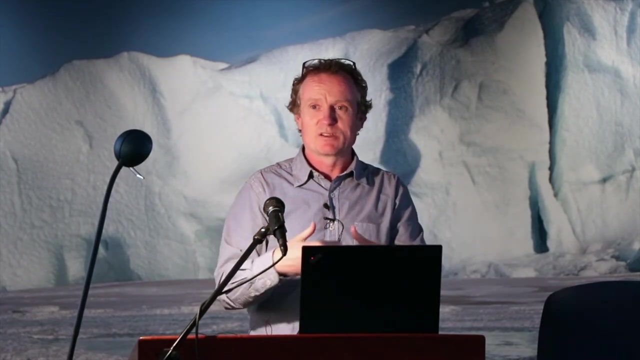 penguins and the seals and whales that also need to feed on that krill. And so we have a precautionary approach, which means that, rather than setting catch limits high and then seeing if it's a problem, set them low and then the fishery can expand if we get the data to understand that. 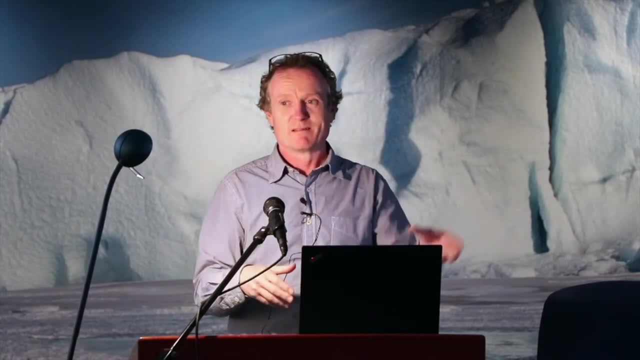 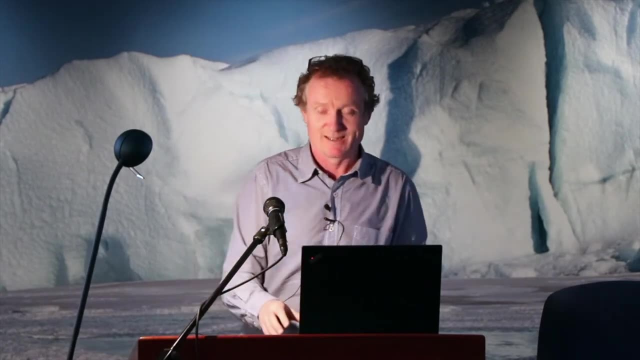 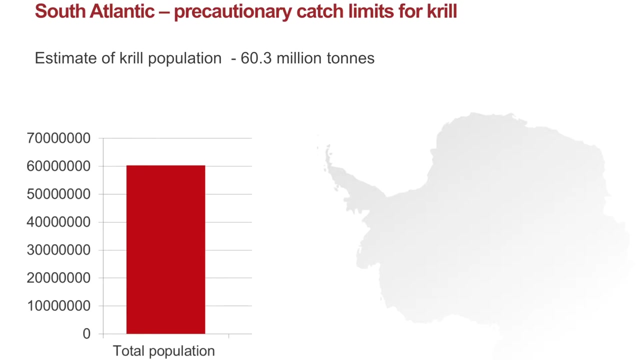 that expansion is going to have an effect, rather than setting a very high catch limit, realising the problem and then trying to fix it, which generally in fisheries and in life doesn't work quite so well. So from that survey in the area of the Antarctic we have an estimate of 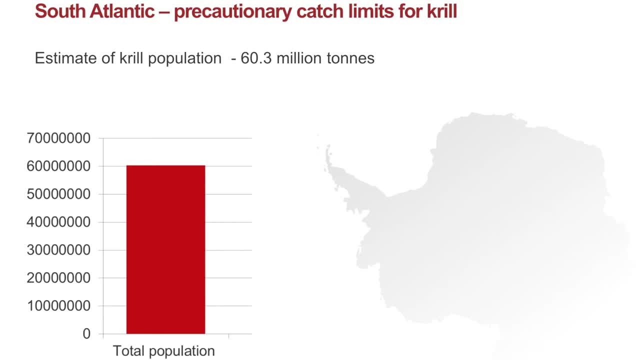 about 60 million tonnes of krill And through a series of mathematical models and computer simulations we can run different simulations to see, well, what would be the effect on the krill and on the dependent predators of different levels of krill. 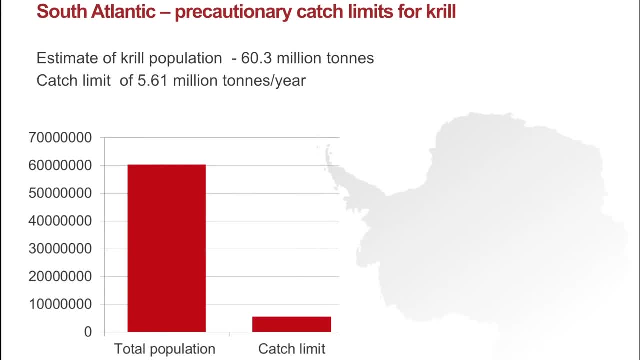 Catch And I won't go into the detail of that process. It takes a long time, but a lot of people are a great deal cleverer than I am doing it. But we come up with a catch limit. that's about 9%. 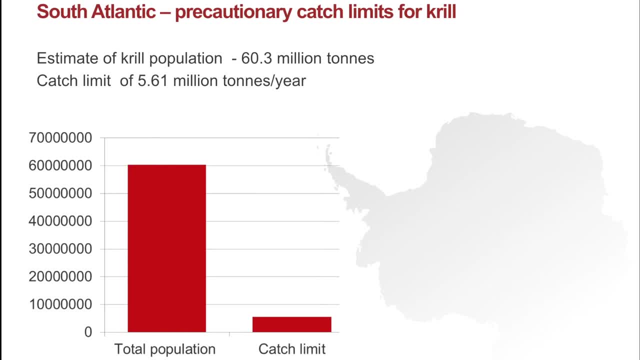 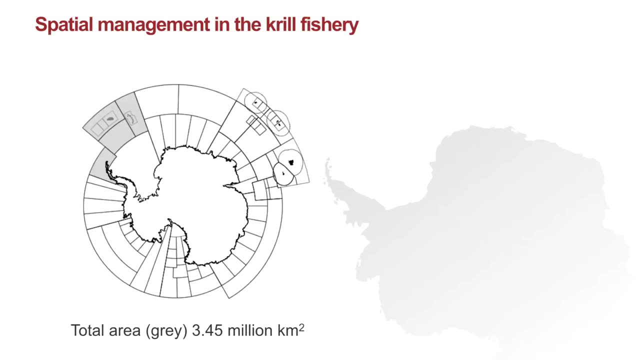 of that population And it's about 5 million tonnes per year. So that's a catch limit that you could take from that krill population that we think wouldn't impact the krill population and it wouldn't adversely impact the predators that feed on krill. But you'll recall that 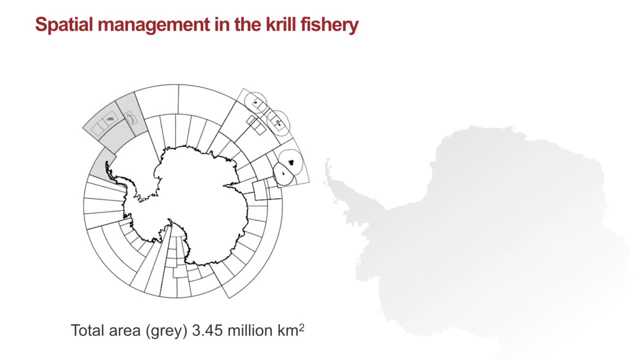 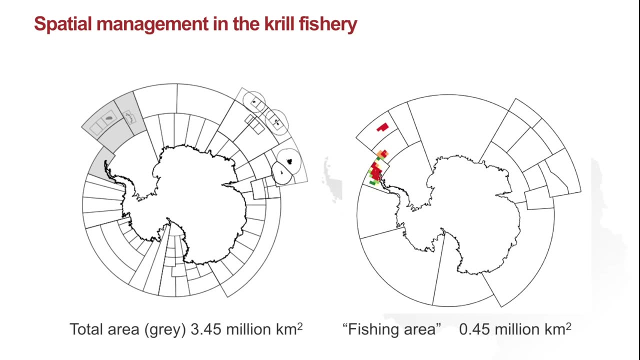 that's a very large area And the fishery itself only actually operates in a relatively small part of that area And, kind of unfortunately, the fishery tends to operate just in those areas that are close to islands or to land masses which are really good for penguins to have their colonies on, And 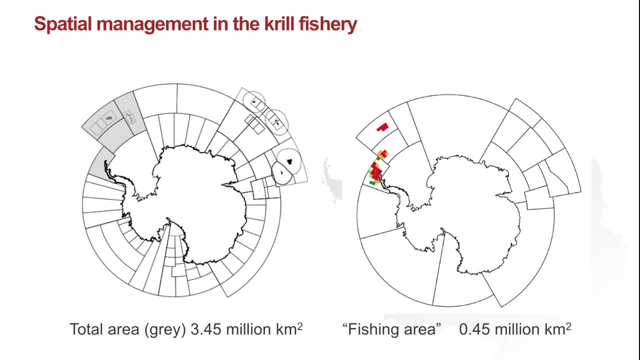 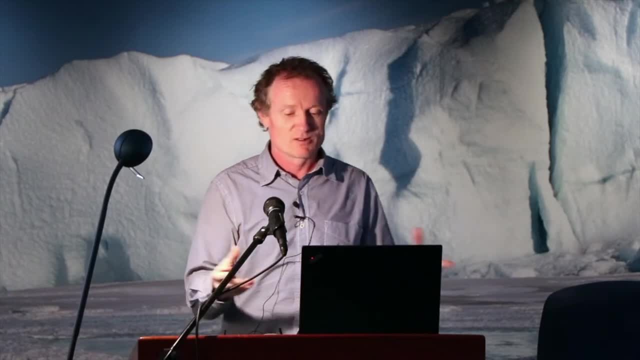 it's also where we know that lots of seals and whales aggregate in those areas. So, unsurprisingly, the fishery operates in the same areas that the predators like to go to that feed on krill, because they're all basically trying to do the same thing. But it means that you. don't want the whole of that 5 million tonnes taken from just one of those small places. If it's spread out evenly it might not have an impact on the krill population or those predators, But if you took it all from one place then the likelihood is that it would. 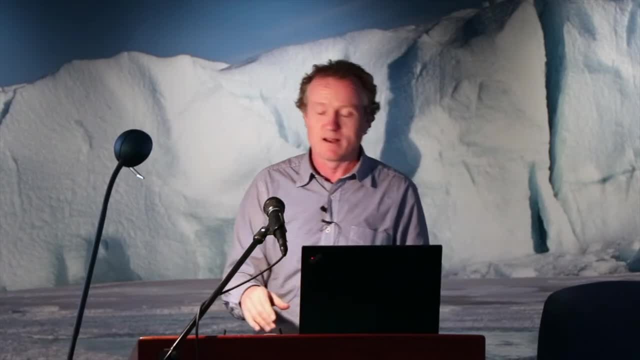 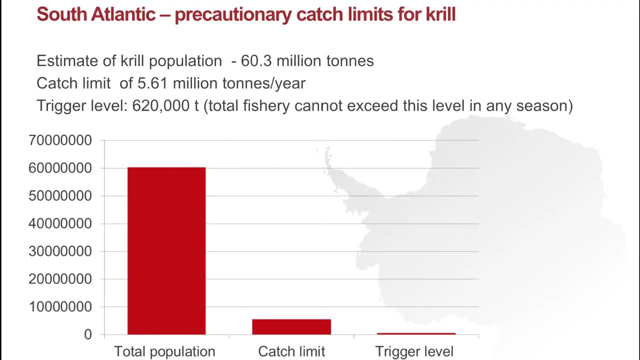 have the sort of effect that we certainly don't want to see in our management approach. So what Kamilar has done is said: until there's a way of making sure we can spread out that fishery, to make sure there's not a localised impact anywhere, we're going. 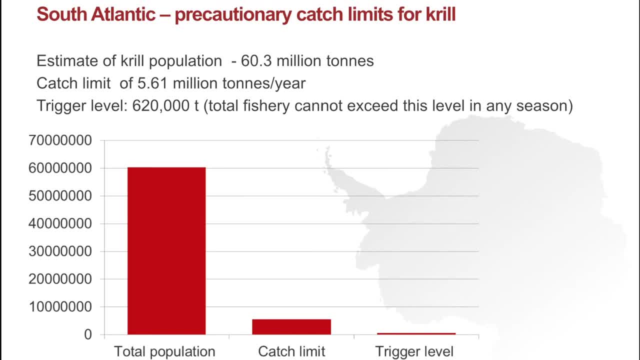 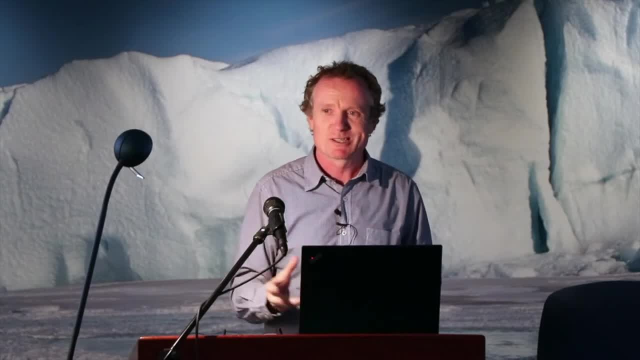 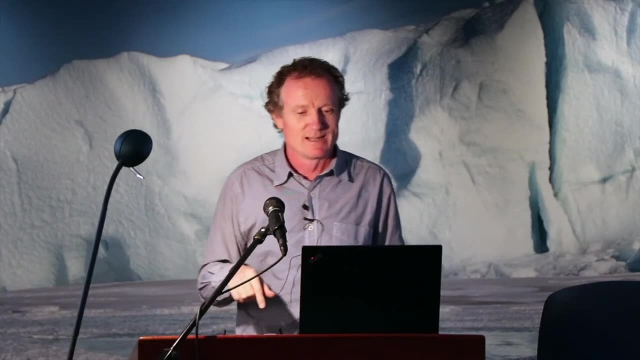 to cap the fishery at 620,000 tonnes. Now 620,000 tonnes has some historical basis. It was also sort of mashed out in some political discussions and darkened smoky rooms way back in the day when Kamilar didn't meet here, they met at Rest Point Casino. I was still 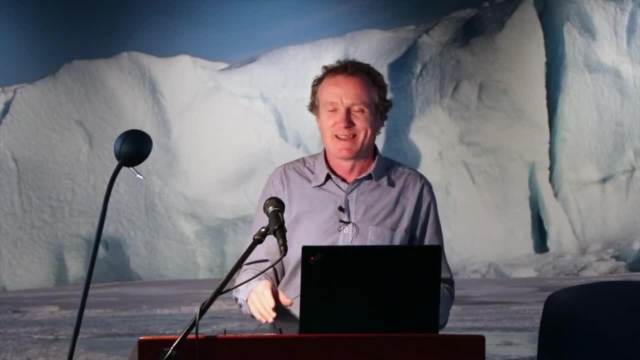 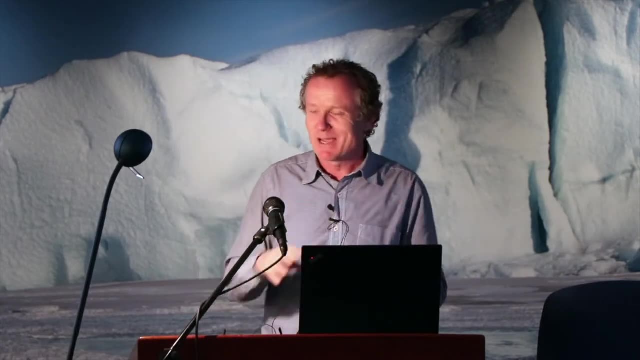 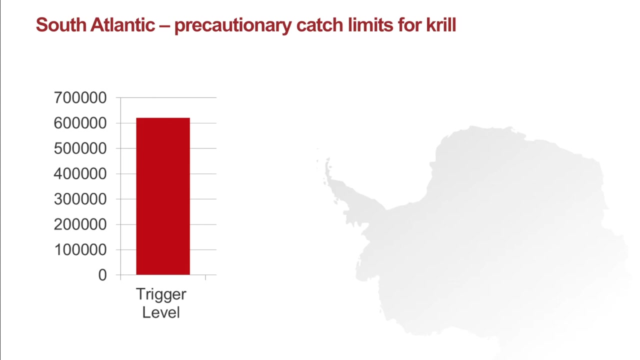 at school then. so I can't take any credit or blame for anything that went on then, But some people in this room who were there And they know who they are. So we have this cap on the fishery at 620,000 tonnes and just to ensure that even that 620,000, 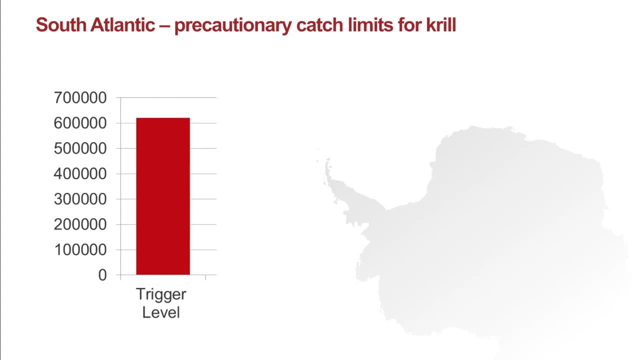 tonnes isn't taken in one place. so we call that the trigger level because it's a trigger. if we went above that we'd have to have a different management system in place. we actually divide that 620,000 tonnes into 3 other portions. You'll recall, on that plot there were 3 areas. 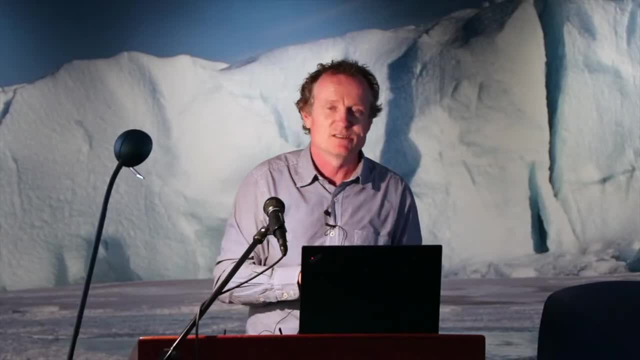 where the fishery was, and now we have 5 other areas where, when we were here, it was all 620,000 tonnes took place and they're around different locations in the Antarctic region: that Southwest Atlantic, around the islands of South Georgia, the South Orkneys and down. in the Antarctic Peninsula. In the last few years that catch limit in the Antarctic Peninsula has been reached, I think maybe in four or five of the last in the last four or five years. This year I think we closed that fishery on the 1st of July when the fishery reached that catch limit And reaching a catch. limit sometimes in a fishery, starts to spark concern in people. well, the fishery must be- must be getting too big. But actually the way that this is being managed, from that 60 million tonnes to start with, to a catch limit of five million tonnes, to something that's a hundred and fifty five thousand tonnes- 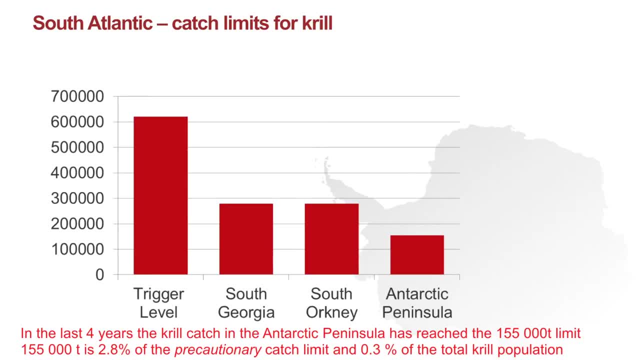 Actually, that hundred and fifty five thousand tonnes is only 0.3% of the crew population and I have to admit that with the best will in the world, we're not. we aren't able to measure the size of the krill population to within 0.3 of a percent. 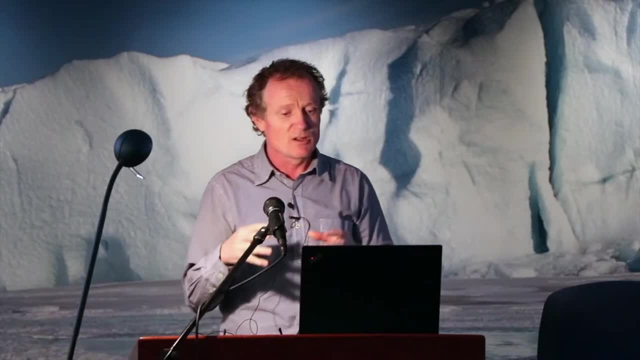 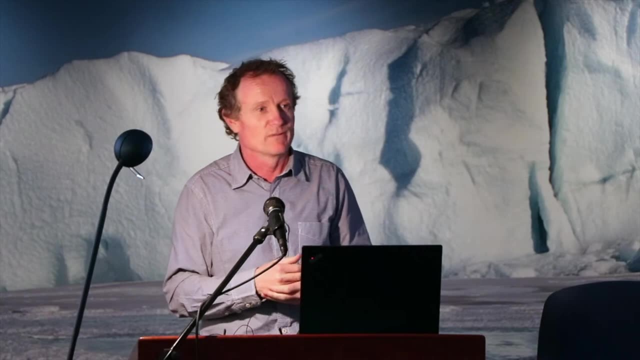 Probably plus or minus 20%. So at the moment, and obviously the big question a lot of people ask me and anyone else involved in the krill fishery is: is it sustainable? Are the catches of krill that we're taking at the moment? 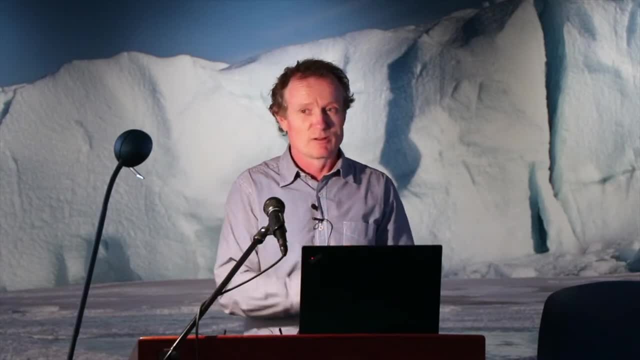 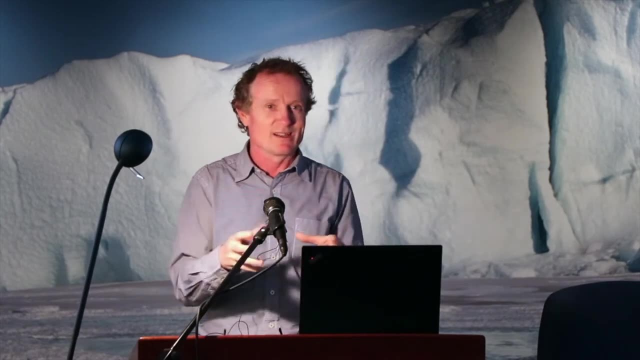 sustainable, And I would say that if the catches of krill that have been taken at the moment are not sustainable, given our current understanding of that ecosystem, then just about all of the scientists who worked on krill over the last 30 years have got it wrong, And I'm pretty. 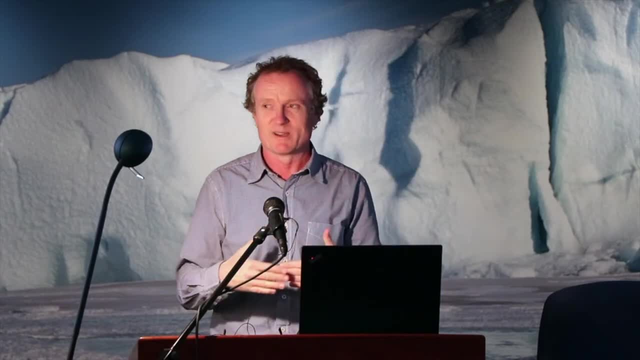 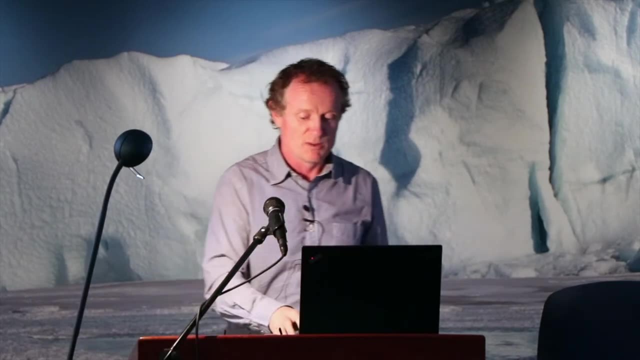 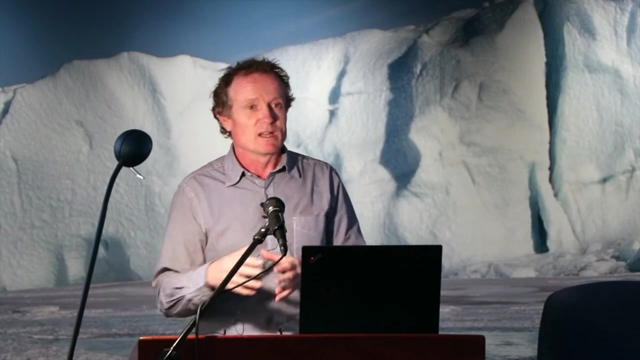 confident that they haven't. So I would say that at the moment the catch levels for krill are sustainable. That doesn't mean we can be complacent about the future, but at the moment the catch levels are really very small in comparison to the size of the population. But in terms of managing a fishery and 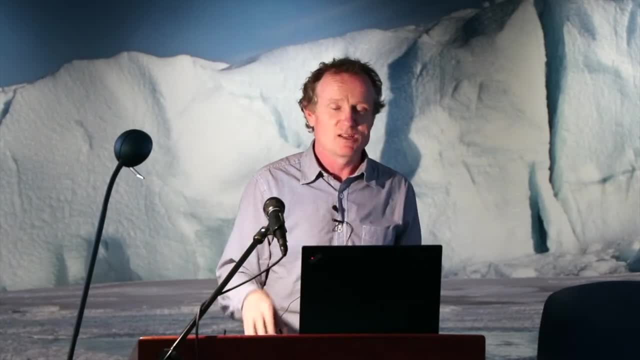 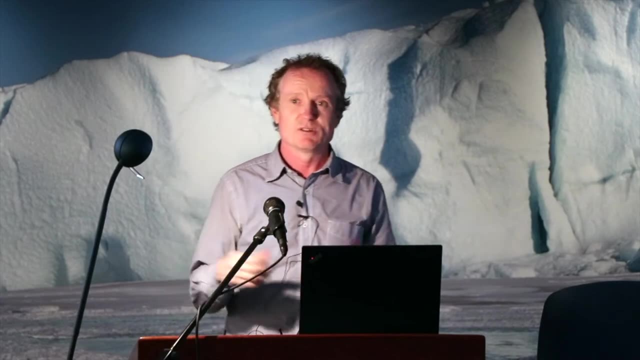 sort of the operational elements of managing a fishery. it's not just about setting a catch limit. You need to know what's actually going on in the fishery and day-to-day. this is the sort of information that flows from the Antarctic into this building so that we can manage the krill. 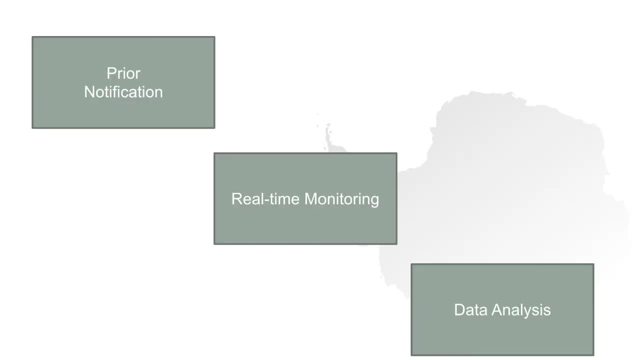 fishery, The first thing that we need to do is know who's going to be there and who's going to be taking part in that fishery, And only members of the Commission, so only the people who can fly one of these flags can fish for krill. 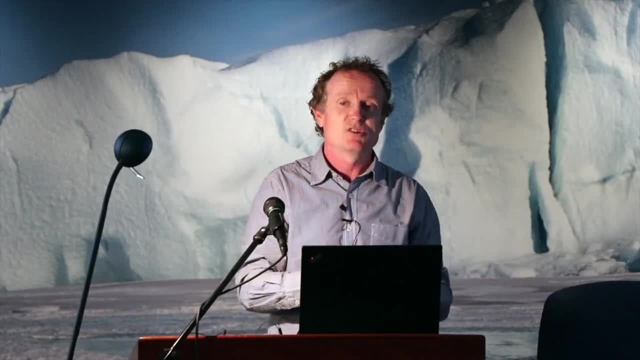 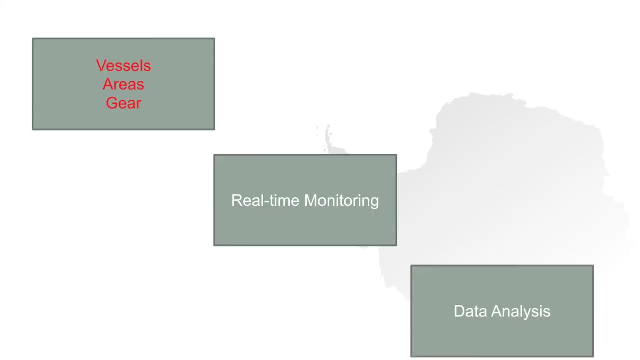 And in order to do so they have to give prior notification the year before. So we already know which vessels are authorized to fish for krill next year. So as part of that, we need to know which vessels, which areas, they've asked to go. 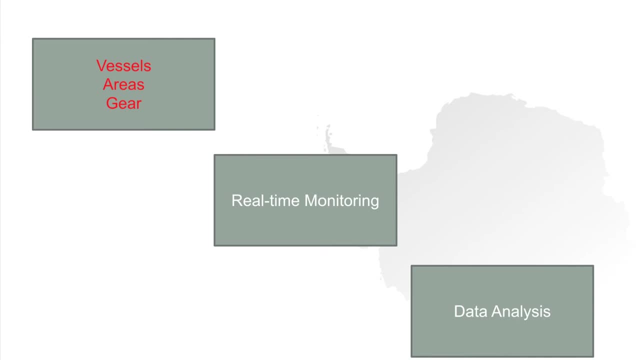 fishing in, because it's not just a free-for-all. There's only certain areas that they can fish for krill in, and also what gear they're going to use. So what size nets? All of those nets have to be adapted to have an escape panel in them which allows any fur, seals or other. things that get into the net to escape so we don't catch them, And also vessels that use, if you like, a traditional fishing method, where you pull your net through the water, haul it up, dump it on deck and sort through the catch. Other ones that don't do that. 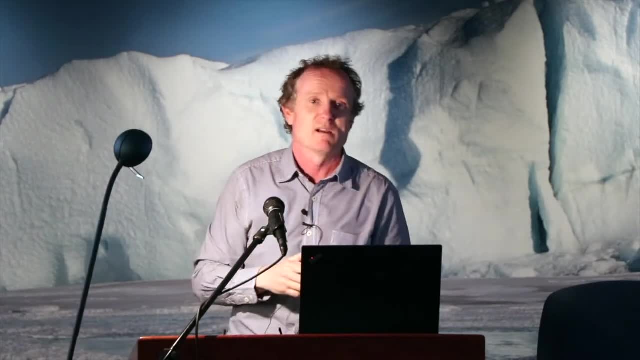 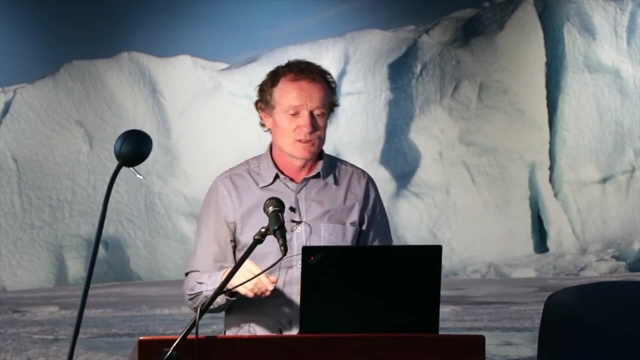 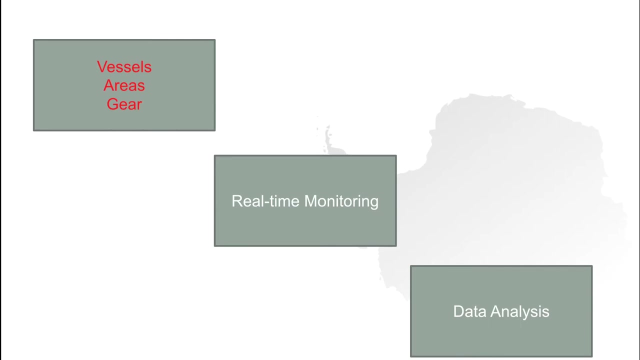 they leave the net in the water but they pump the cod end with an airflow water pump so they're just catching fresh krill on the vessel all of the time. They can leave the net in the water for much longer periods and have a very steady stream of krill coming onto the vessel. So we know which. 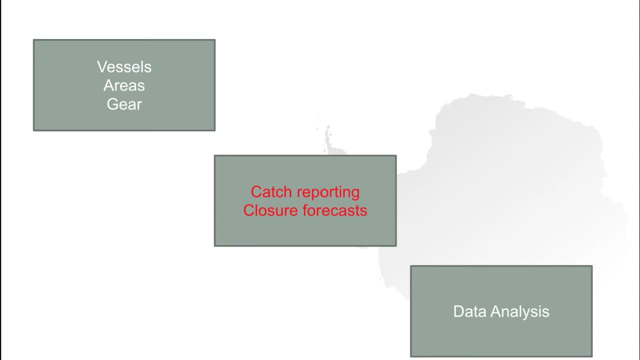 vessels are going to take part. when they enter the Camelot Convention Area They have to send a message to us here to let us know and then we can monitor what they're doing. They have to report their catches when the fishery is quite a long way away from the catch limit. They can report monthly. 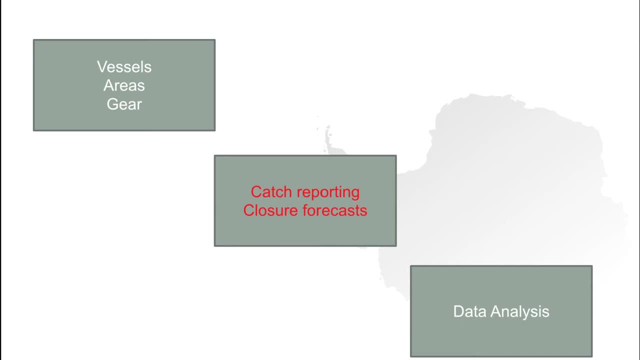 as they get closer to it. They have to report every five days. We have other fisheries that we monitor that have to report their catches to us every day, and then we can see how the catch is progressing towards the catch limit. so we can then notify all of the vessels. 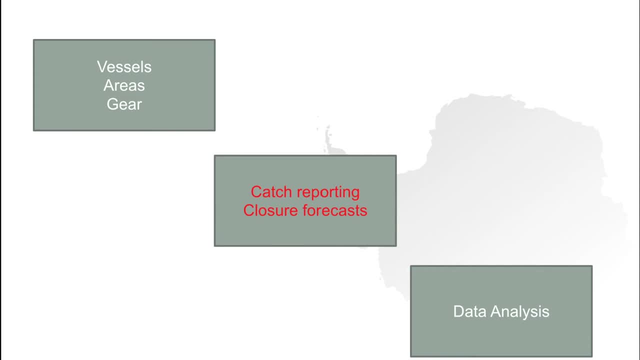 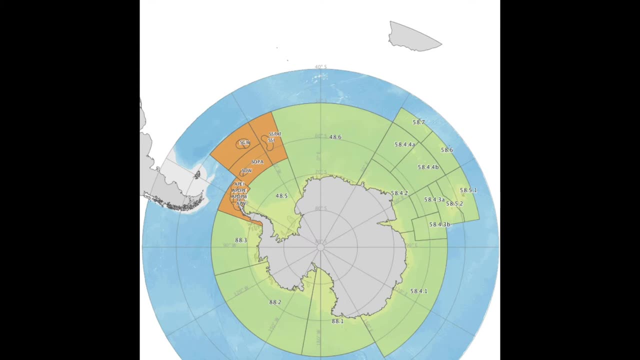 that the fishery is going to close. As I said earlier, we did that for the krill fishery in the Antarctic Peninsula this year. That closed on the 1st of July. All of the vessels have to have a vessel monitoring system, so a satellite linked location indicator. so we know that the vessels 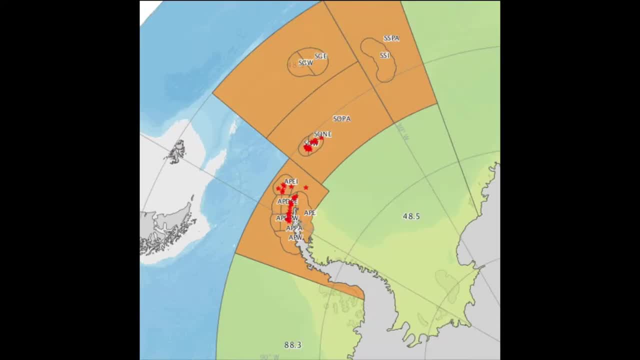 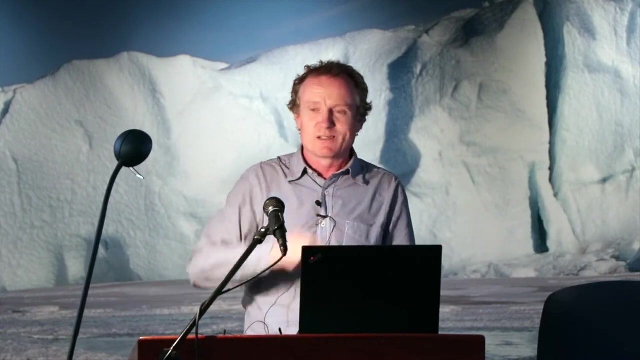 once the fishery is closed, they have to leave the area and we know that we can check up to make sure that they do that. So that's the within season monitoring. and then we get every haul or every time period for the vessels that leave the nets in the water for longer and pump. 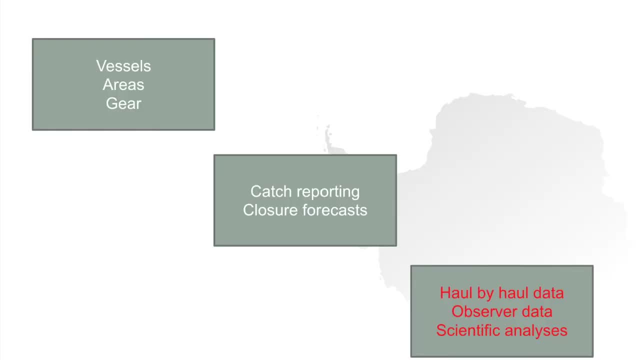 the cod end out. We get information on where and when and how deep the water was and how deep their net was for every haul that they undertake. We also have scientific observers on probably about 90 percent of the krill vessels now will be moving to 100 percent in three years time. 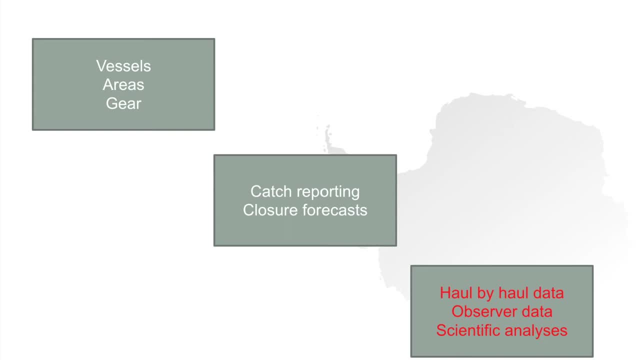 So they're measuring krill, seeing what sex, what stage they're at, Also checking to see if there's any fish by catch that's taken with the krill as well and other elements of the broader ecosystem impacts that that fishery might be having. We bring all that data together in 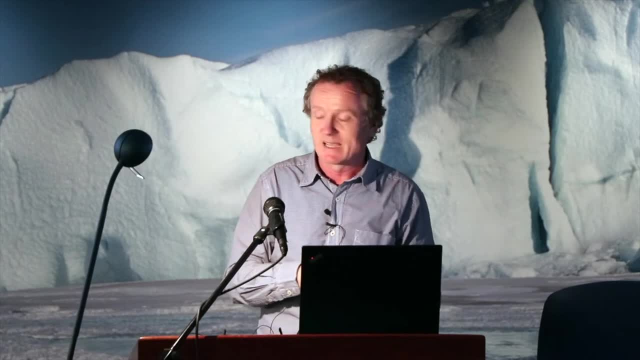 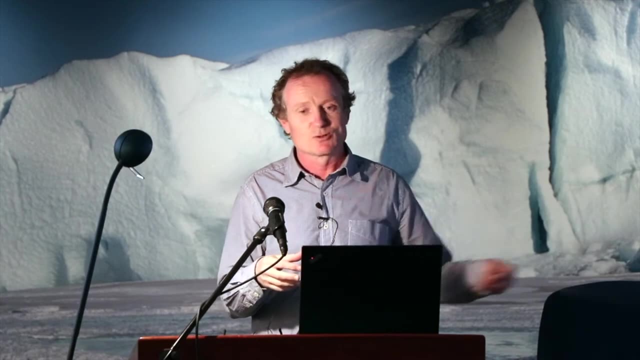 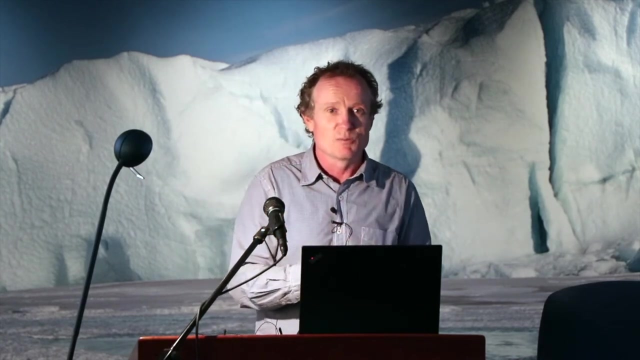 in this building but also in different members are engaged in that fishery, bring those scientific analyses forward. along with that other information about the notification of vessels, who's going to fish, the within season monitoring, and that's the sort of information that we bring together So when the commission meets in October. 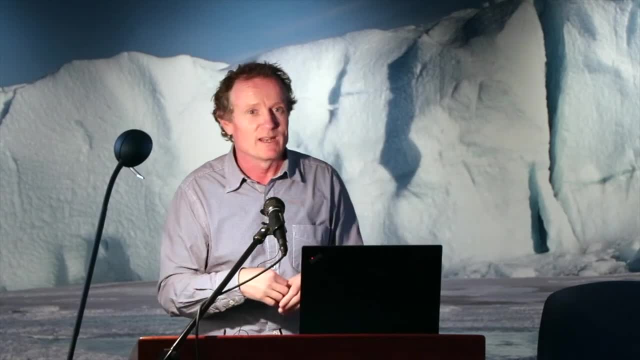 they have the information about who's going to fish and that's the sort of information that we bring together. so when the commission meets in October, they have the information we're going to put together with which to make decisions about how we manage the fishery. So, although the 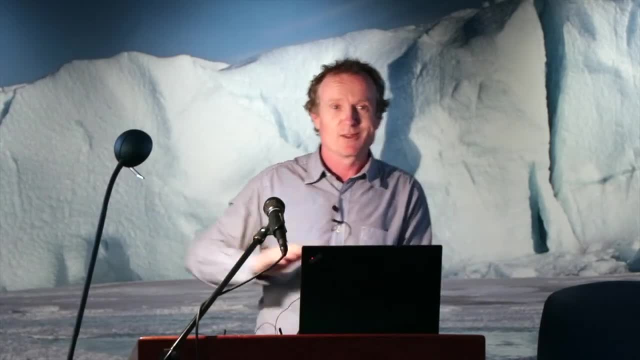 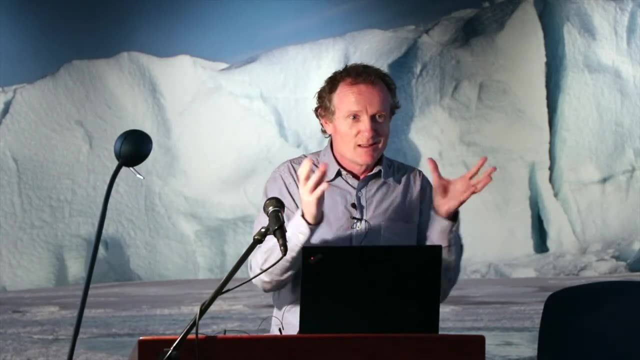 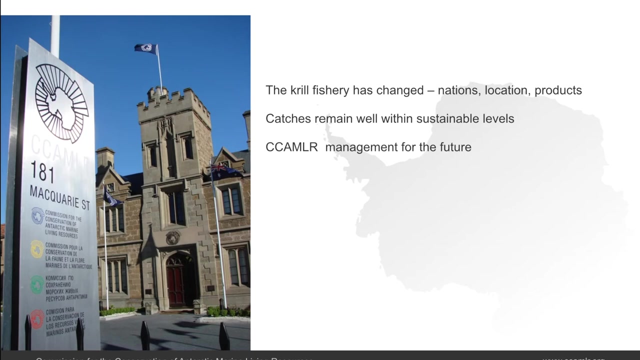 Krill fishery happens an awful long way away from here, right at the other side of the Antarctic. all that information flows into this building. This quiet little building on Macquarie Street is the hub of where the Krill fishery is being managed. One of the key messages, I suppose, is that we know that the Krill 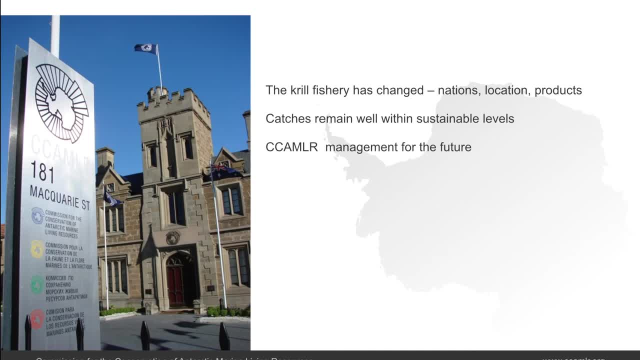 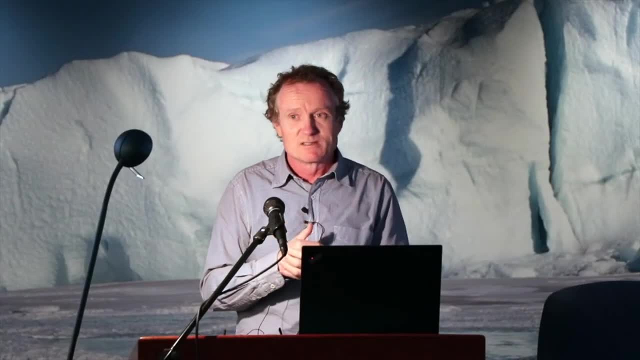 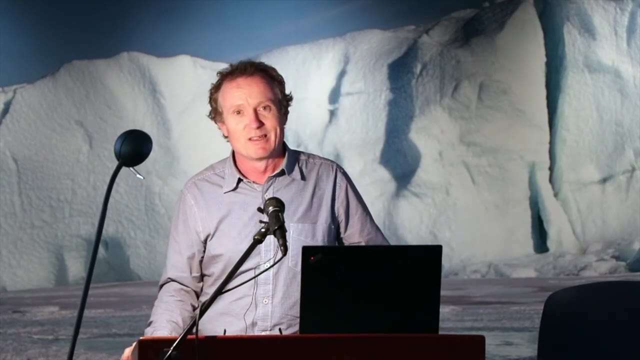 fishery has changed over the time that's been operating different countries involved, different locations, different catches. Those catches are, I would say, currently under sustainable levels or well below sustainable levels, and obviously it's our management objective to make sure that I could stand here in. 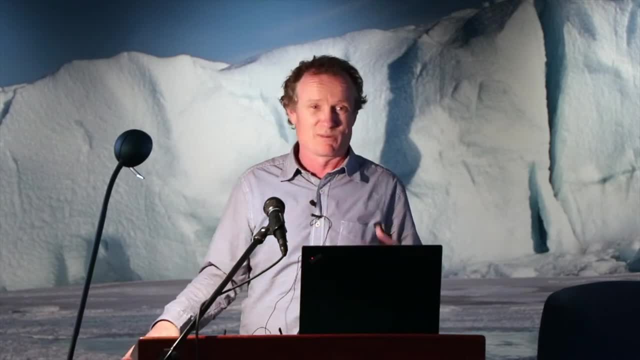 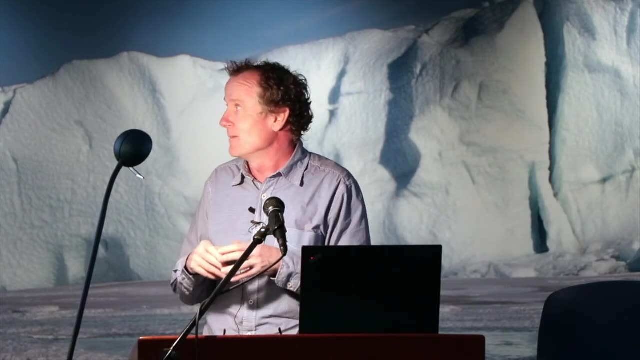 20 years time and say exactly the same thing. well, perhaps not me, but somebody else, But one of the the key things that has changed is that you've got to be able to manage the fishery, you've got to be able to manage the. 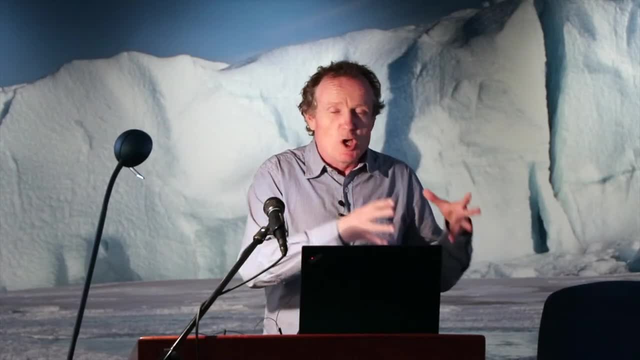 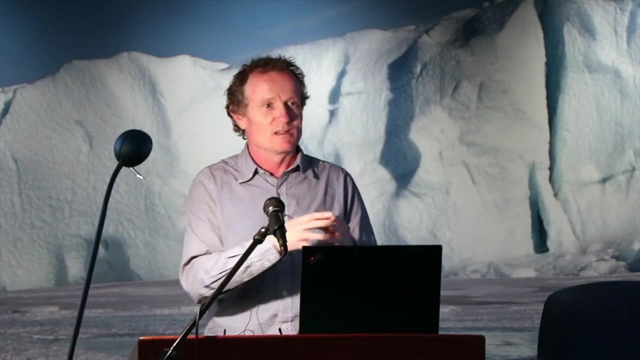 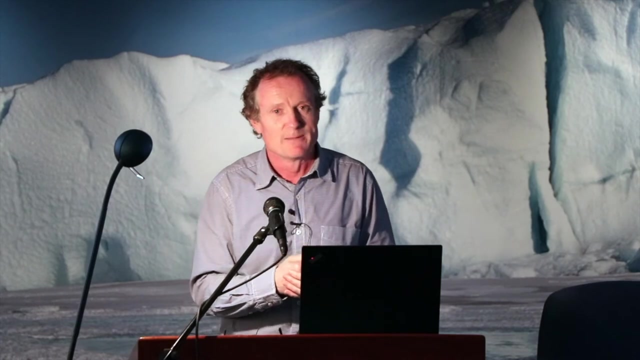 the I guess in the in the early part of the Krill fishery the emphasis was on collecting marine protein to feed the masses, if you like. This was a seen as a big source of an expanding human population and that potentially, this massive source of marine protein and that increased more recently in the. fishery is much more driven by a change in the market for Krill and in particular for krill oil, and that's one of the things that that's changed driven particularly the Norwegian interest in a high-value commercial product, in getting krill oil for the nutraceutical and pharmaceutical markets. 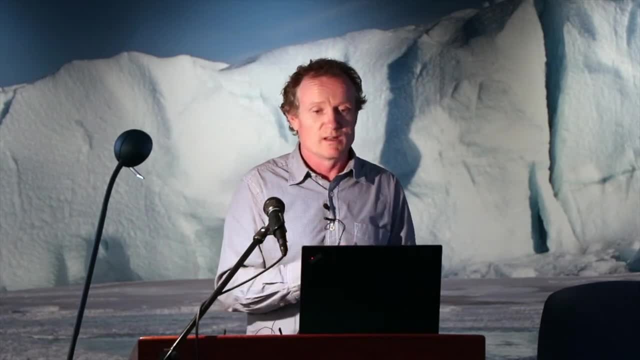 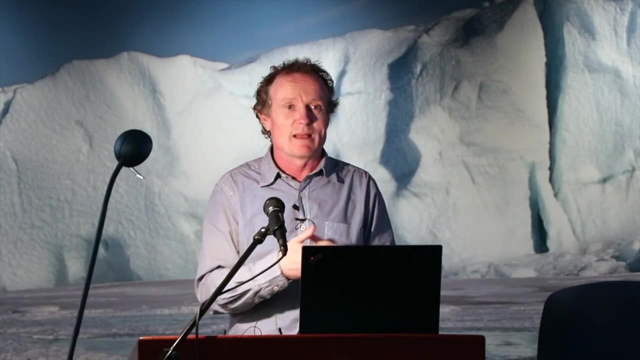 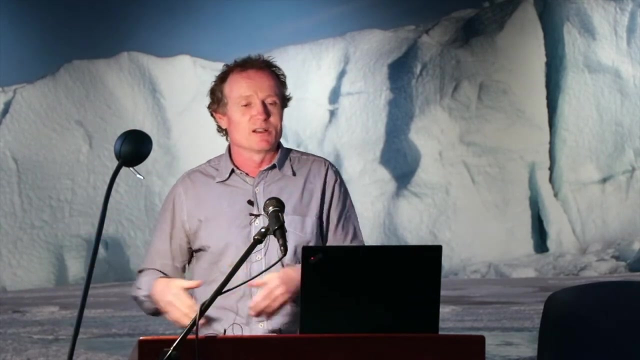 So there's different drivers for an expansion in the krill fishery, but of course we have to be mindful of the sort of work that so has been doing in the longer term about the effects of things like ocean acidification, that we're looking there at, say, sort of 50 to 100 year timescales, where we're probably not. 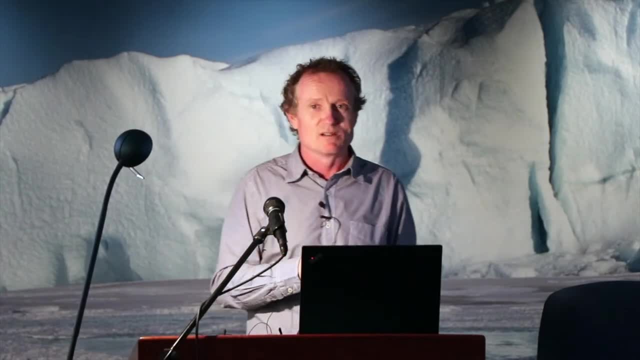 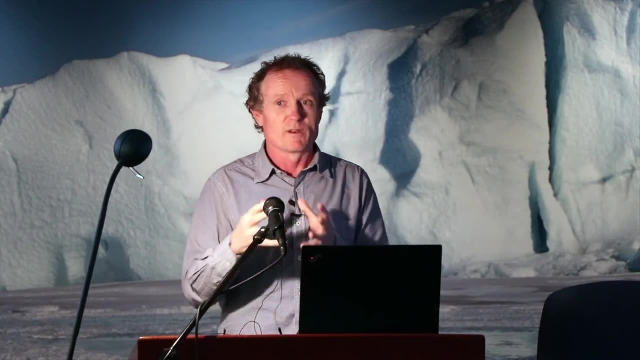 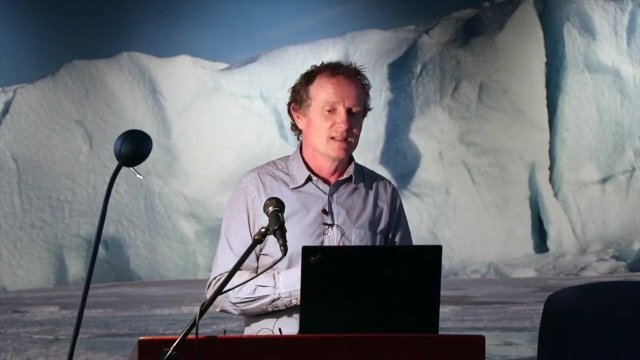 managing the fishery In decision-making at those sort of timescales, but obviously we want to ensure that we have that sort of sustainability in the longer term. but one of the most, I would say one of the most interesting developments is that change in the market towards things like krill oil, and that's the other. 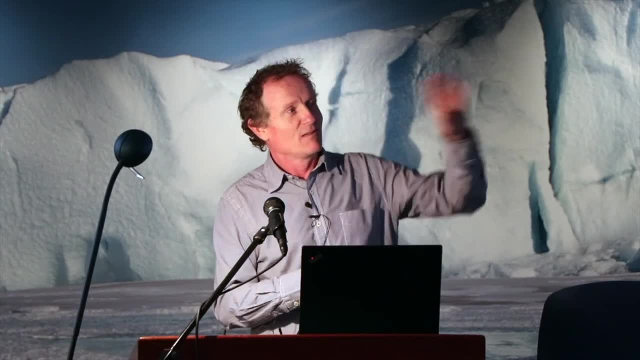 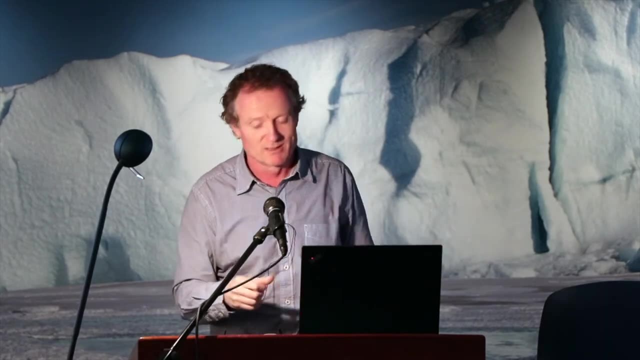 connection that we have in Hobart. so we have the aquarium at AAD doing that cutting-edge research on on what's going, what might happen to krill in the future we have. so if you sort of drive through, you come from Margate or you've. 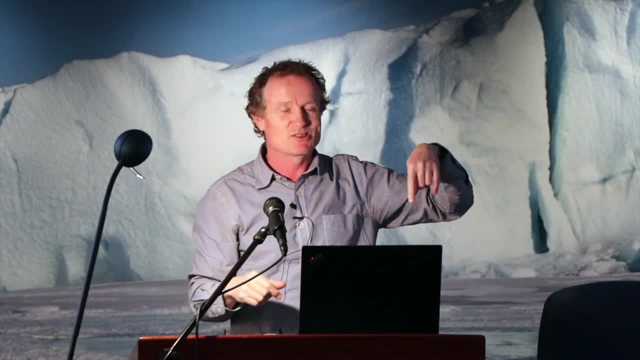 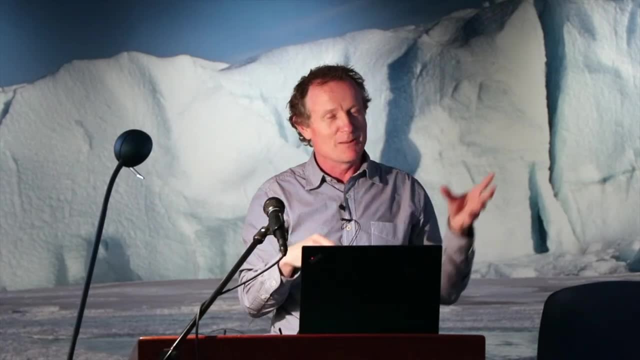 got to the fork in the road to do some DIY shopping and you come past the AAD, then that's the first of those sort of krill connections. drive down Southern Outlet, come down Macquarie Street, come past here, then that's where the fishery. 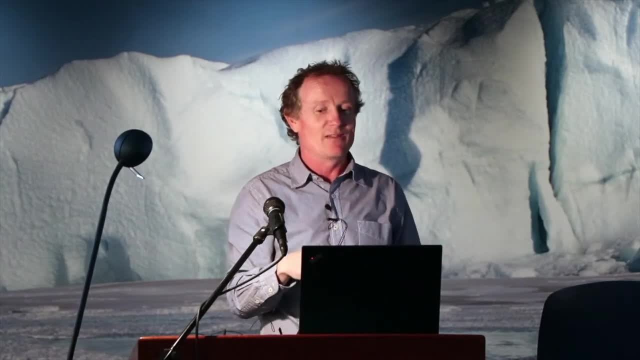 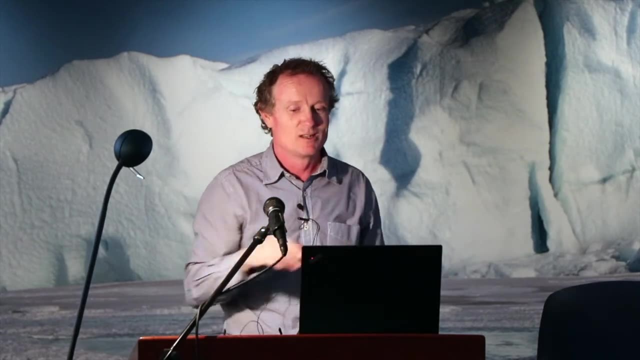 is managed if you keep going down at the bottom to the traffic lights turn left and you go past the Menzies Research Institute, which is where the next of our krill connections comes in, and I'm going to pass across to Laura who's going to. 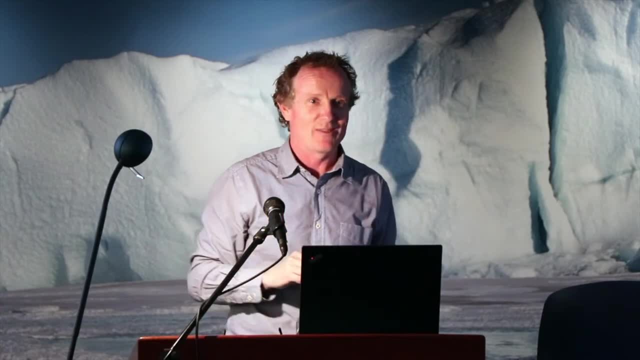 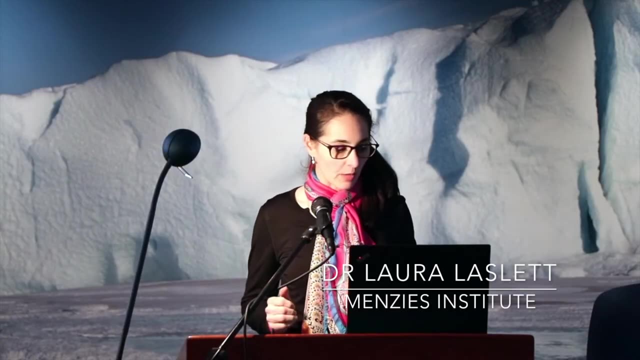 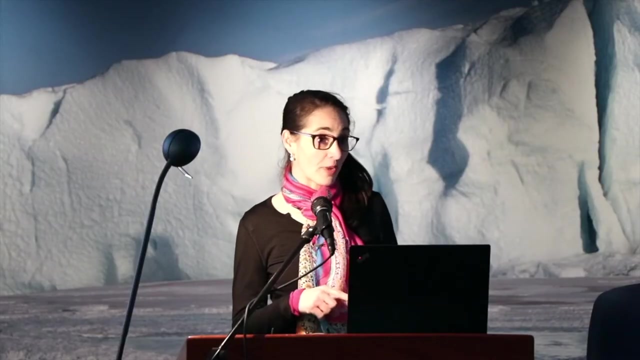 explain about the krill oil industry, The uses of krill and how that research has been conducted in Hobart. So I'm going to talk about about our use of krill oil a bit and, as Keith has just said, that I don't have any krill in tanks and I'm not managing the fishery. 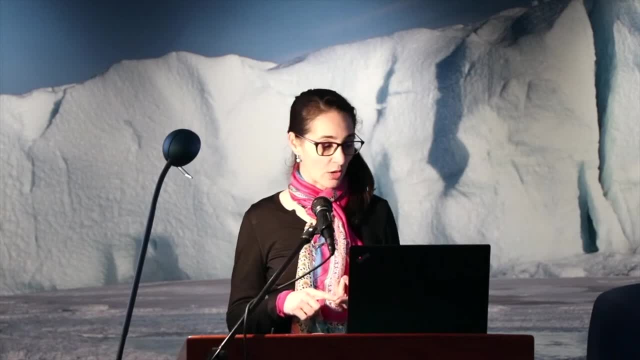 but I am looking at a use of krill oil in human health. so our research group at the Menzies Institute in Hobart is working to find treatments for osteoarthritis. so our research interest is is musculoskeletal health, and we're doing that because there's some evidence that. 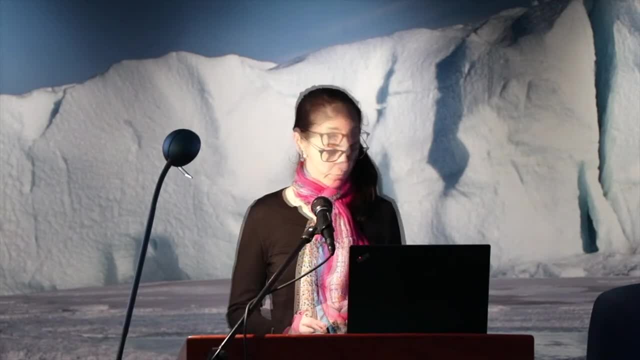 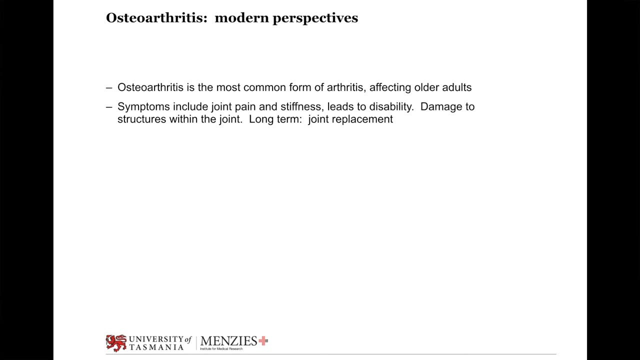 krill oil might be helpful for treating knee osteoarthritis. so I'm going to talk to you first about osteoarthritis. it's the most common form of arthritis. there are over a hundred different forms of arthritis, and osteoarthritis mostly affects older adults, and the symptoms of osteoarthritis include joint pain and 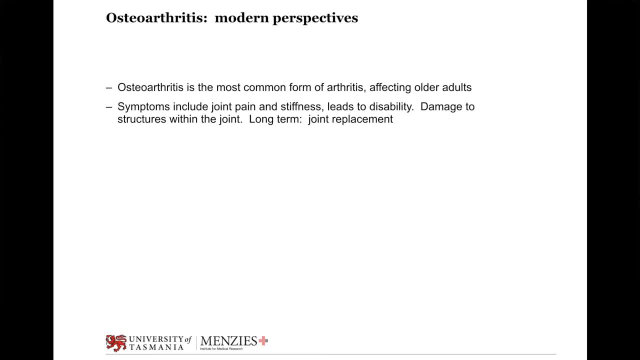 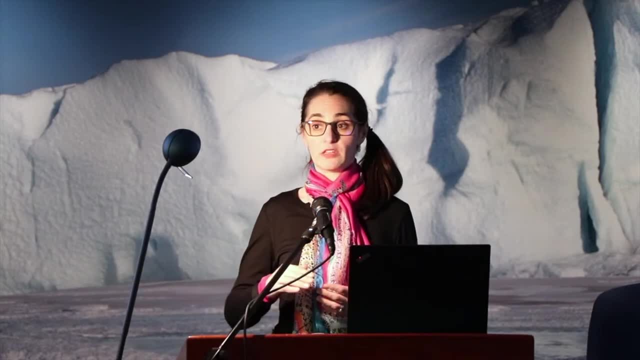 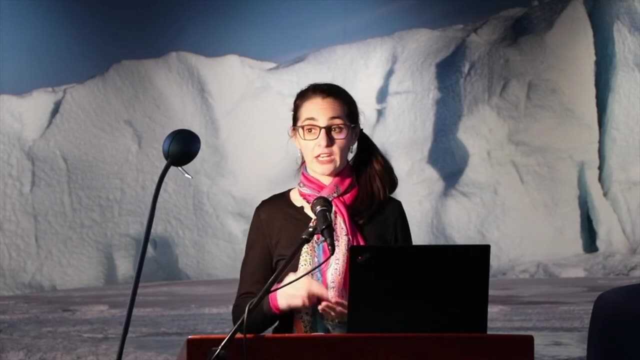 stiffness and this leads to disability and damage to structures within the joint. so people who have osteoarthritis and in the long term, the main treatment is knee replacement- but hopefully people won't get there. but basically, once everything else fails, you're looking at a knee replacement and so our job is to try and make sure that we can treat. 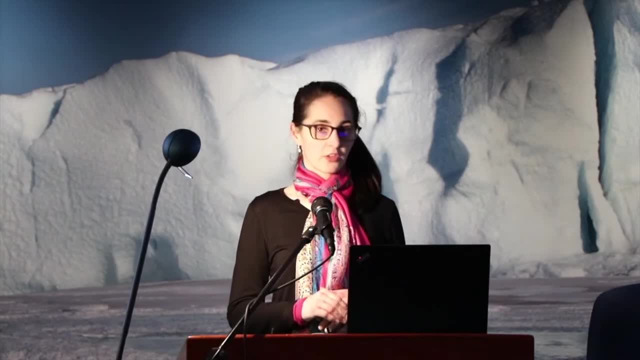 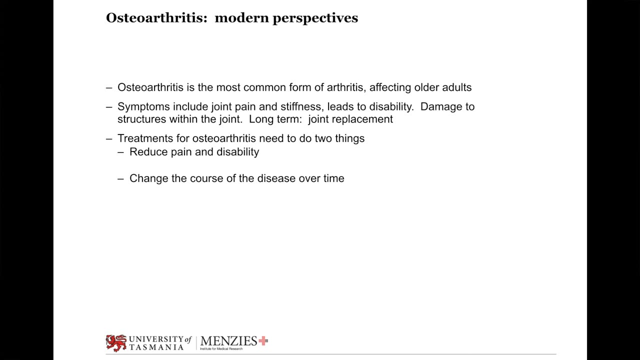 osteoarthritis well, and we can stop people from getting there. so treatments for osteoarthritis need to do two things: number one, they need to reduce pain and disability, and number two, they need to change the course of the disease. so we're going to talk about these. 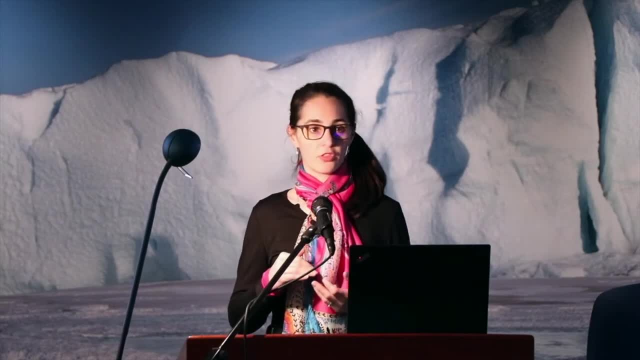 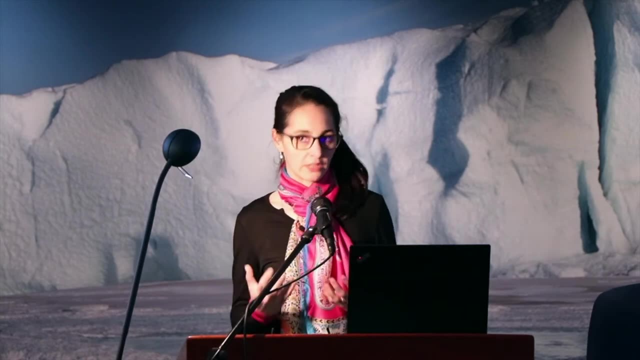 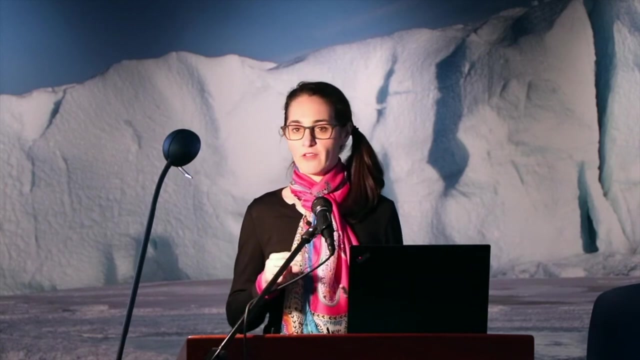 we really want to be doing is to be slowing down the path of any individual with osteoarthritis towards a knee replacement- and mostly I'm talking about knee osteoarthritis today because that's where my expertise is- but osteoarthritis affects the large joints, so people have osteoarthritis. in their hips, and you can have osteoarthritis in your hands as well. predominantly, treatments for osteoarthritis at the moment focus on reducing the pain and disability, so treatments are essentially that's what. that's what we focus on and that is in part because it's important. 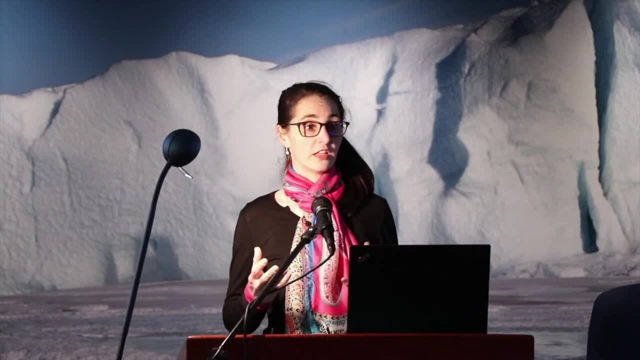 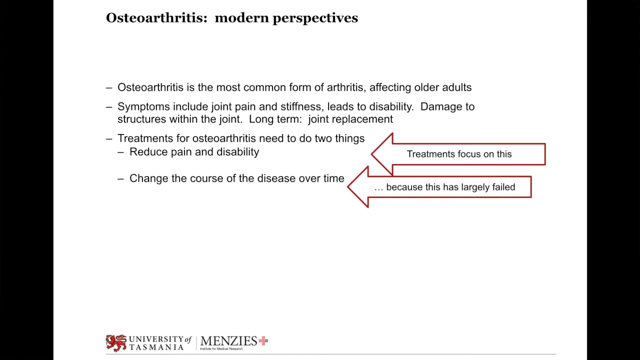 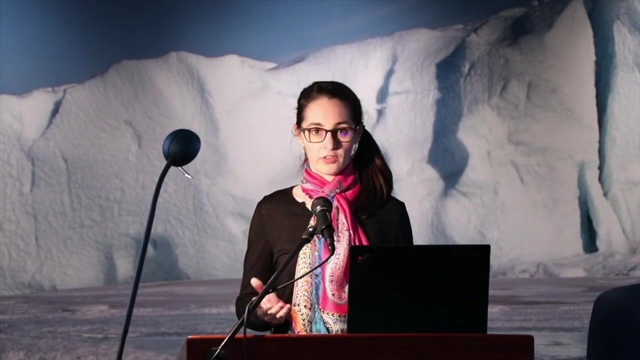 and that's what patients tell us is most important to them is is pain and and their limitations on daily life. but secondly, treatments focus on on the pain and disability because the second aspect, which is the changing of the disease course over time, has largely failed. that's quite disappointing. 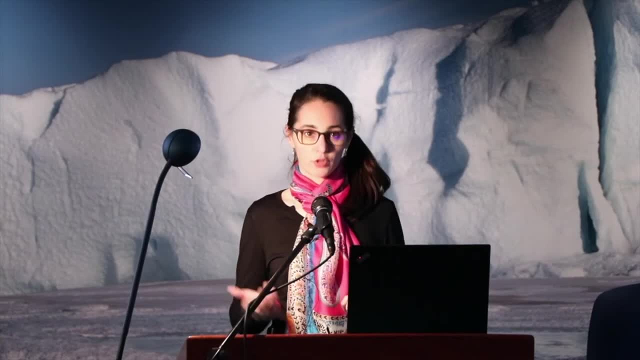 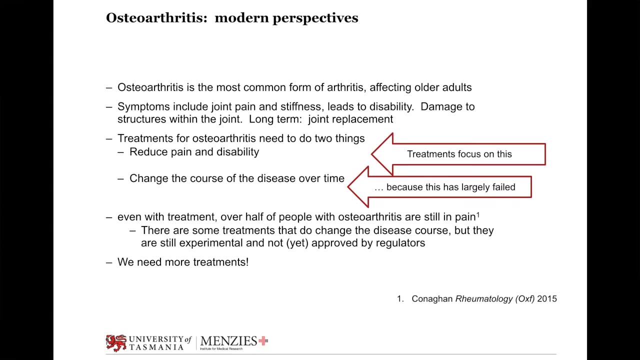 that essentially what we, what we have been doing in the past in osteoarthritis treatment, is actually treating the symptoms and not really treating the cause. and even with treatment, over half of people with osteoarthritis are still in pain, and we do have some treatments that do change. 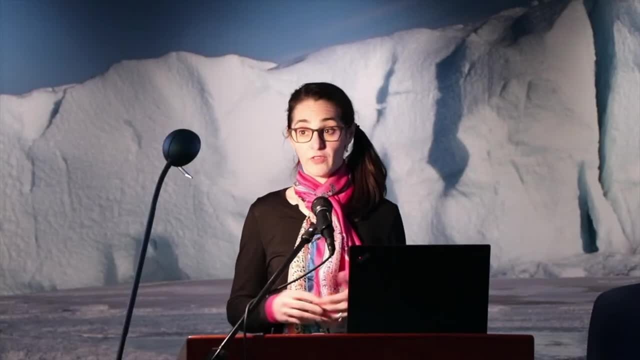 the disease course, but they're all experimental. some of these we've actually done in our centre in Hobart, but they're not approved by regulators at the moment. so we need more treatments, and so that's um. so that's why we're interested in krill oil, and so at the moment, what happens? 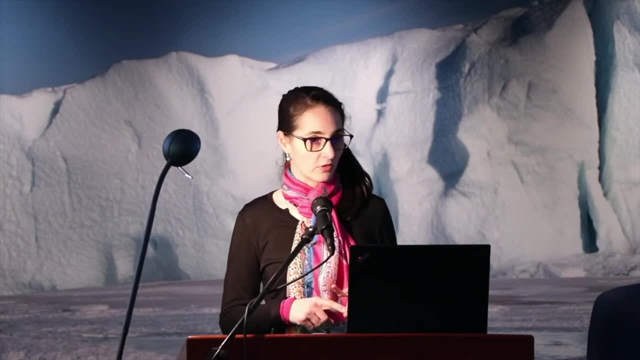 for most people is: they go and see their GP, they get some treatments, which you know might include drugs but might include other things, and then the next thing that happens usually is they get sent, sent to see the orthopaedic surgeon, and we know, for a number of reasons, 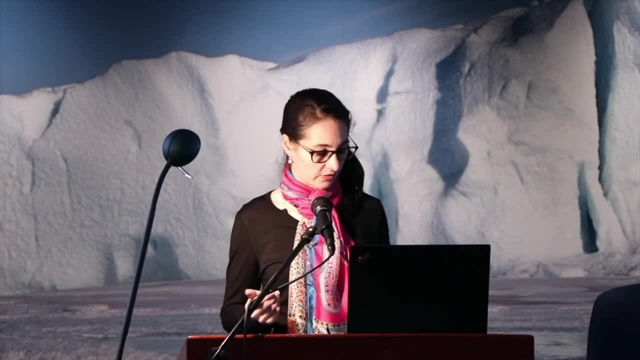 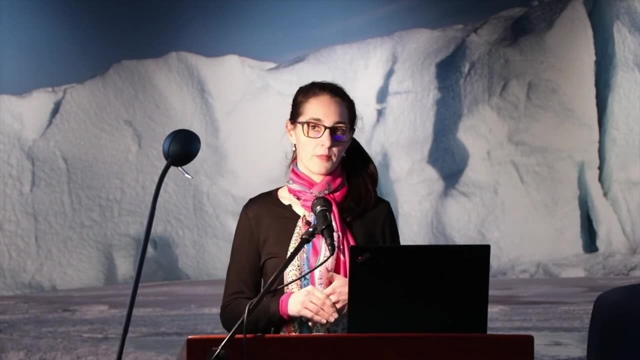 that's not. that's not good and if, if nothing else, it's not sustainable. it's it's expensive to be giving people joint replacements. there are a number of different types of osteoarthritis, so subtypes. we think that one of the reasons for the failure of the treatments 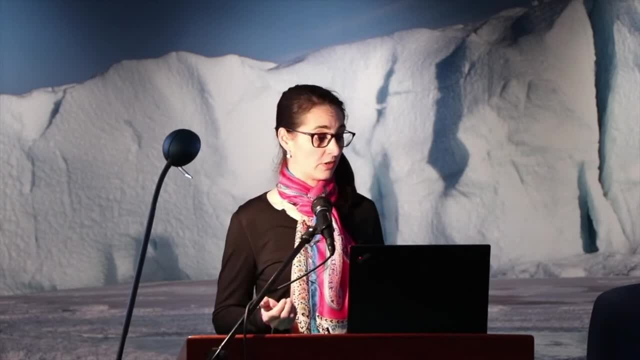 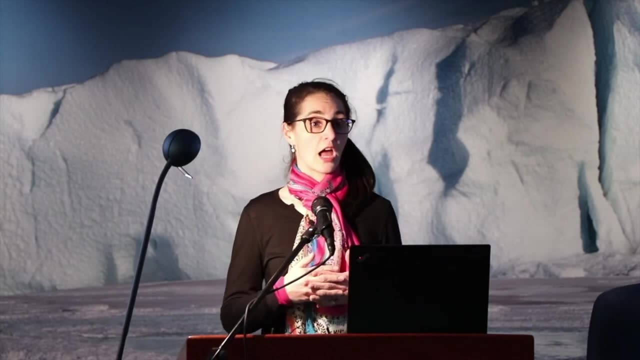 in osteoarthritis is it's been treating everyone as if they had the same disease, but actually we'd know that they don't. that's actually not true. there are- there are actually many pathways towards, towards pain and towards disability, and because there are many, many, many parts. 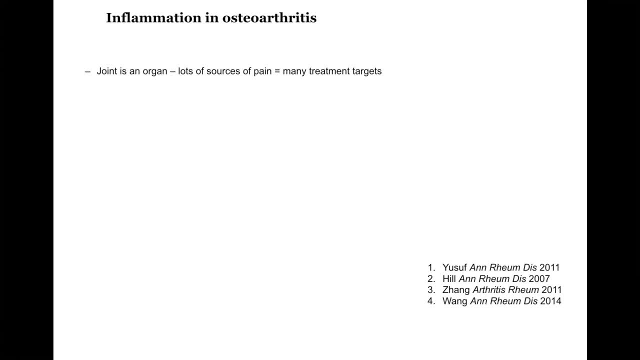 of the joint, and the joint works as an organ, and one of the subtypes of osteoarthritis that we know of is inflammation, so localised inflammation in the knee, which is known as effusion. so that's, that's a swollen fat hot knee. this is one type of osteoarthritis that we've been focusing on. 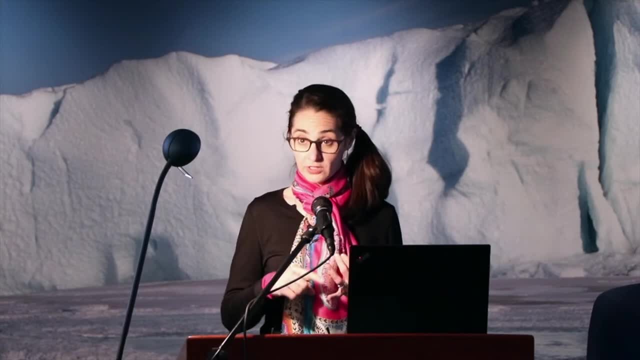 and so this localised inflammation is important because it predicts pain. now you might also be thinking about. one of the types of osteoarthritis that's well known is rheumatoid arthritis, and that type of arthritis is where you have inflammation everywhere and you have very high 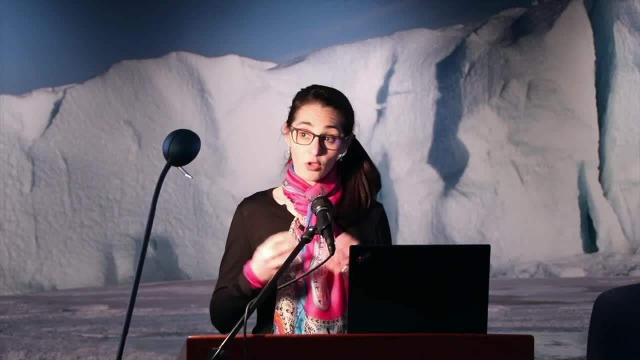 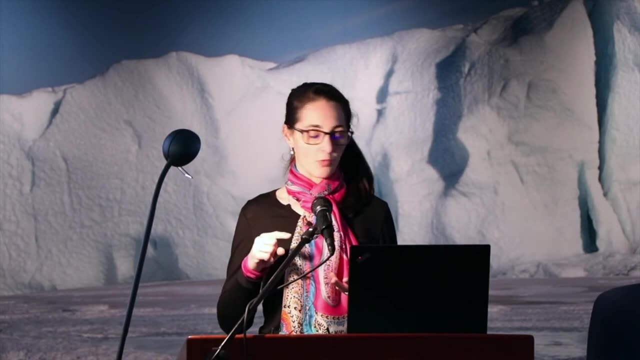 levels of inflammation, but inflammation in the context of osteoarthritis is very localised, and so this localised inflammation predicts pain, especially pain, what we would call non-weight-bearing. that would be pain when you're doing what you're doing now. you're sitting, you might be lying down. 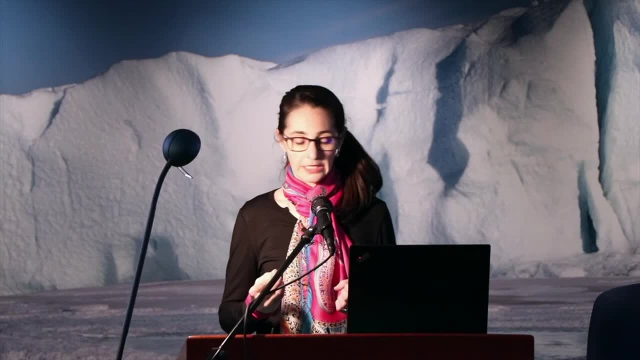 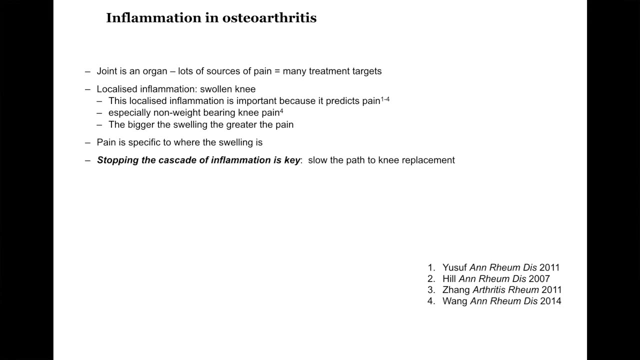 in bed trying to sleep. so that sort of pain is typically an inflammatory pain, and the bigger the swelling in your knee, the greater the pain. so stopping the cascade of inflammation is the key and- and this is how we're planning- to slow the path to knee replacement. 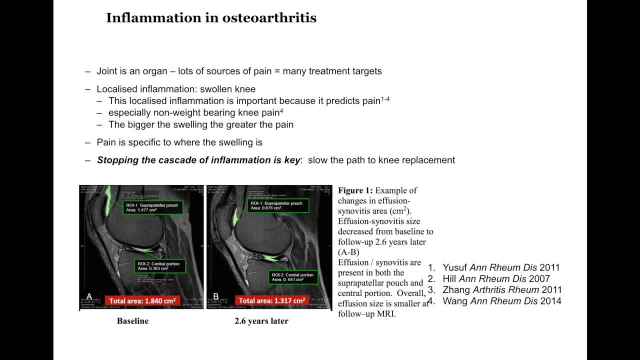 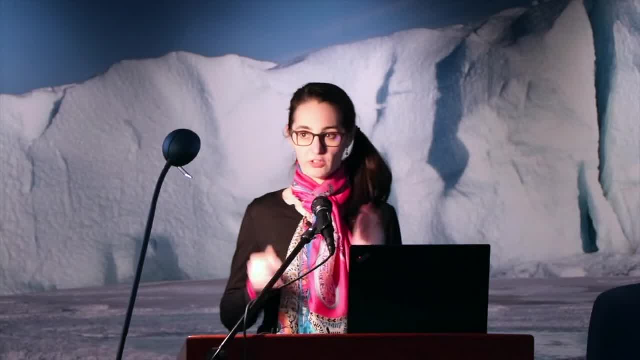 and so this is the only medical picture i've got for you tonight. so this is what, um, what swelling looks like on an mri. you can see the, um, the kneecap, the on the left hand side. so if you imagine one facing that way, this is a slice through their knee and so the green bits in there are. 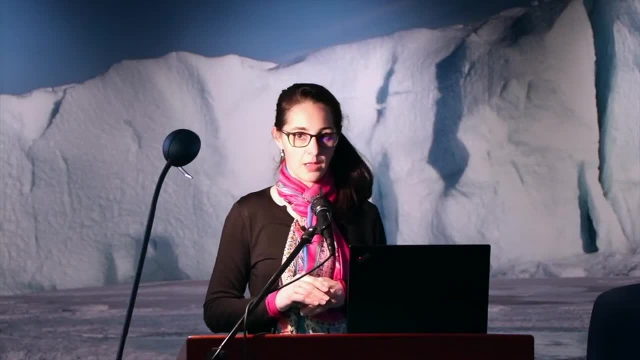 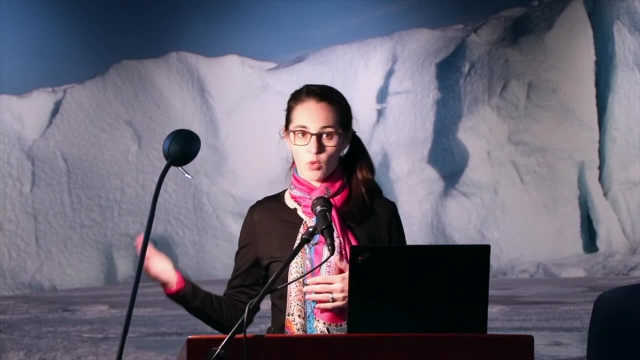 some swelling on the inside of the knee. so this particular um picture is taken from one of our longitudinal studies. so we've looked at people and followed them over time, just looking at what happens. we didn't treat them and the panel on the left is at baseline. so at the beginning and the 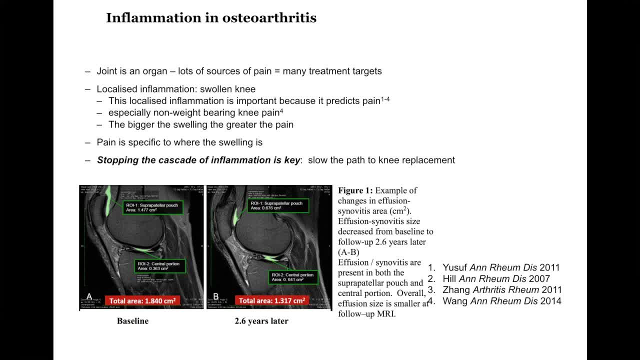 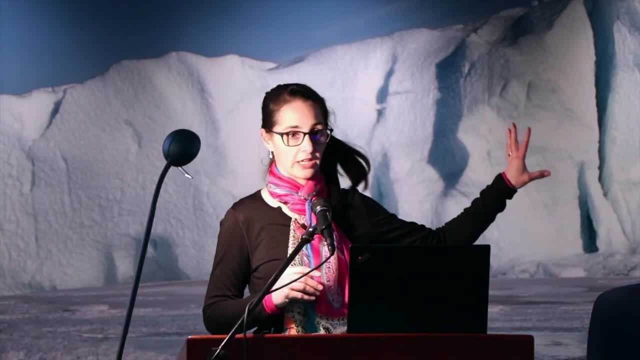 second panel is two and a half years later. so for this particular person, the swelling inside their joint, um, is about two and a half years later. so for this particular person, the swelling inside their joint got smaller and the technical term for what we're looking at is a fusion sign of itis. all that means. 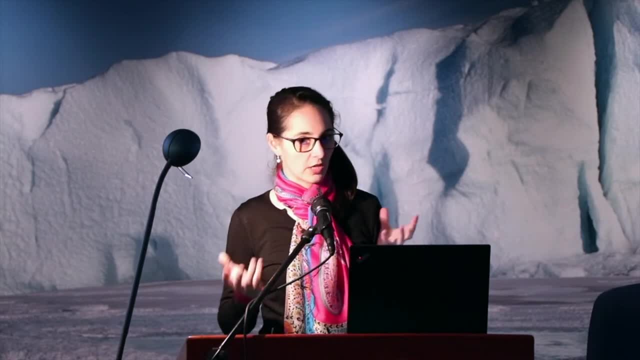 is that we actually can't differentiate between some of the things we're seeing on these mris, and that's because, for research scans, we actually choose not to give people the chemical that would be required to see the difference, because it's not very not safe enough for research. 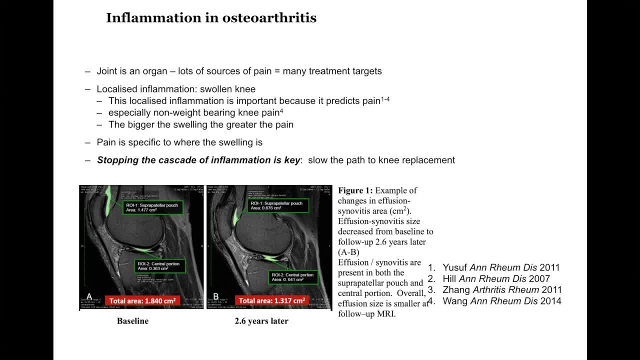 patients. so you can see those green bits on the on the slide, and so that's actually what we're looking at inside the knee. so if you see it from outside the knee, it's a hot fat knee. if you see it from the inside of the knee, you can see 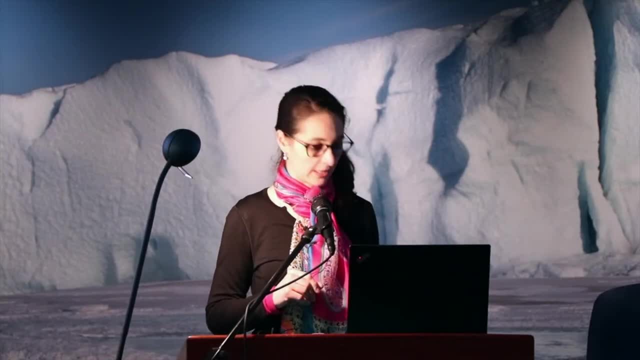 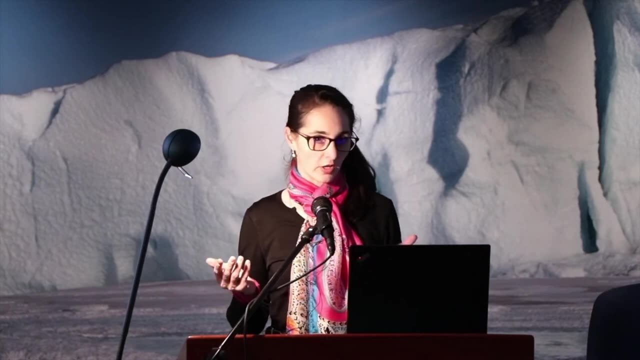 you can see bits of fluid that um, that are actually quite clear on the mri. so i'm going to take a step sideways for a moment and talk about how we're going to know that a treatment works. so the last slide i showed you i said that was from one of the studies where we've 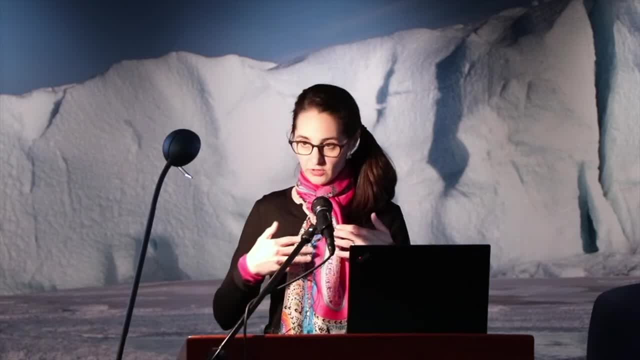 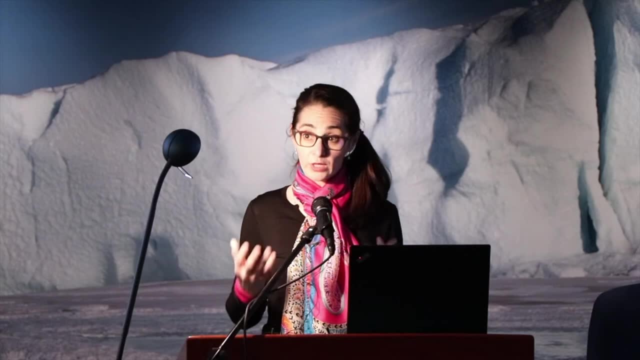 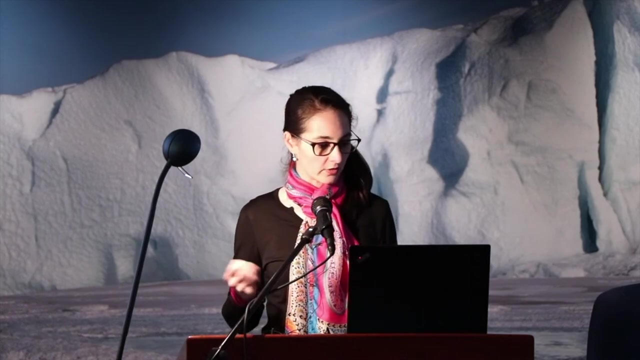 just looked at people over time. we didn't treat them, we just looked at what was happening over time and so that's called an observational study. but a really important tool we have in medical research is is the randomized trial. so this is a way of helping work out whether a treatment works. so we randomly assign people in suitable people to receive one. 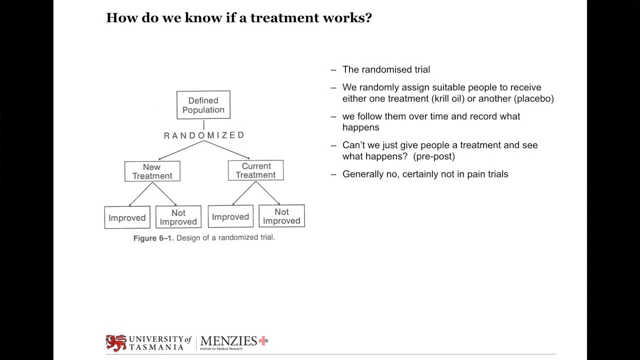 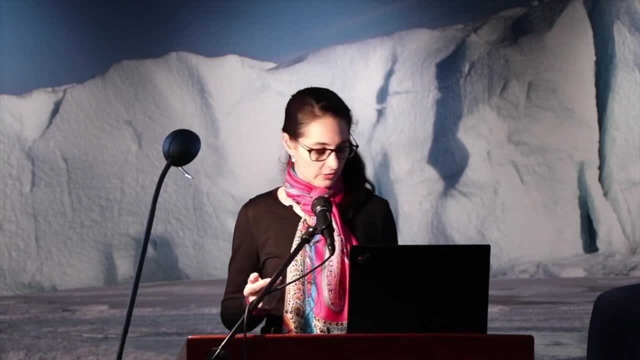 treatment or another and we follow them over time and see what happens. and you might be thinking: why are we bothering with this? can't we just give people something and see what happens? but we can't, certainly not in pain trials. and that's because in in osteoarthritis and in other painful conditions, it's not the same all the time. so people go through cycles of pain. so today you might have a lot of pain, maybe because you went for a long walk yesterday, but today your pain might be better. but also that the pain cycles are longer than that, and you know they just they fluctuate over time. 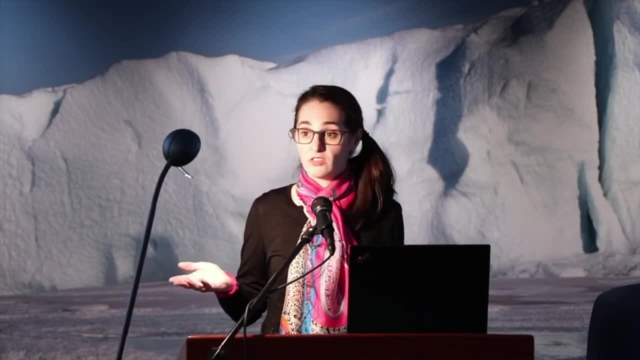 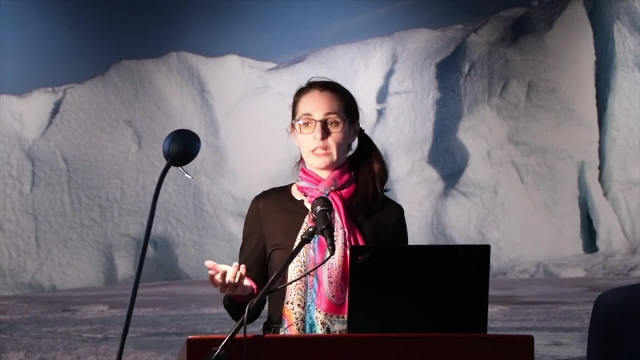 related to maybe factors to do with the disease, or maybe activity, or maybe nothing at all or nothing that we know of, for example. so we typically in a clinical trial when they're in a lot of pain. maybe they see an ad in the paper and think my knee really hurts. 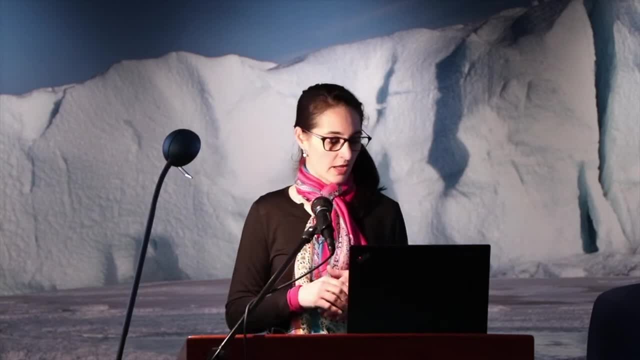 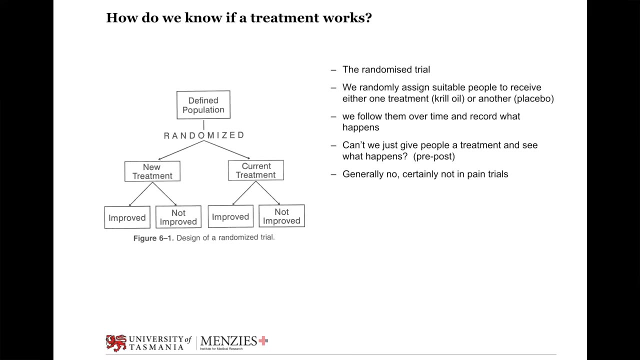 i think that i might go and try some of that and maybe, if your knee doesn't hurt well, you might just scroll past and read something else in the newspaper. so in our trials, typically we see people when they're in a lot of pain and then over time and their pain will go down and this fluctuation- 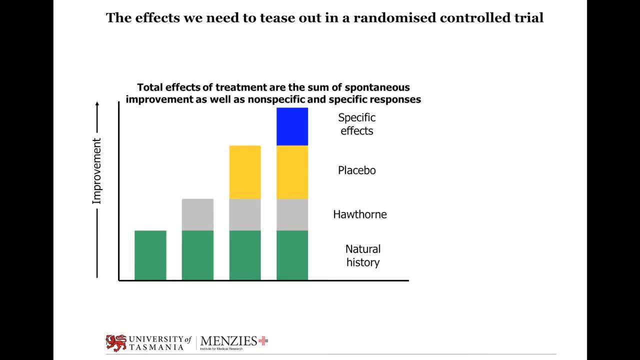 is normal and is part of the disease process. what i've just described is, in part, called natural history, so we know that people's pain changes over time. if we're recording what's happening to someone, there's also what we call the hawthorne effect, the effect of being watched or observed. you know. 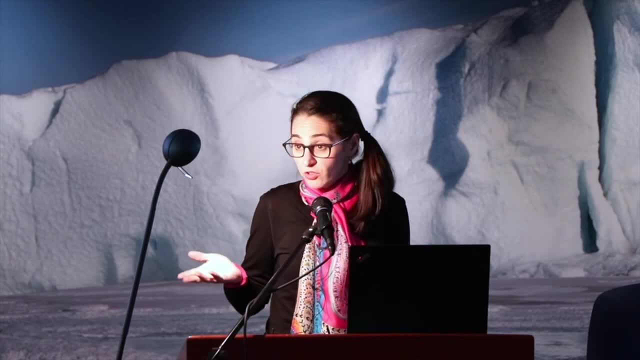 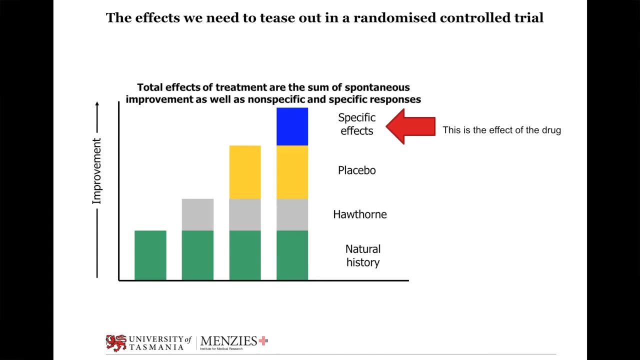 you talk to a nice researcher, you know the doctor asks you some questions, and then there might be the placebo effect, which is the effect of being given a treatment that you think might work, and then there's the effect of the drug. so if you, if you don't do the sorts of trials that 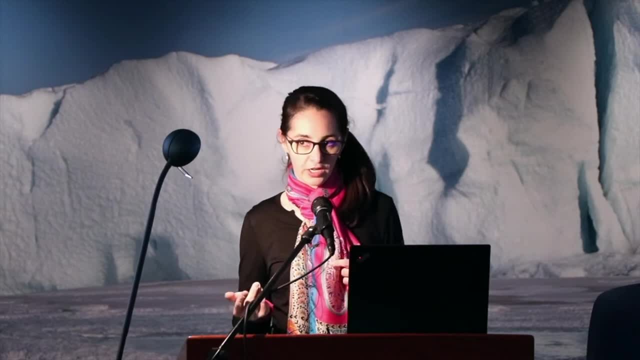 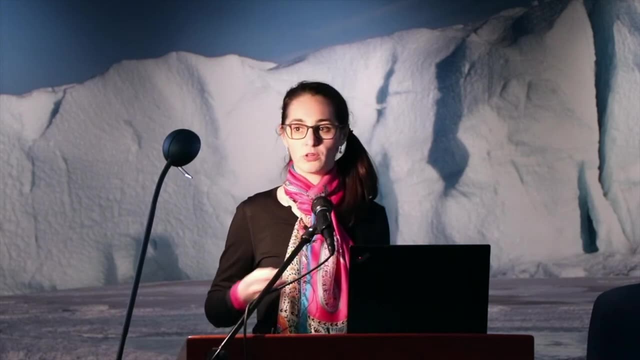 we're talking about. how are you going to know what the effect of the drug is compared to all these other things we're talking about? so doing these sorts of trials in medical research is really important, because that's what helps us work out what the effect of the drug is, and it 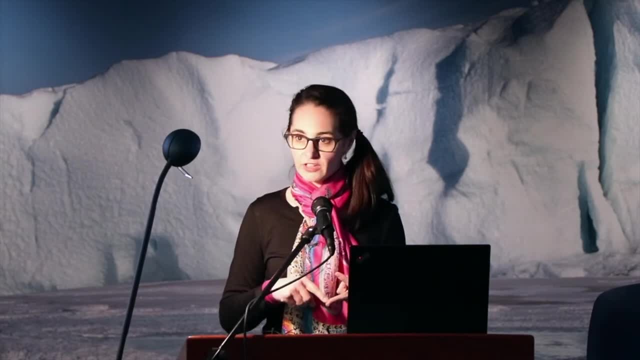 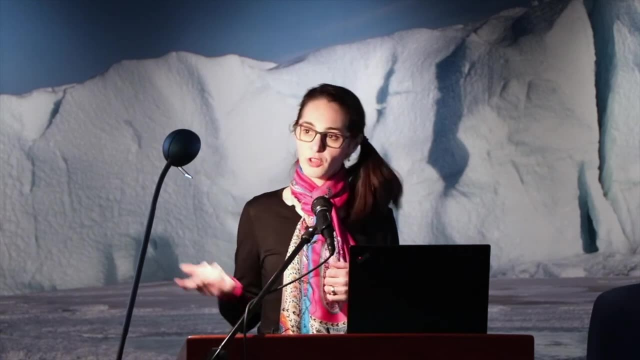 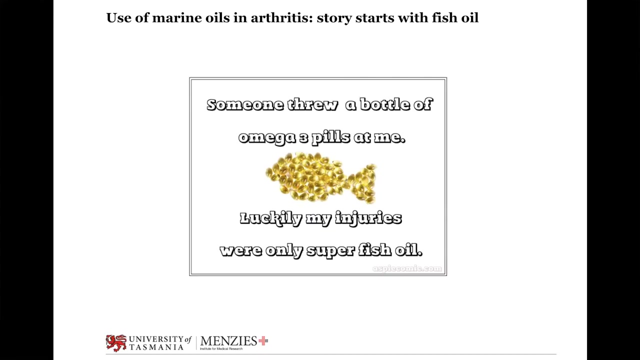 also gives us an opportunity to figure out what the side effects might be, or, in fact, anything else that might be important. i've told you why it's important that we do these trials. so back to osteoarthritis, and i promise this is my only bad joke for the talk. so the the use of marine oils. 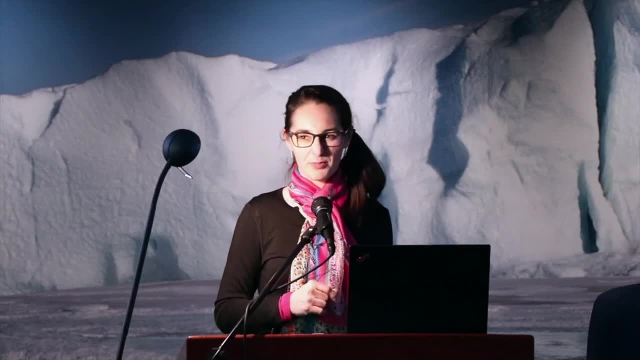 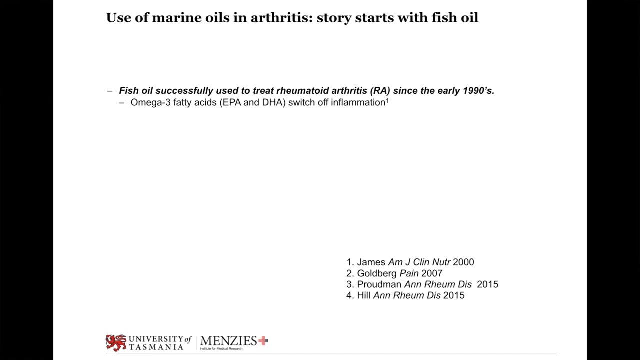 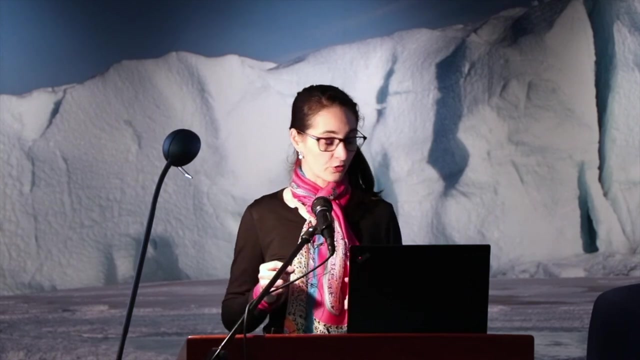 has a history going back a few years. yeah, it is a pretty bad joke, isn't it sorry? the use of marine oils dates back to the 1990s, so fish oil has been successfully used to treat rheumatoid arthritis since the early 90s, and we know that the omega-3 fatty acids in the fish oil switch. 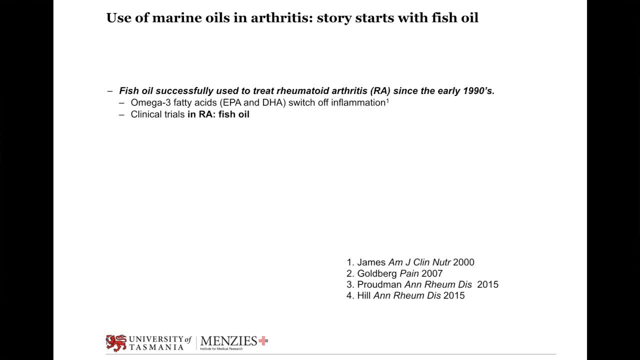 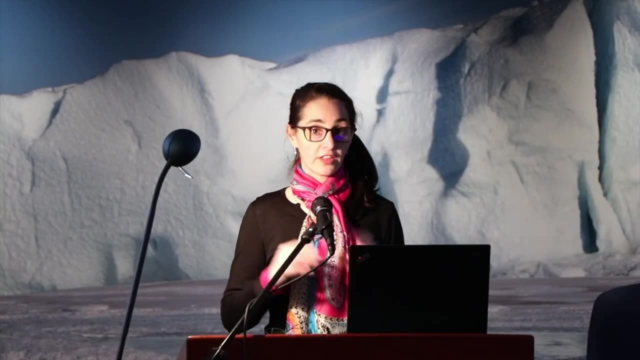 off inflammation and clinical trials have shown that that fish oil reduces pain, morning stiffness, the number of painful and tender joints and use of pain medicines, and it increases the likelihood of that someone will go into remission when used as well as the standard therapies, so that's a good. 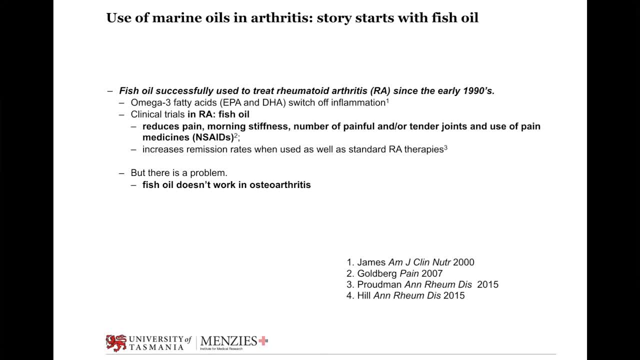 news story. if you've got rheumatoid arthritis, fish oil is good for you, but we have a problem as far as osteoarthritis is concerned, that we know that fish oil does not work in osteoarthritis. so a two-year trial of high-dose fish oil versus low-dose fish oil in people with knee osteoarthritis. 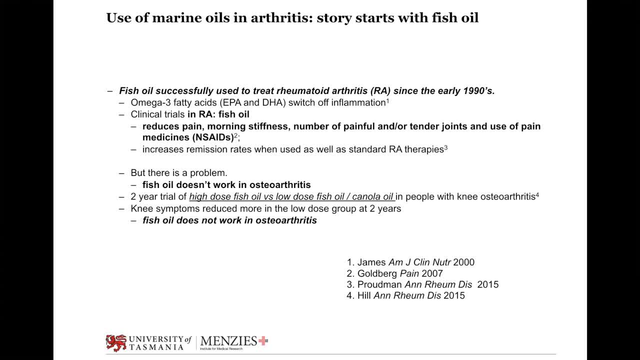 some of which patients came from hobart and were looked at in our center. this two-year trial showed that the knee symptoms reduced more in the low dose group, which was supposed to do nothing, compared to the high dose group. so this has shown us that fish oil doesn't work in osteoarthritis. 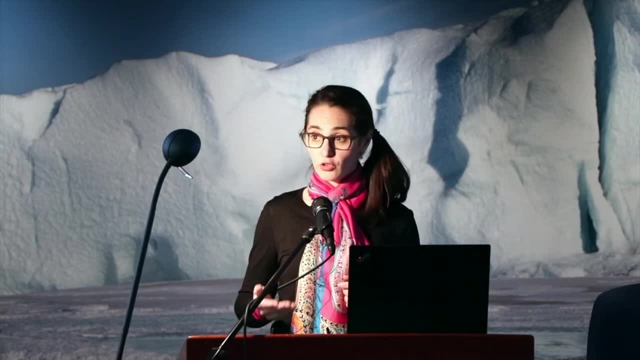 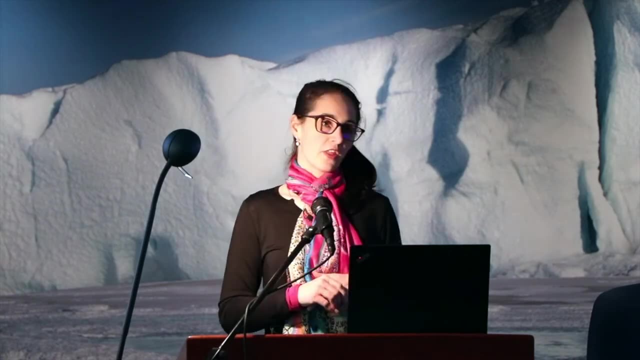 or, conversely, that perhaps canola oil does. so that's contrary to what we were expecting, but certainly it tells us that it doesn't have the effect in osteoarthritis that it did in rheumatoid arthritis, and there's been some evidence in krillo that krillo might in fact 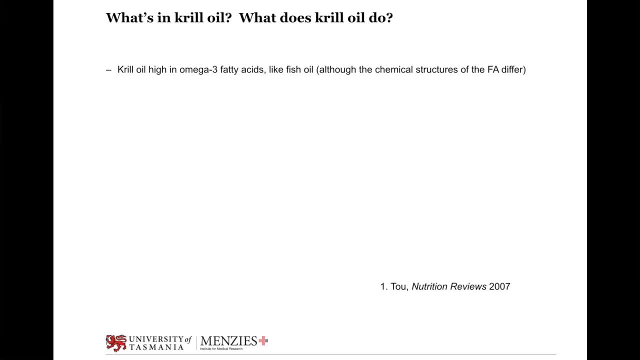 work. but i've just told you that fish oil doesn't work, so why might krillo work? well, krill oil is high in the omega-3 fatty acids that are also occurring in fish oil, although the chemical structures are a little different. but krillo also has antioxidants. 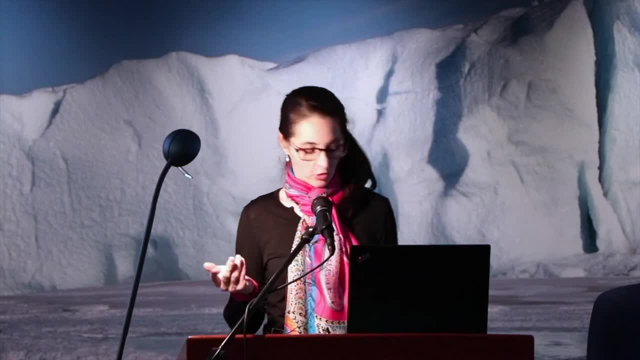 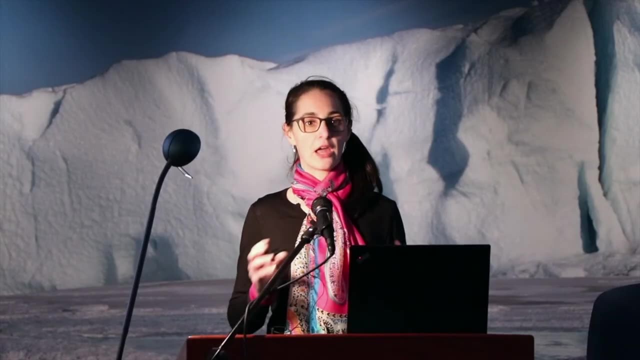 which fish oil doesn't. might this be the magic ingredient? well, we're not sure, but in terms of the two marine oils, the bioavailability of the krill oil is better, so that means that for a given amount of oil, you would get more of the good things in it, which is important for you know. 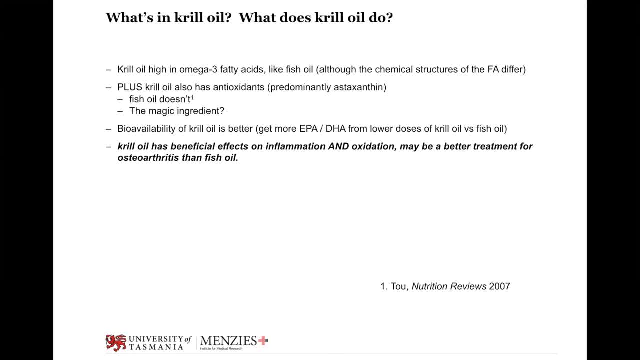 the biomass and you know amount in a pill and all that sort of stuff. so there's evidence to say that beneficial effects on inflammation and oxidation and therefore may be a better treatment for osteoarthritis than fish oil. Then we move on to some of the 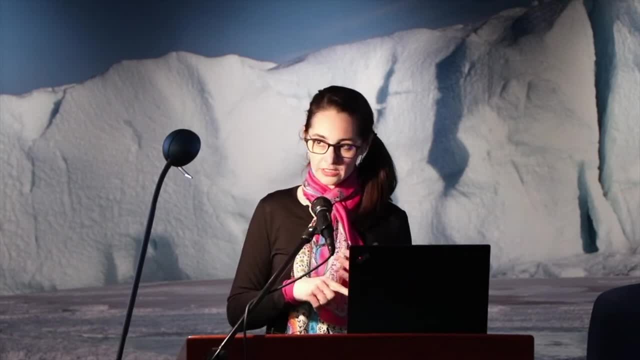 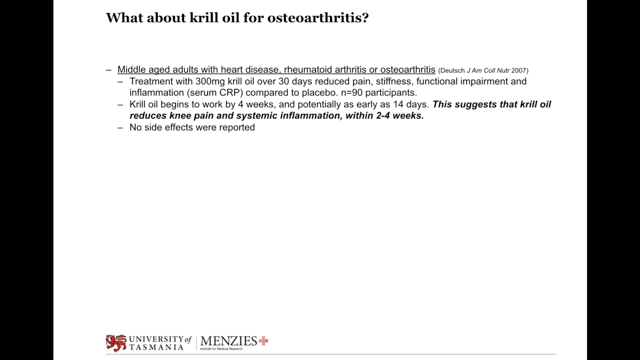 evidence. So, given that you can buy krill oil in every pharmacy, every supermarket, how many trials do you think there might be in osteoarthritis? This is it One trial, And in fact there are three other trials I've been able to find in human. 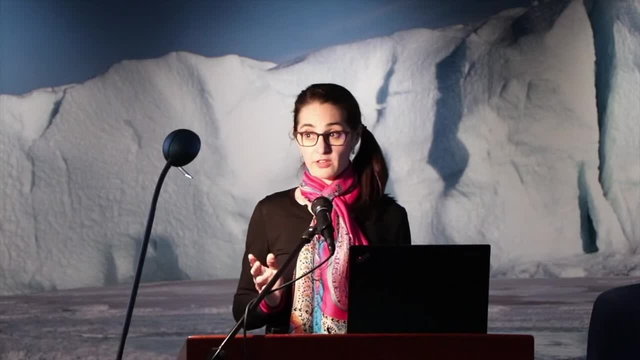 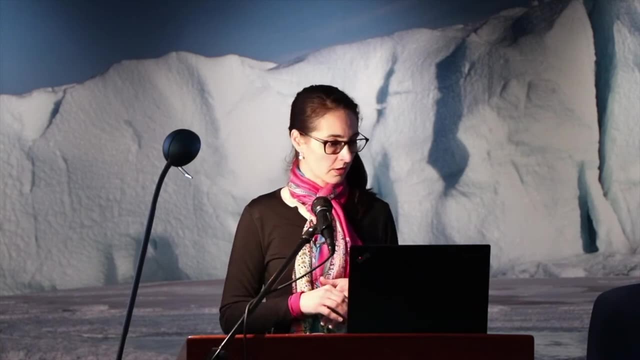 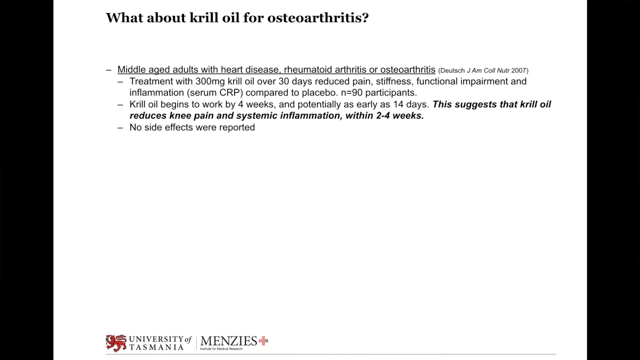 health. That's it. So the evidence base is certainly not anywhere near as strong as fish oil and one would say is encouraging but not strong. So the one trial of krill oil for osteoarthritis looked at 90 middle-aged adults in 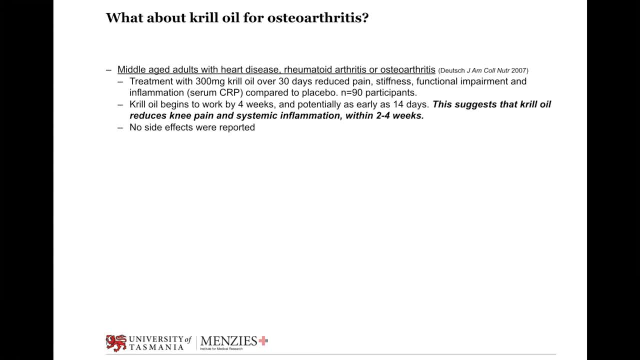 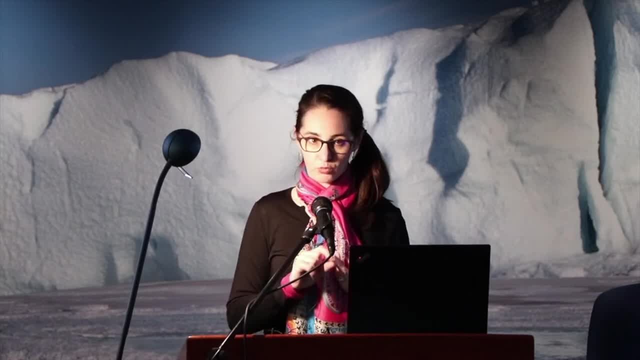 people with three disease groups: heart disease, rheumatoid arthritis and osteoarthritis- And certainly from the fish oil story that I've just told you, there's certainly important reasons to think that people with rheumatoid arthritis and osteoarthritis can have a higher risk of osteoarthritis than people with osteoarthritis might respond differently to krill oil, So this study looked at treating them with a low dose over a month and looked at various aspects of the disease that we know are important, and has shown that krill oil begins to work by four weeks and is potentially as early as two weeks. So this suggests that krill oil reduces pain and systemic inflammation within two to four weeks. So that's great. So not only is there evidence that it's reducing pain, which is important to patients, there's also evidence that it might reduce the risk of osteoarthritis. So that's great. So not only is there evidence that it's reducing pain, which is important to patients, there's also evidence that it might. be modifying what's going on in the knee, which is also very, very important. And there were no side effects reported, So we know that krill oil is very safe, but most people would take any medicine for more than 30 days and that's. 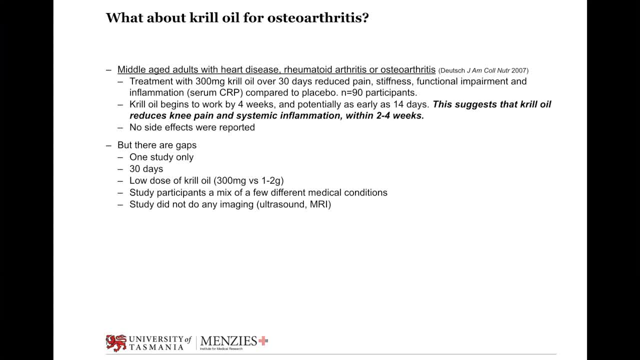 not very long to look at side effects. So, as I've said, there's gaps in this study. There's only one of them. It went for a month and it was low dose and the participants were a mix of a couple of different medical conditions and there 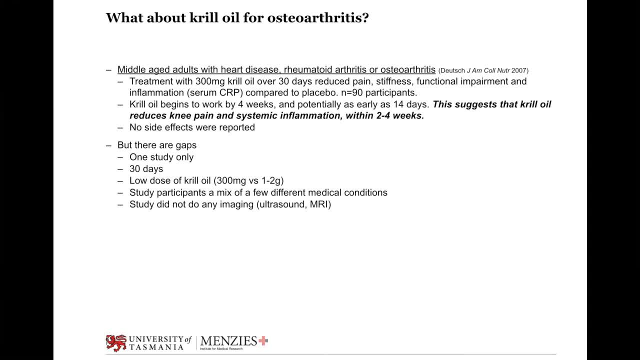 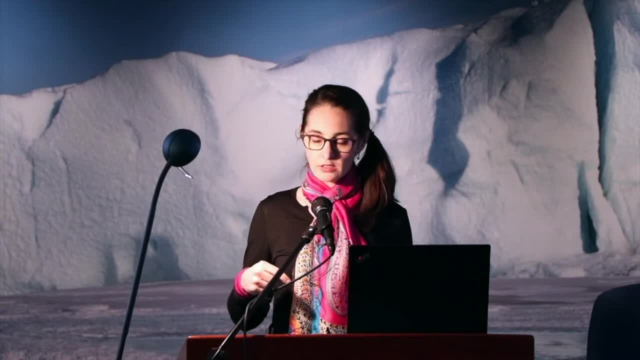 wasn't any analysis that allowed us to look at any of those groups individually, and there was no imaging data. So I've shown you some of the scans from our research studies. We really want to know what's going on in the knee, and there's 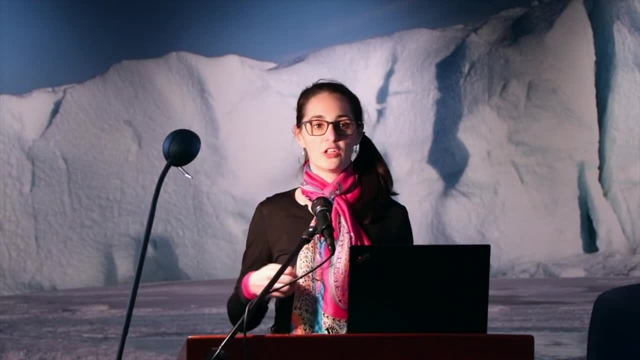 there was no data in this study for that, and that the the gold standard for osteoarthritis these days is MRI. Well, x-rays are good, but they're a hundred-year-old technology and there's many things you can't see on them, so we 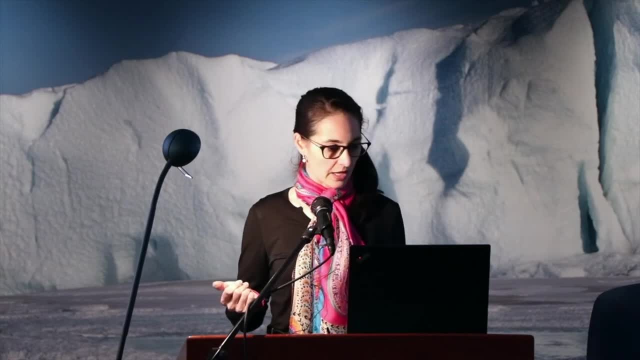 use MRIs. Obviously, there must be a need for a bigger, better study, and so our group has been successful in getting funding to do just that. So I'm hoping that if I was in, if I was standing here in two years, I'd be able to tell you what the effect of krill oil was in people with knee. 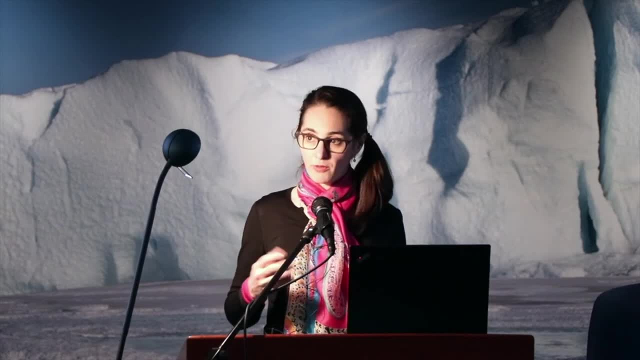 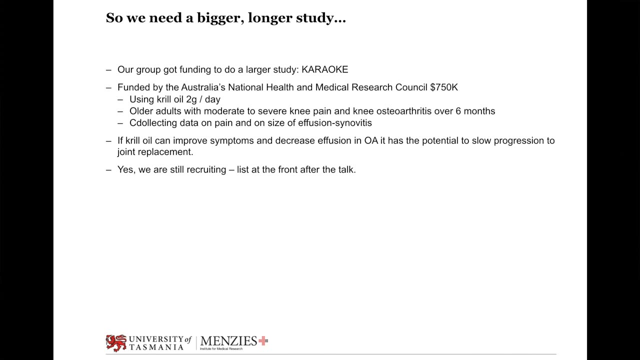 osteoarthritis, who have inflammation type of osteoarthritis. But we're not there yet, We're here today. so so today that I can tell you that we've got funding to do a longer, larger study, and so we've gotten funding from Australia's. 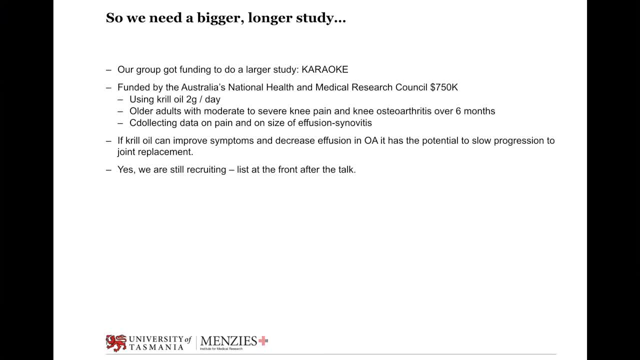 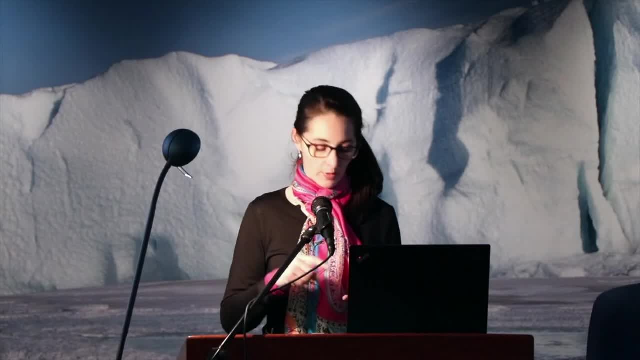 largest medical research funding body to do that, and so we've already started. in Hobart, One of our centres is yet to start, so we are running this study in Hobart, Adelaide, Melbourne, Perth and Sydney, and we'll be recruiting about 60 patients from each site, and so we've now 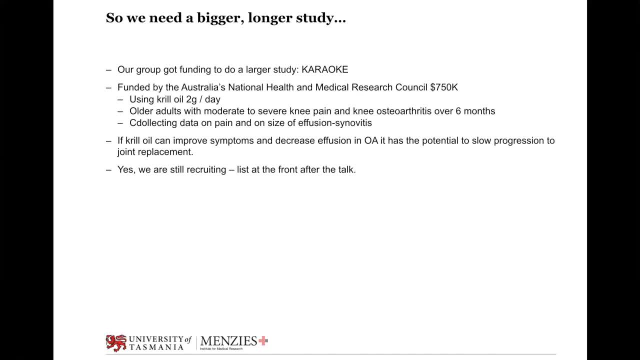 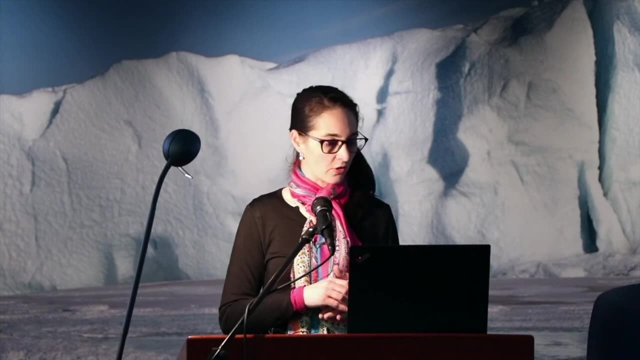 well and truly started in Hobart, and we're recruiting older adults with severe knee pain and knee osteoarthritis using a high dose of krill oil, and we're collecting data on the pain and also some information on what's going on with the knee and so that we're hoping. 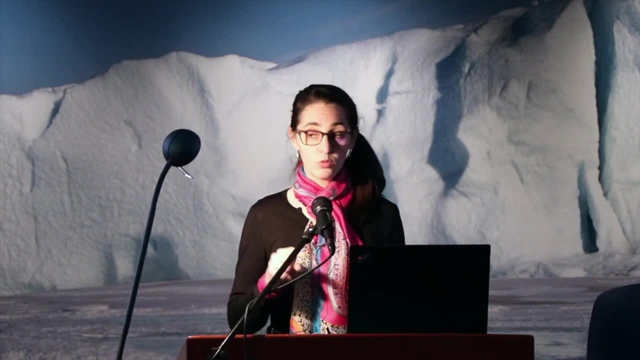 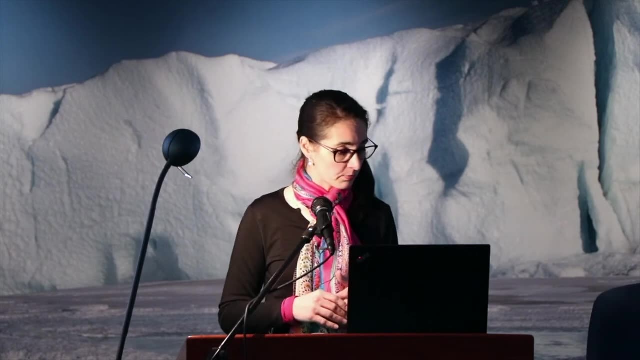 to find out whether it does change pain, as we expect that it will, whether it will change inflammation and other aspects of lipid metabolism. It's really exciting to be here to be able to talk to you about this, and actually I'm so excited to see these amazing krill- I've never seen these before tonight- and to think 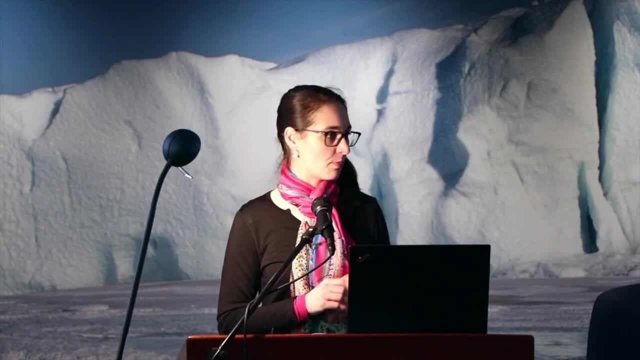 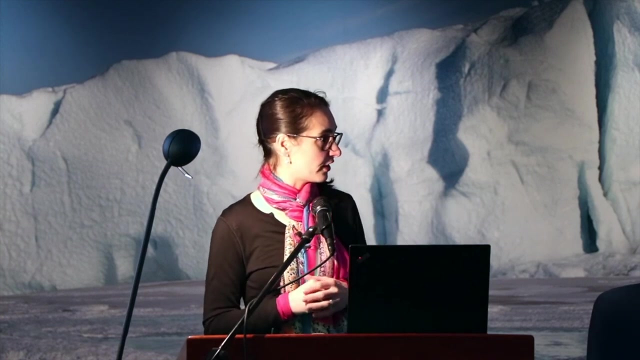 that these krill from the Southern Ocean You know, You know being well managed and being, you know, hopefully that they actually do work for osteoarthritis and these little guys can help us. So that's all I wanted to talk about tonight and I think we're moving on to the next section. 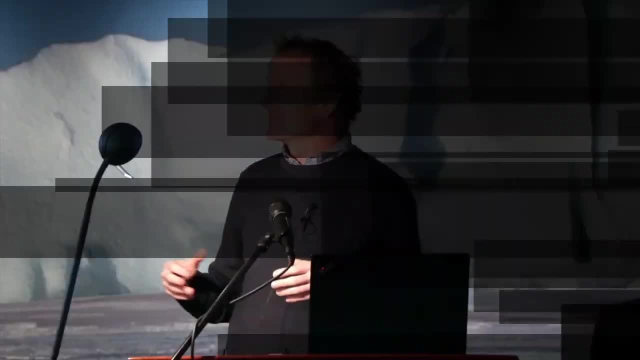 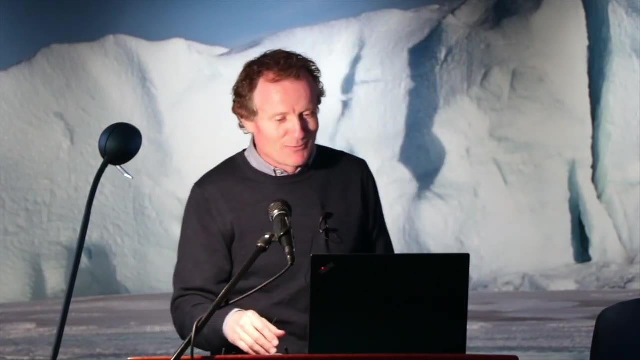 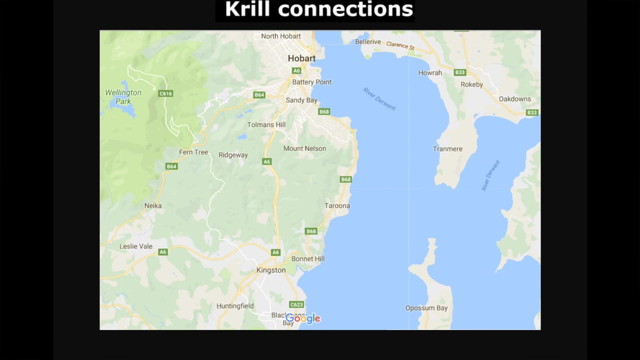 Thank you. So I go back to the question that we posed on our flyer: are we in the krill capital of the world? You know I'm biased If we start with our journey from the South, because that's where krill come from and